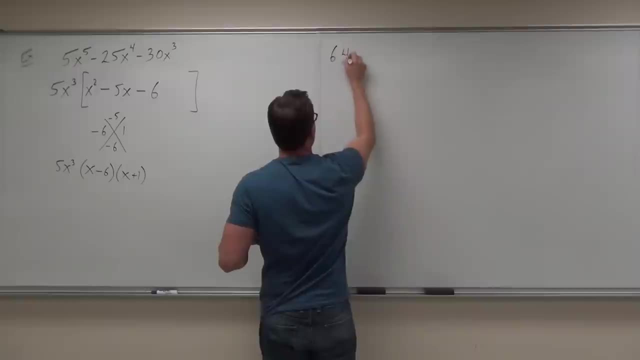 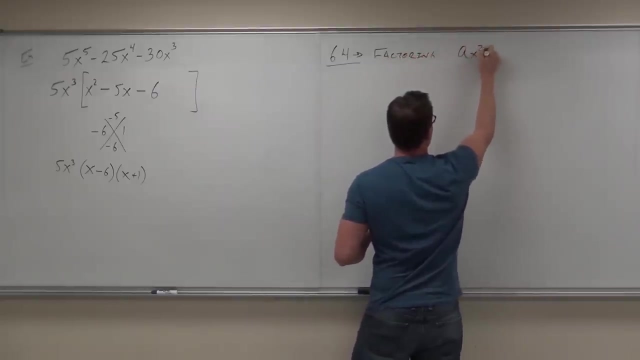 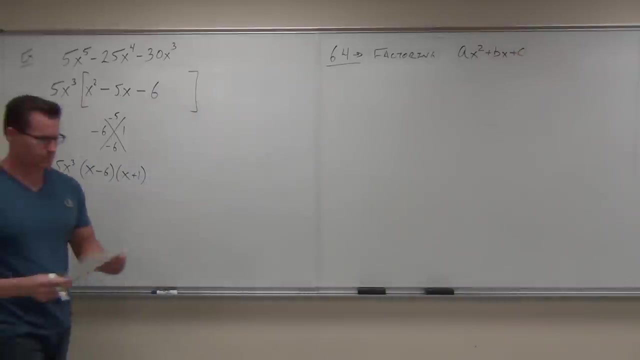 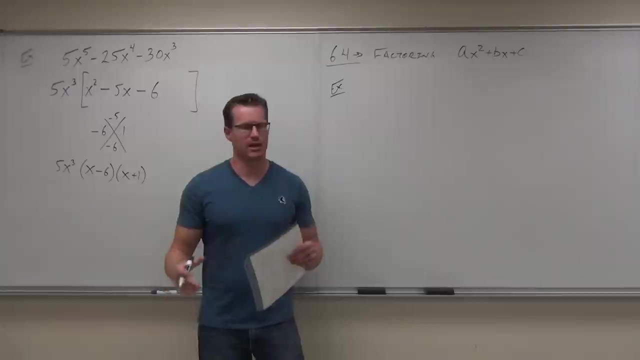 Section 6.4.. We're only going to have time for one example, because I want to explain this. It's going to be quick, I promise, And the rest of our day, probably like tomorrow, is just going to be practicing this stuff. alright. 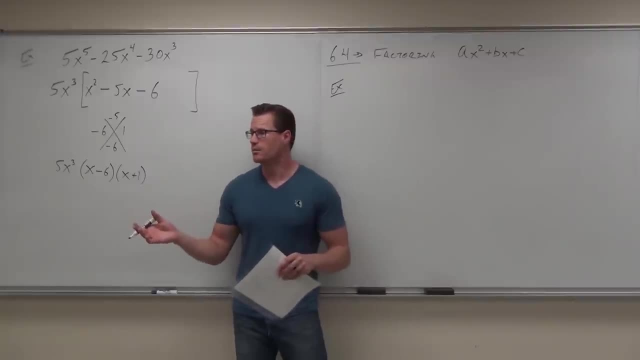 Because, honestly, this is one thing: you have to be pros at. Everything else in this class, like chapter 7, not so much chapter 8,, chapter 10, chapter 11, it all revolves around, or at least it does involve, factoring. 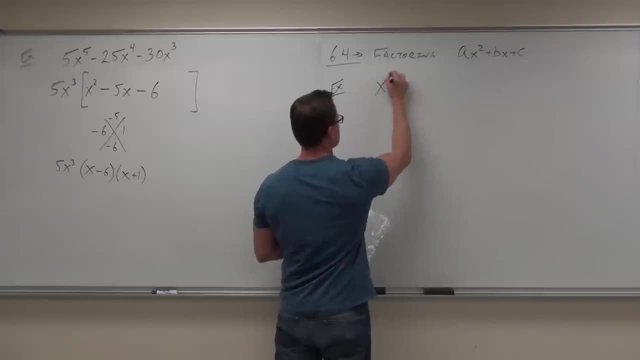 So here's an example of what I'm talking about: Old stuff, right, Old stuff. What would you use here? It actually doesn't factor, but you would try it, And if it did factor, you'd go directly to your factors with a shortcut. 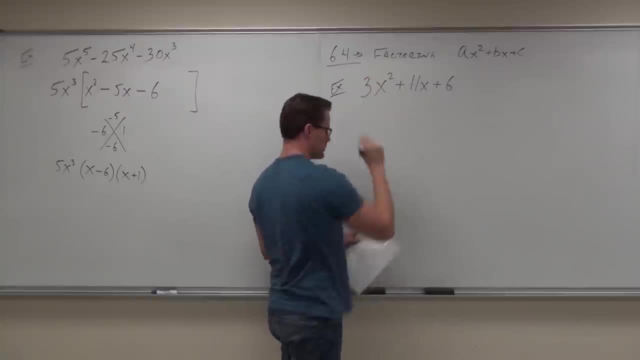 Are you understanding that? Okay, Now, as soon as I do, that you still have the same basic ideas in that first question. is it in order? That's great. Is the first term positive? If it's not, you'd factor the negative out. 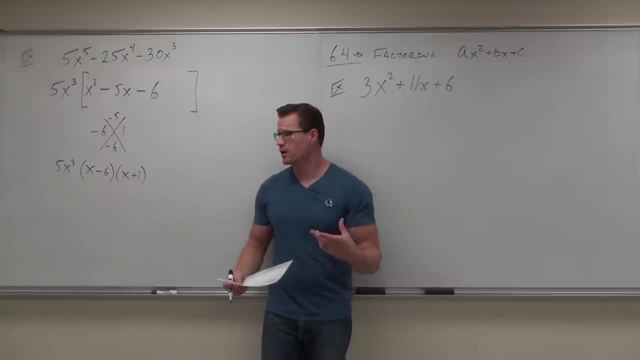 That would act like a GCF. Does it have a GCF besides 1?? Okay, So you're all good as far as that goes, But the problem we have here is that we have an A that's not 1.. That doesn't mean you switch everything up. 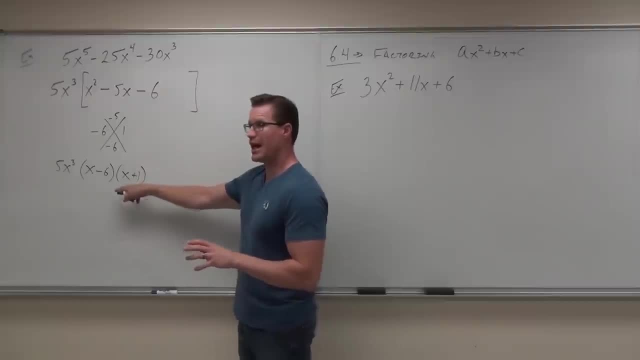 That just means that instead of going directly from here to here, you have that extra step I was referring to. So diamond problem, part 2.. We are still going to put B here. Still going to do that Now, do you remember? 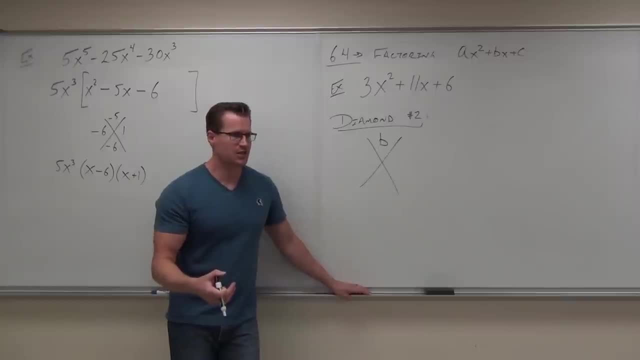 Hopefully you understand. You understand why I did what I did. You understand that the reason why I had you always do A times C, even though A was 1, all the time was for this. So you get in the habit of going: oh yeah, A times C goes here. 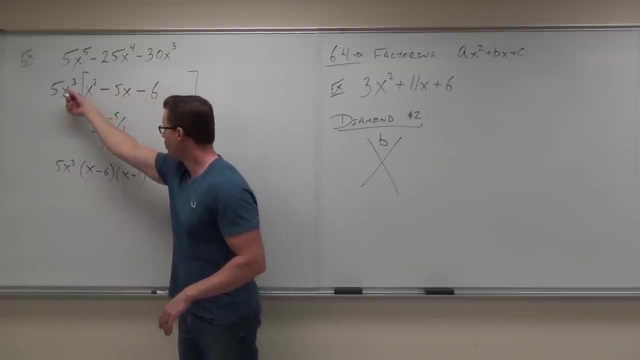 A, even though it's 1.. It looks like it's just a C, but it's 1 times. this goes here. Well, what's our A? 3. What's our C? 6. What's A times C? 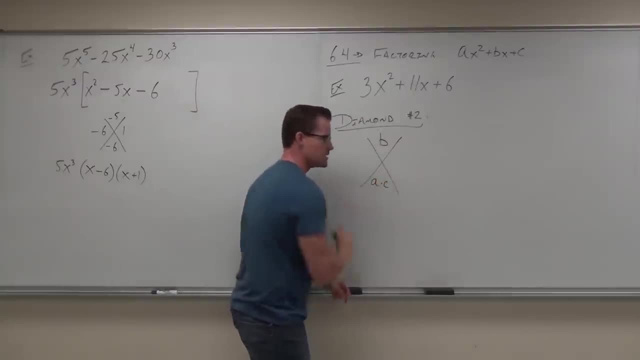 8.. That's what's going to go here. It's going to be A times C. that goes there. Same as before. It's exactly the same as before. So if you're okay with it so far, Well, you should right, because it's exactly the same as before. 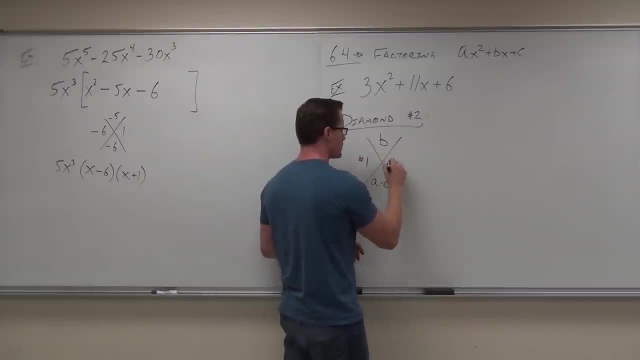 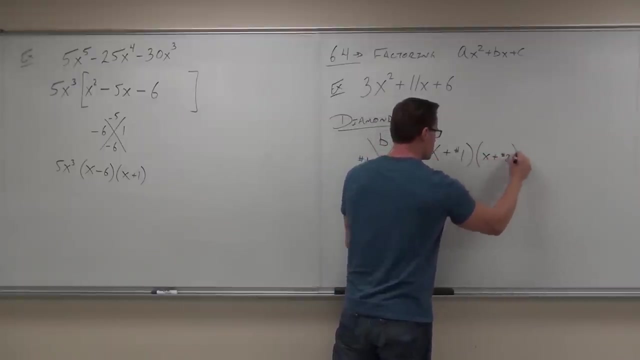 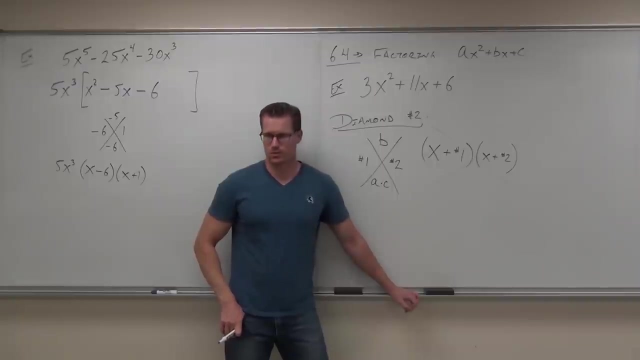 Now we're still going to find our two numbers, but what you're not going to do. you're not going to do this. Why not? Because it's not going to work. I know it's not going to work. Why wouldn't it work? 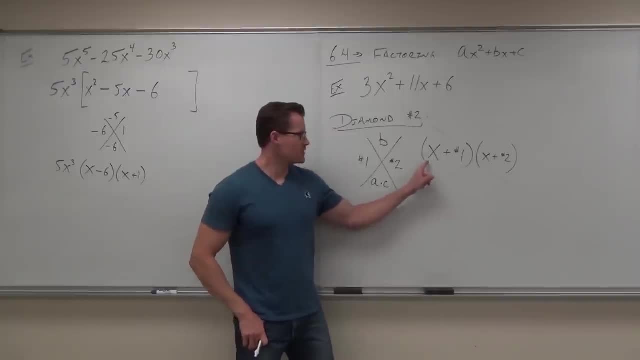 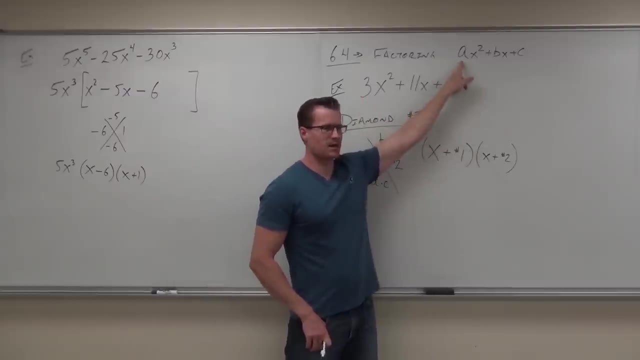 Because A is not 1.. Yep, Because if I do this, if I do X times, how much is X times X, X squared? I don't have an X squared. X times X is not going to give me my A back. 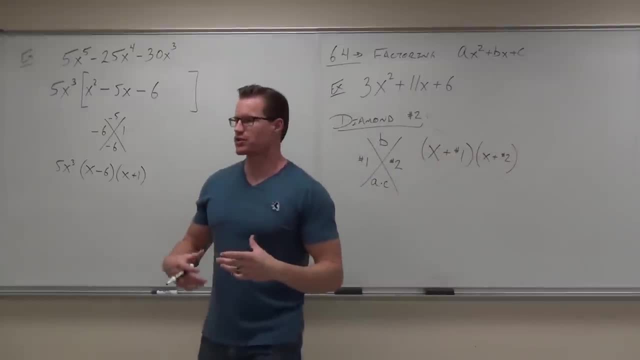 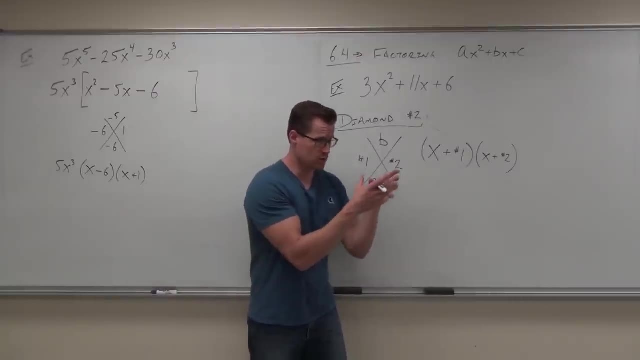 That doesn't work. The only thing that will work here is doing the factor by grouping, And that was the whole idea. That's why in the previous examples, the ones I gave you in the last section, that's why I said: well, you know, you can do it with the shortcut or, if you forget the shortcut, 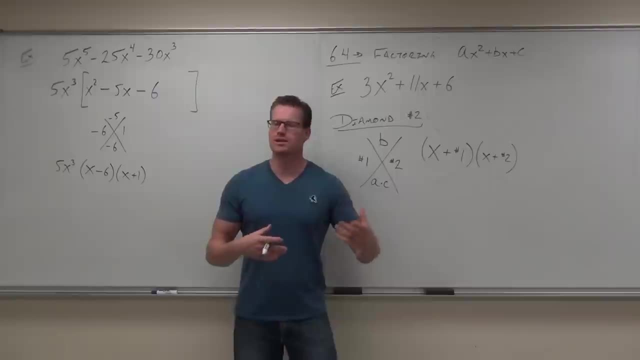 you can split it up and you can use the grouping. That is what is necessary here. There is no shortcut. This is the long way every time if your A is not 1.. So one last time. When can you go directly to your factors if A is? 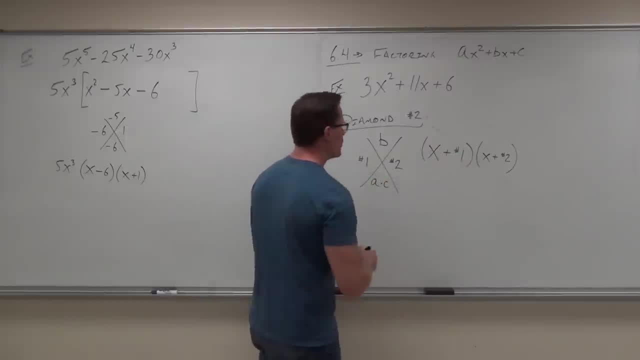 1.. If A is not 1, you have this method. Here's what we do. We do our. so this is for AX squared plus BX plus CX. It's a little redundant, So here's what you do. I've already done it for you in the last section, but again I'm going to show it to you here. 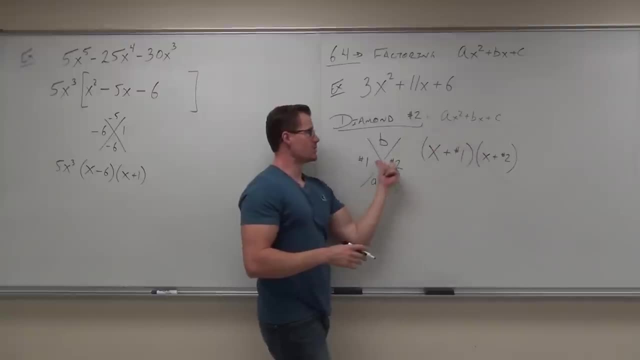 How many terms do we have? Three? We're going to use these two numbers to make it four terms. We're splitting it, We're splitting it up And the reason why we can do this, these two numbers have to add to this one, correct? 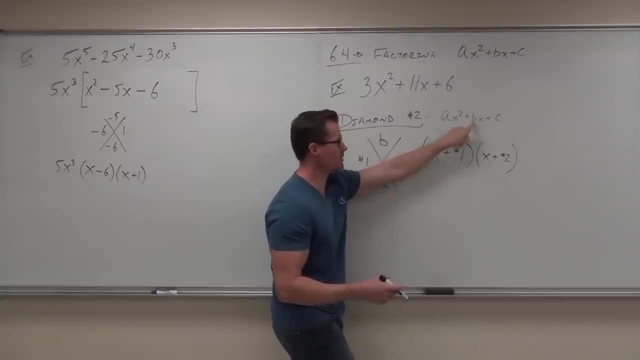 If they have to add to this one. that means I can separate this term, this B, into two different terms. So I'll have AX squared plus number 1X plus number 2X plus C, And then I'll factor by grouping. 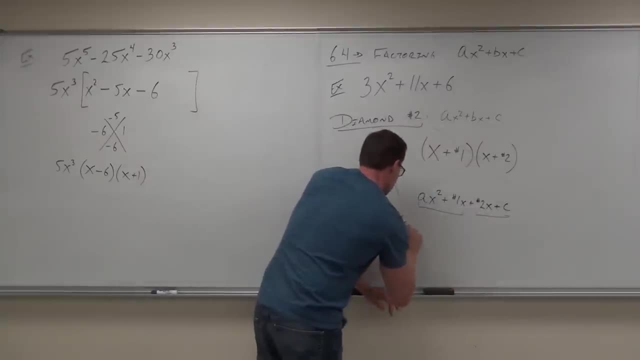 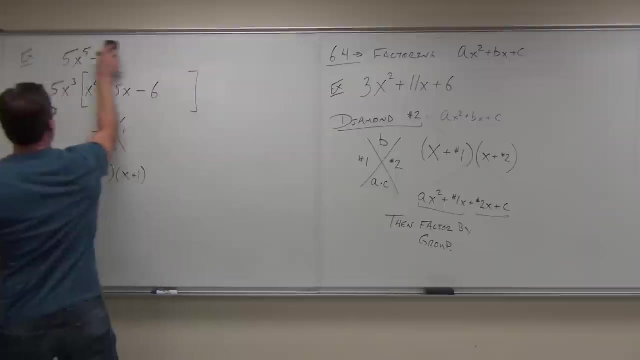 That's the whole idea. So let's go through this example, this example one time. I'm going to go kind of quickly. Next time we'll get a lot of practice, so bear with me here. I just want to make sure that I at least give you something before you leave and don't leave you hanging. 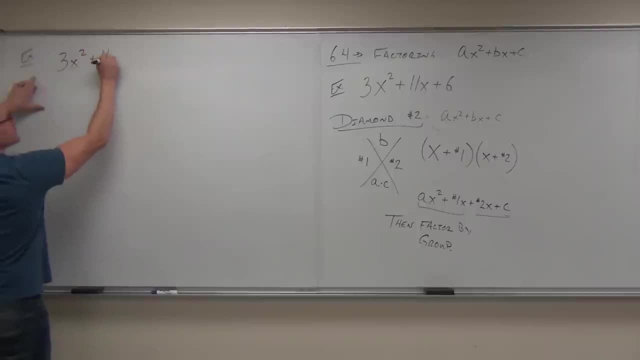 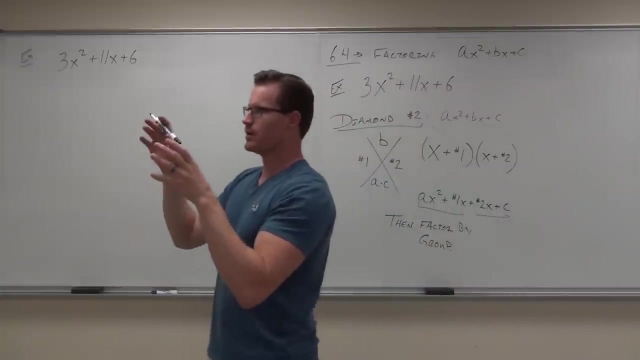 So 3X squared plus 11X plus 6.. Okay, Super, super fast. Is it in order? Yes, Is the first term positive, Yes. Yes, Do I have a GX? Yes, Do I have a GCF? 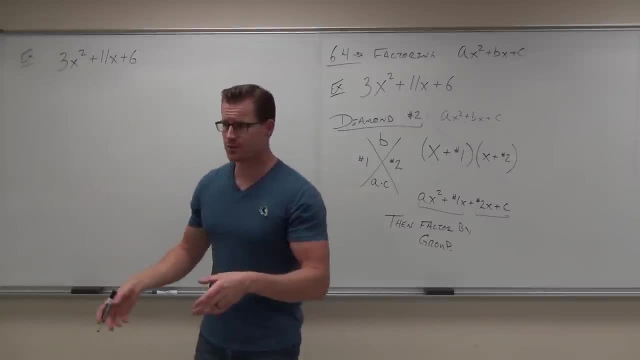 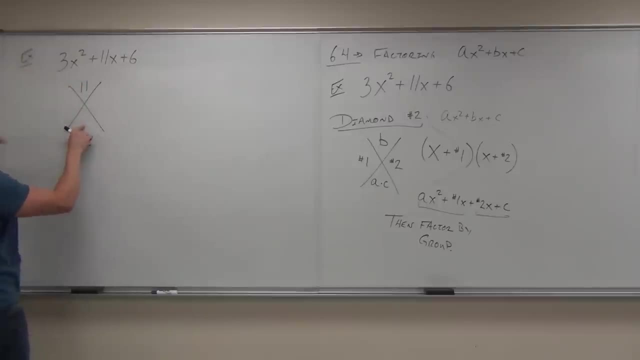 No, No, Okay, How many terms do I have Three? What do I use for three terms? Diamond, Diamond, That's always the process. What goes up top? 11. 11. Does 6 go here? No, 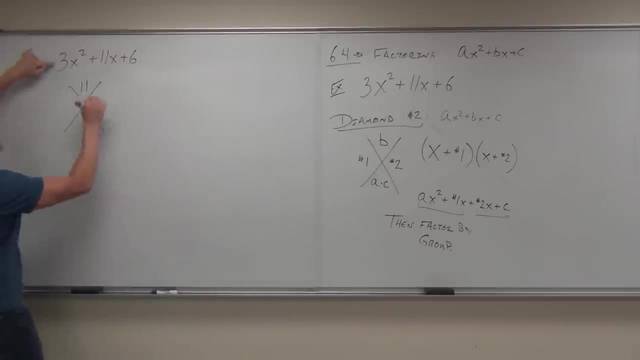 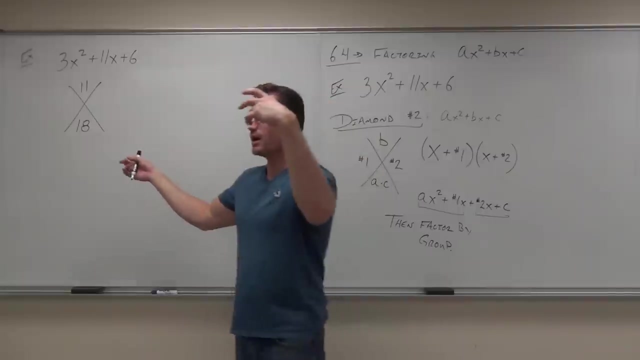 Why not? Because it's 8 times C. Okay, So A is 3,, C is so 18.. We are still going to find two numbers that add to 11, our top number, B, and multiply to 18.. 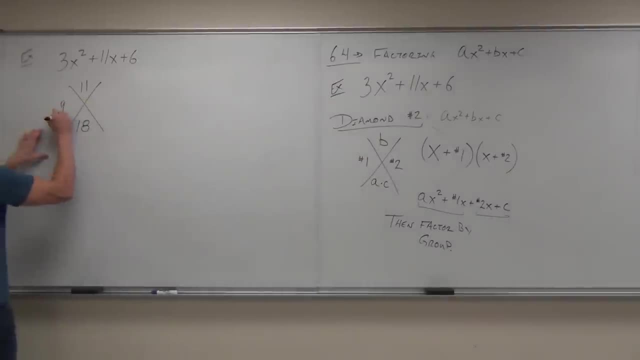 Can you think of that? Do I need 18?? Yeah, they're both positive, 9 and 2.. Would it be a good idea? It would be a good idea if I did X plus 9 and X plus 2.. 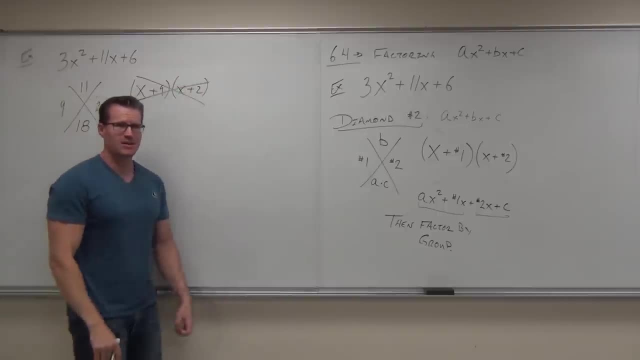 No, because it wouldn't give you the answer. This makes me sad. Don't do that. You're going to break my clerks. Don't do that. Okay, What this is is you only do this if A is what. 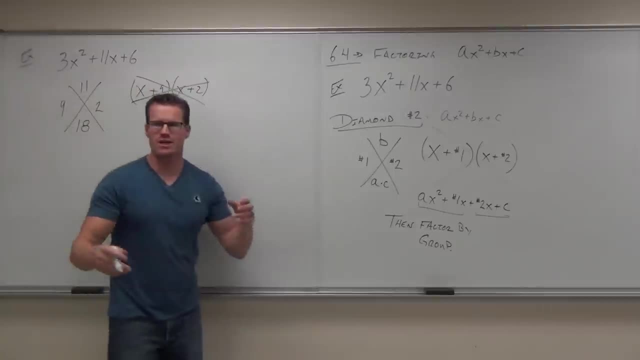 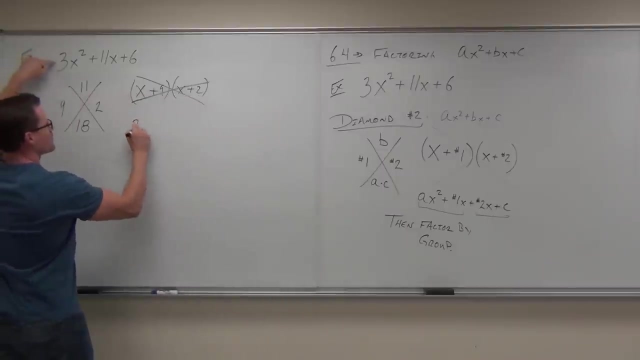 1. It's not 1.. Now we go through the group. Remember I told you, even if you forget about the shortcut, you can still solve the problem by doing the grouping, And that's what you have to do here. We keep the 3X squared. 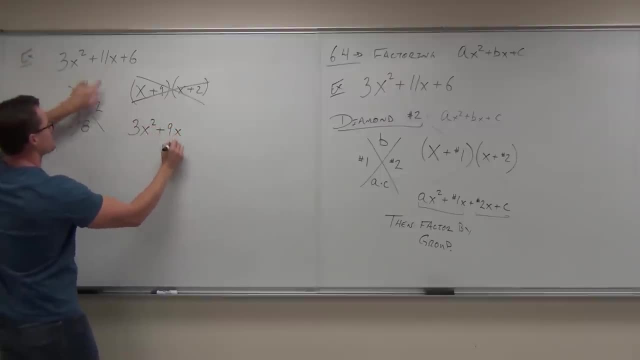 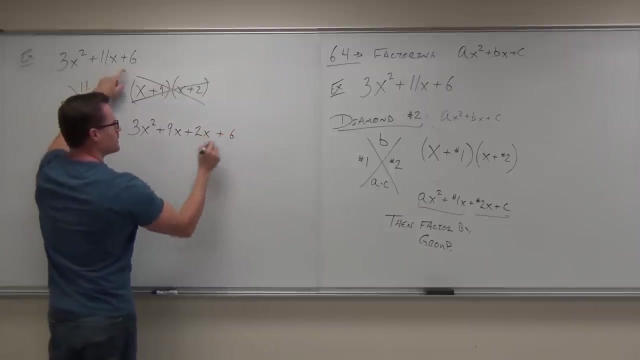 We're using these numbers to split this up: Plus 9X, Plus 2X. Notice, please, this is still 11X, Do you see it? Plus 6.. And then what we have? we change 3 terms into 4 terms so that we can do our grouping. 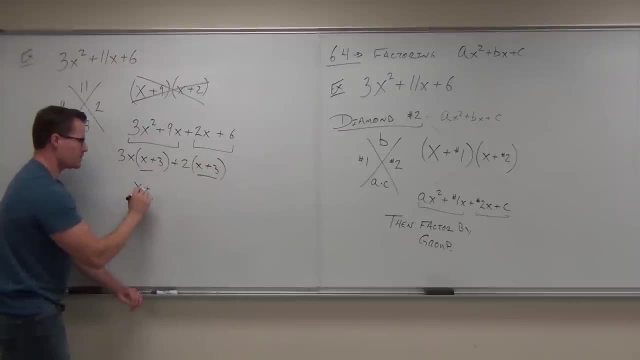 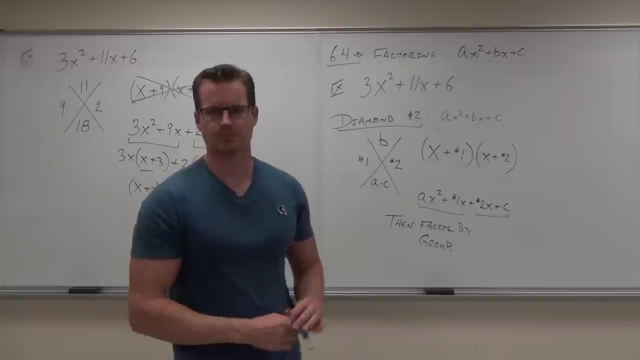 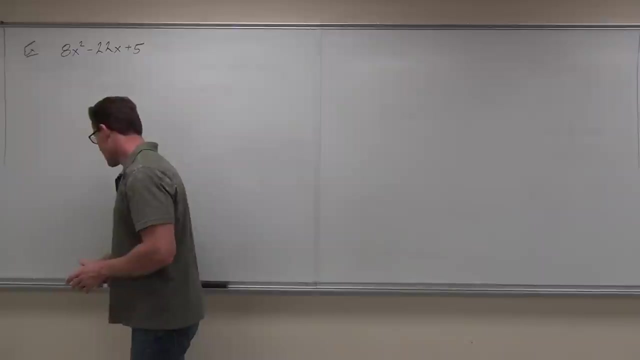 And this should be old stuff for us. We already know how to do that And we finish off with a vector And that's completely vector. So a continuation of factoring, and we're still factoring these type of problems. but I do want to make sure that you're going through the thought process every single time when 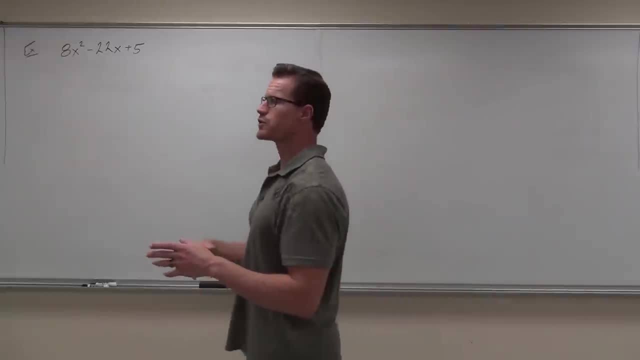 we see these. So, if you remember from last time, what's the first thing we check for? any time we are factoring anything, The first thing It's not GCF, The order, The order. Then we want to make sure that these things are on the correct order. 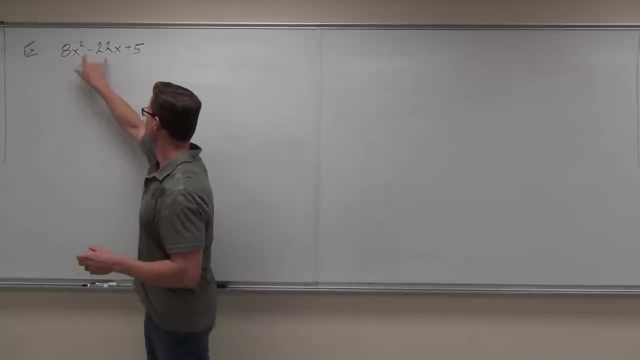 Is this an order? for us, Yes, Order means X squared X number, So is it an order? Yes. Next thing we check: Is the first term positive, Because if it's not, our techniques really don't work that well. 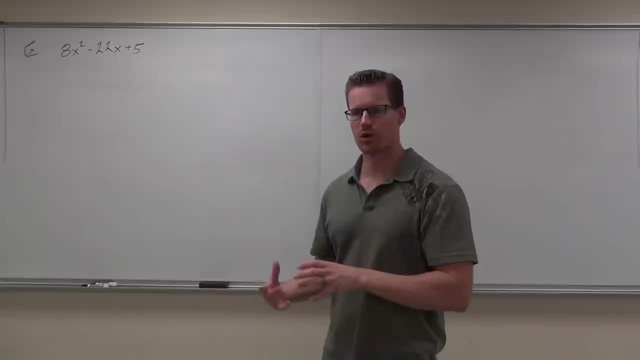 Is the first term positive, Yes, OK. If it's not, we would consider our GCF to be negative 1, and we'd factor that out. So when we're looking for a GCF, we're also kind of looking to see whether that's negative. 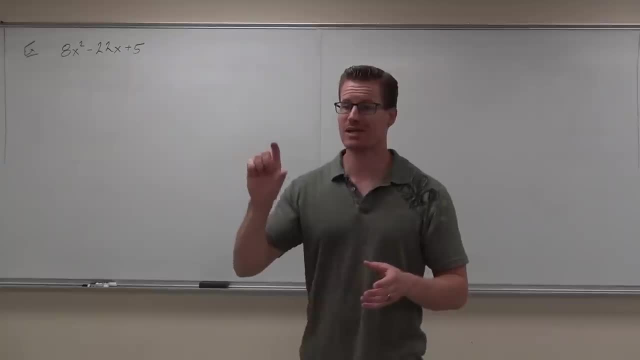 or not, If it's not cool. If it is, then we factor out that negative. Does this have a GCF besides 1?? All right, Then we start going on and counting the number of terms. How many terms do we have? 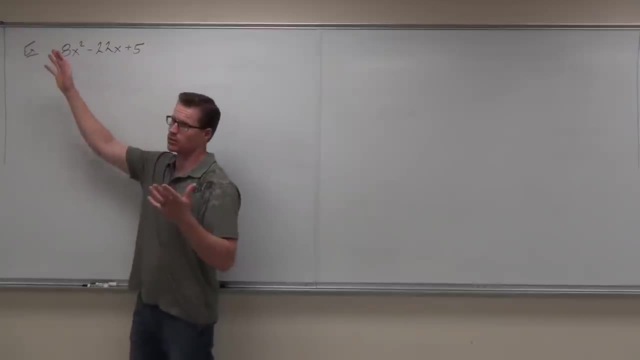 OK, And in your head, whenever you see 3 terms, you're going to start counting the number of terms. OK, And in your head, whenever you see 3 terms, you're going to start counting the number of terms. All right. 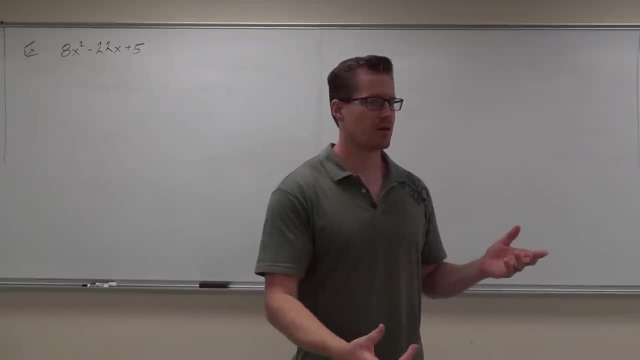 And in your head, whenever you see 3 terms, you're going to start counting the number of terms. I'm going to start counting the number of terms. OK, And in your head, whenever you see 3 terms, boom goes off. 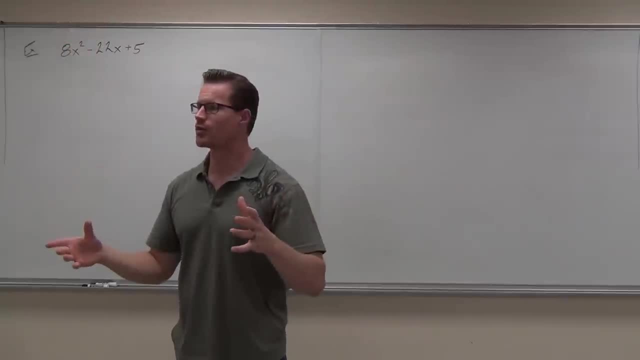 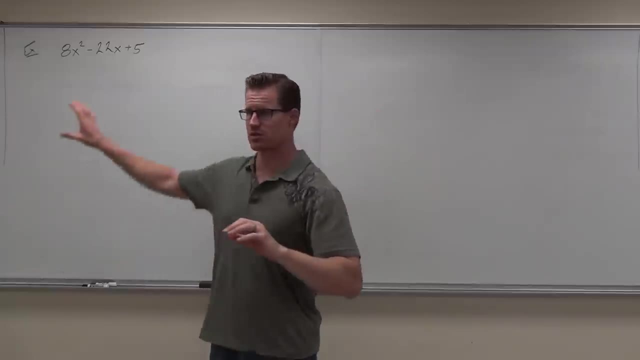 Diamond Diamond, So diamond method. Now, from before we have 2 kind of types of diamond method. We have one where we can do a shortcut and one where we can't. Which one is this A shortcut or no shortcut? 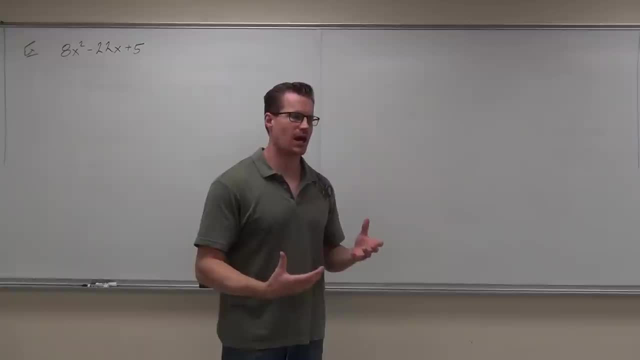 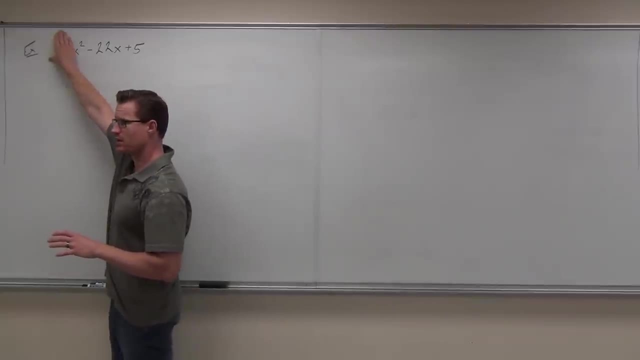 No, OK good, But you have to understand that the process is identical. It's the same thing, It's just. if this is not there, we have a shortcut that we can choose to do. You don't have to do it. 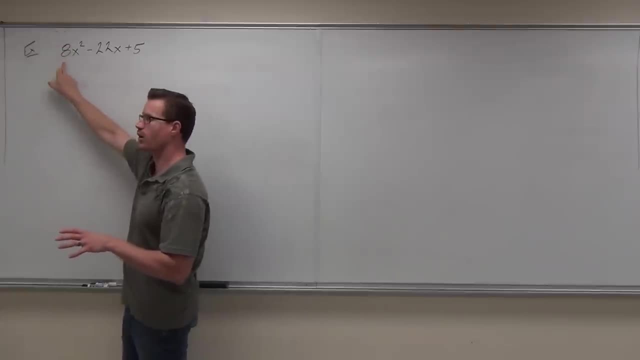 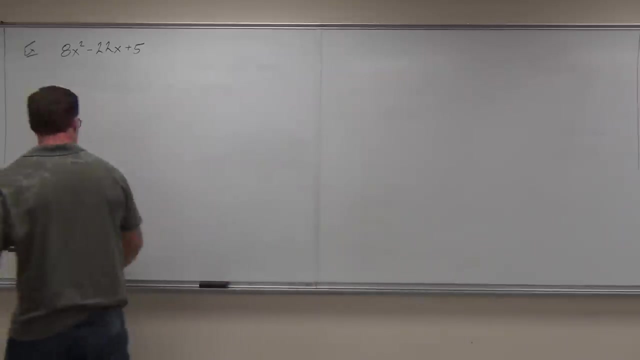 You can choose to do it. It makes your life easier. If that is not one, then we don't have a shortcut. There's nothing else to do besides what we're doing now, just the grouping idea. So let's go through two examples together. 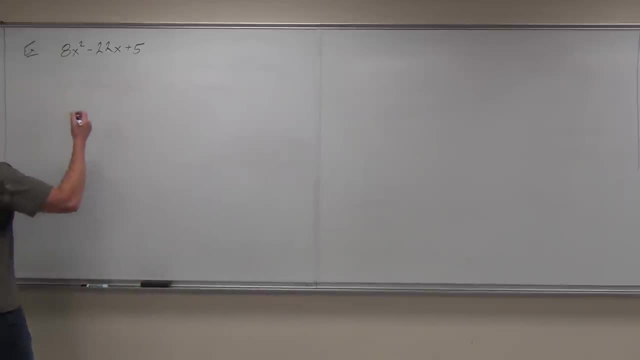 And, like I said, I'm going to give you a couple to practice right now. So diamond problem: absolutely Tell me what number goes up top, please 22.. I like how it goes with the sign, so negative 22.. 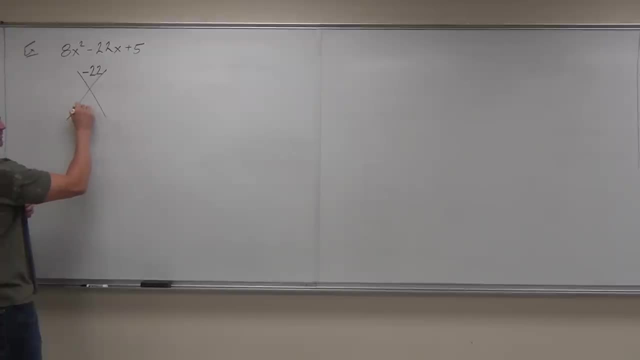 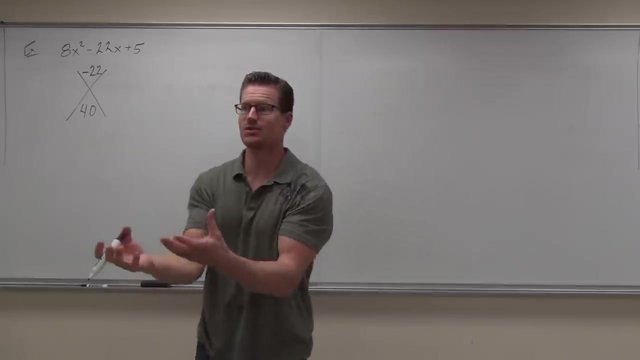 True or false? 5 goes here. No. What goes here? 40. 40. And then we start thinking about two numbers which add to negative 22 and multiply to 40. And remember, I can't do this for you all the time, so you're going to have to be good at that. 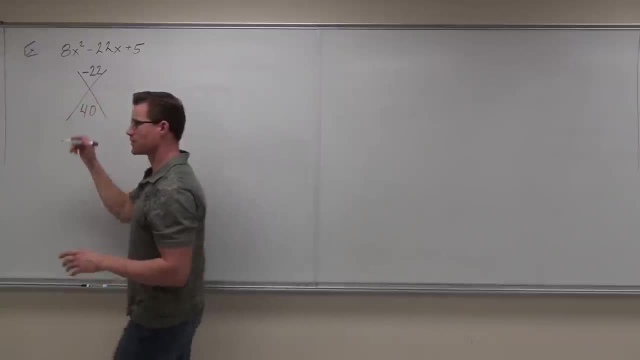 I've taught you the tricks. okay, If that's a positive and that's a negative, these are both negatives, Negative 2 and negative 20.. Negative what? Negative 2 and negative 20.. That's a kind of nice one. 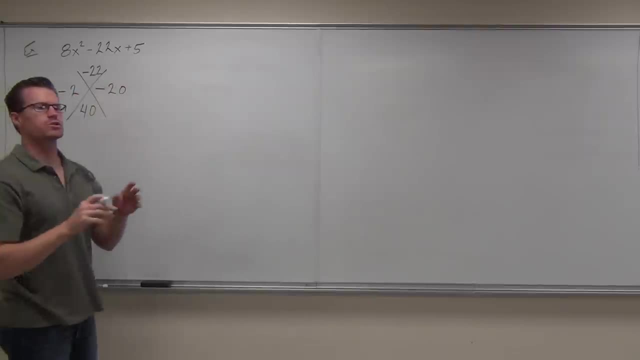 Negative 2 and negative 20.. That's right. We double check before we go any further. So negative 2 plus negative 20, we know that's negative 22.. And if I multiply those two numbers it's positive 40.. 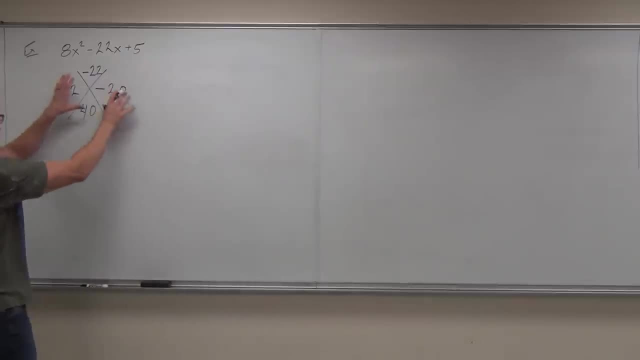 So I know I'm going to go. Don't go any further until you're sure that those are right Now. after that, you know what? I asked it to you or asked it of you, but I want to make sure you know it. 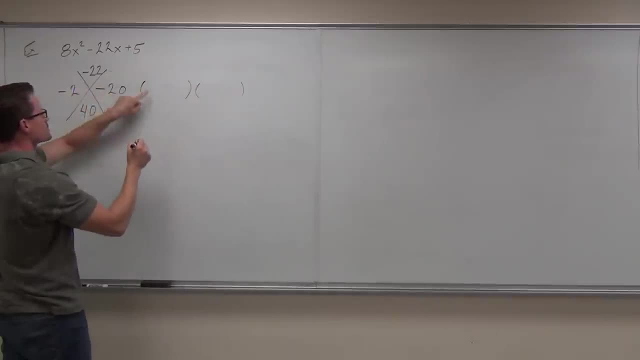 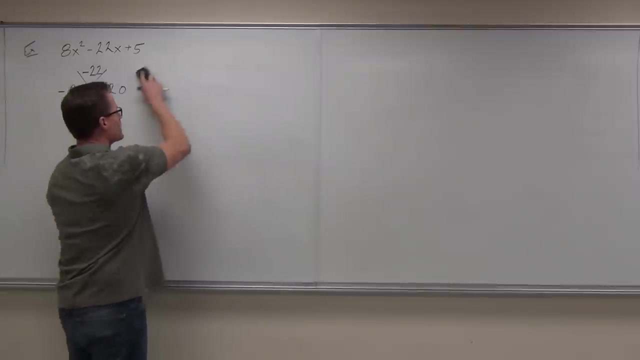 Can I go and do the shortcut right now and just do x minus 2 and x minus 20?? No, it's going to fail having the 8x squared. It's going to fail having even the 5.. So what that should tell you is: oh my gosh. 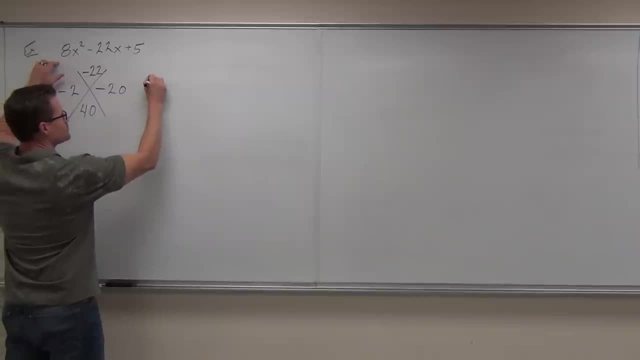 Well, yeah, There is no shortcut here. We're just going to use those two numbers which add to your b to split up that middle term, Changing three terms into four terms using the two numbers that you just found, And the whole reason why we're doing that, why we're changing three terms into four terms. 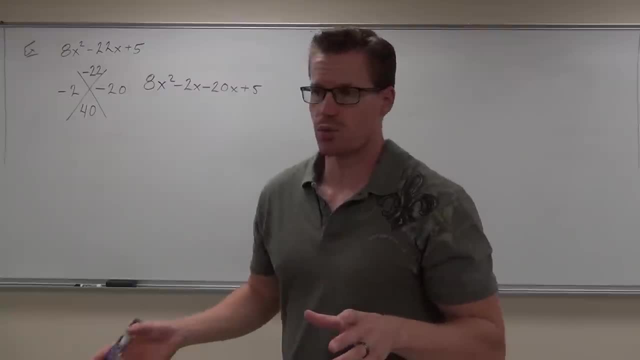 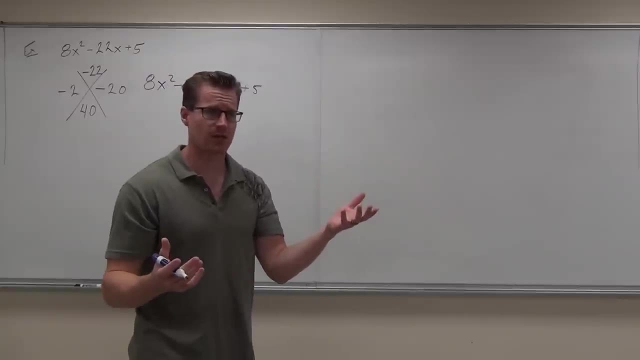 is because we learned how to factor by grouping really well, So why not take advantage of that? So changing the four terms, and then it's not bad. You don't have to guess and check. There are other methods to do this. I'm not going to lie to you. 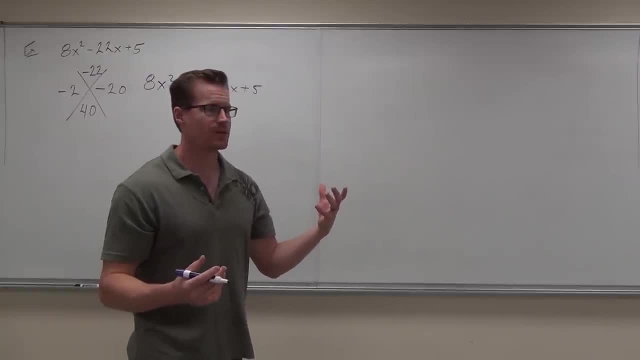 There are. Some people can do these in their head and that's cool, But this is kind of a fail safe that gives you the right answer all the time, and that's really what I'm looking at for: you guys Get the right answer all the time and give you a way that's mathematically relevant. 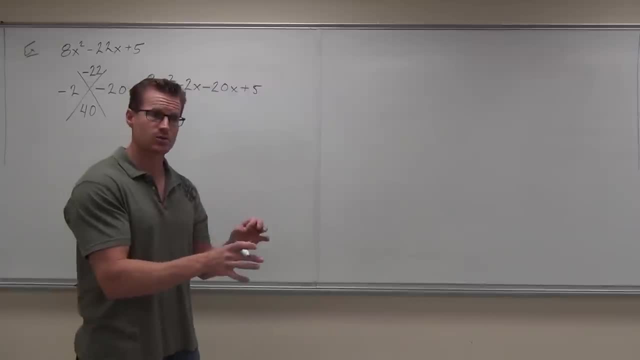 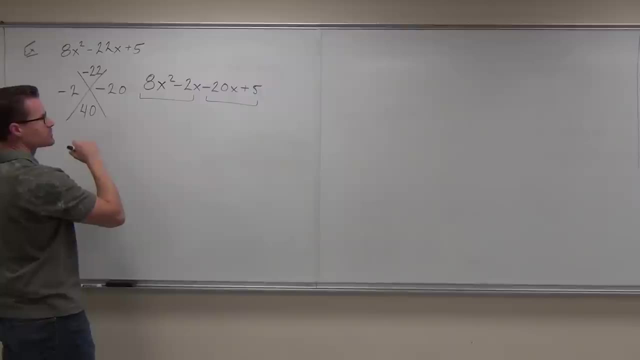 that you can follow the math and not just do a little trick. And there are some tricks that actually work, which is awesome, but I want to give you a way that you understand. So, factor by grouping. I'm not going to patronize you by having you do it every single time. 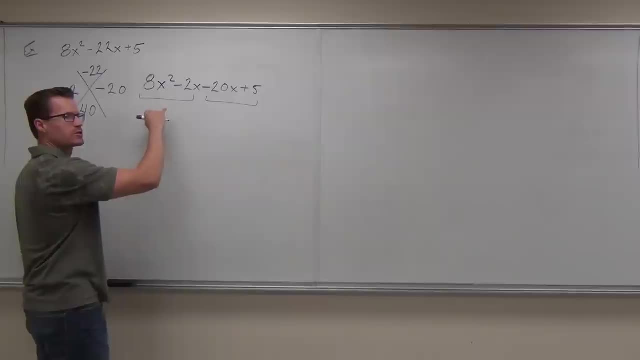 It's going to take a little bit longer. I'm just going to walk you through it. So factor by grouping. I'm going to assume that you can factor GCF at this point with no problem, because it's been like two weeks and we should be pros of that right now. 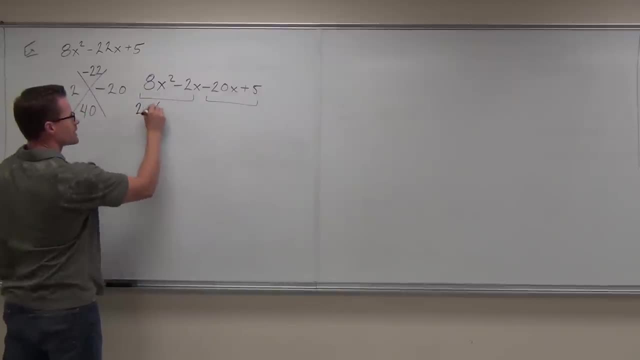 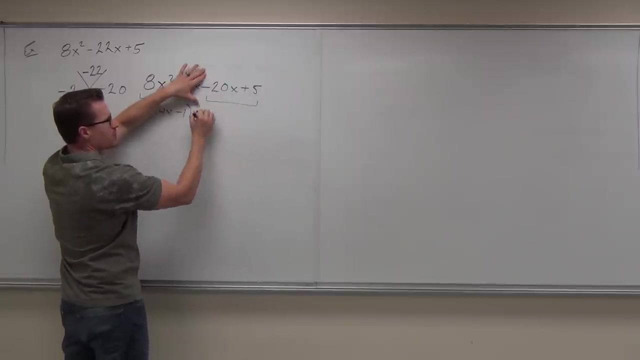 So we look for the biggest number is 2.. The biggest variable that's shared by both is x. We get 4x and we get minus 1.. Here we're looking at the number. There's no variable to share, but the number is 4.. 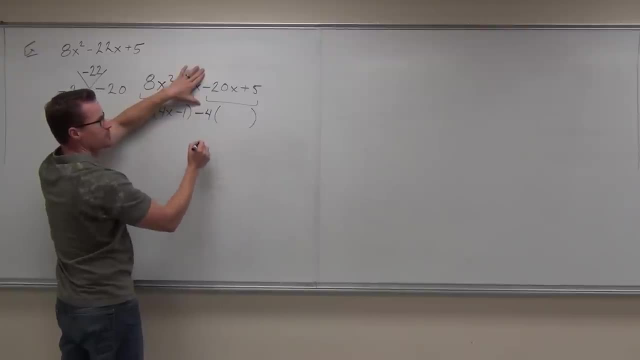 That minus forces me to factor out a negative 4, which simply means my signs are both going to change. This becomes a positive. It's pi over 4.. Sorry, I didn't do the math in my head. Pull out the 5.. 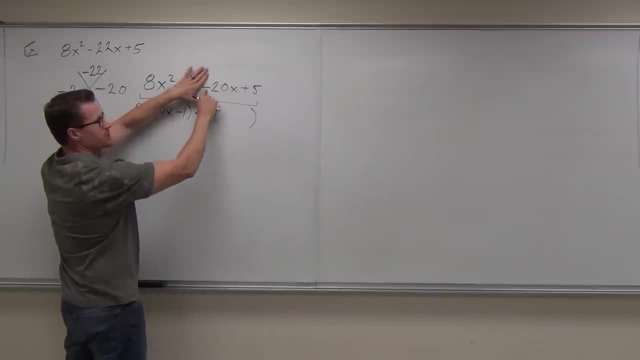 I was thinking about this one already. So 5 goes into both those numbers. This forces you to factor out a negative 5.. What that negative is going to do is change both these signs. So this will be positive 4x. This will be minus 1.. 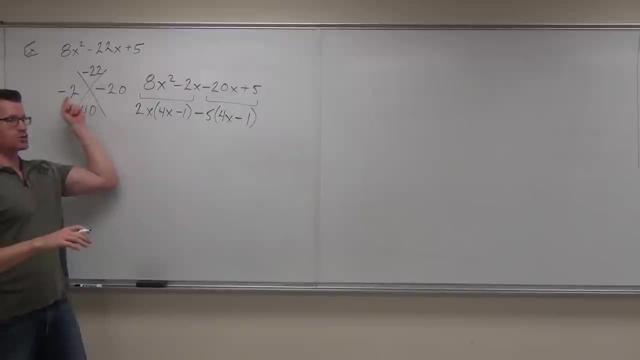 Here's how you know if you did it right. If you can do this and you're sure you're right, this has to work. It has to be exactly the same, okay? So if you're finding out, man, that's something different. 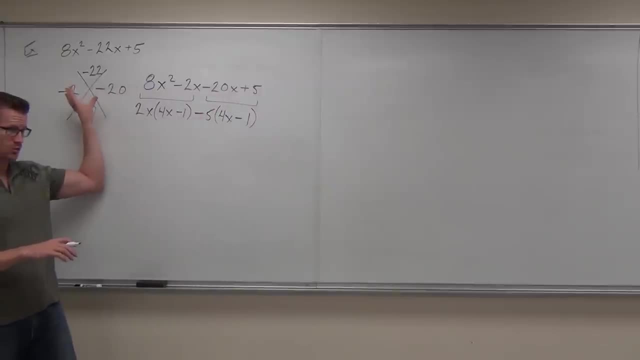 You made a mistake here, Not here. Okay, if you check this, double-check it and you're right, then your mistake is coming up here. Okay, and that's where you need to focus your work. So we have two big terms. 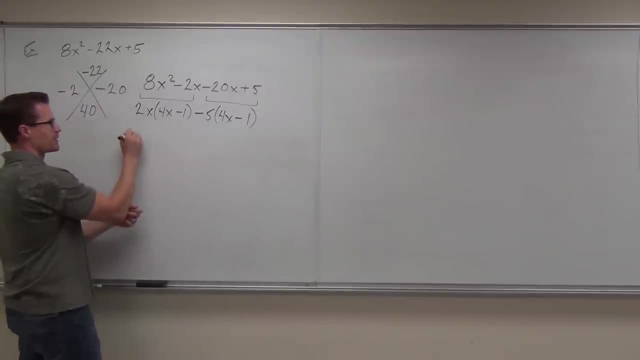 I know factoring by grouping says if there's a common factor, we divide that out, create a new set of parentheses, because we're factoring. Once we divide it, we put the remaining pieces of those terms, the remaining factors, in that second parentheses and it's completely factored. 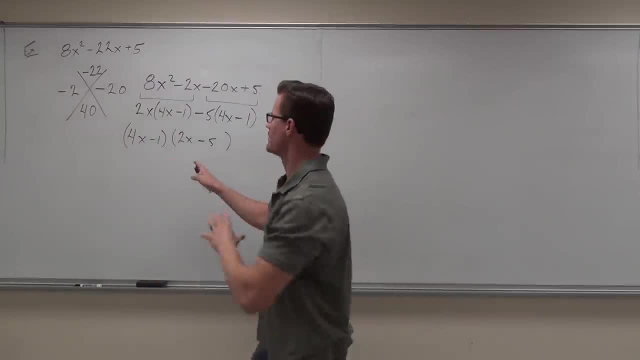 We can check our work by some simple distribution. Just FOIL it and it's got to be exactly the same as we started with. If it's not, then you've made a mistake. Quick head-down if you're okay with it so far. 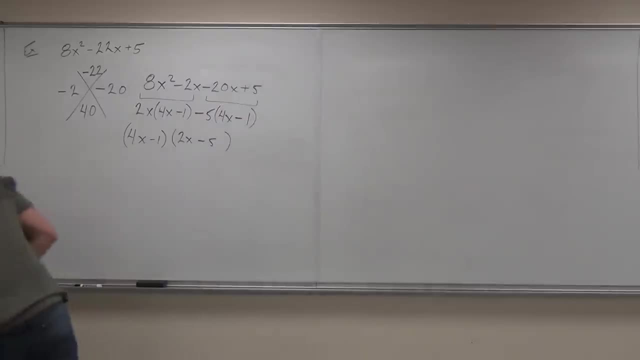 Okay, let's do one more, but I want you guys to guide me through it. okay, I want to know if it's getting easier for you. This might have started off like, oh my gosh, Is it getting easier as we're going through it? 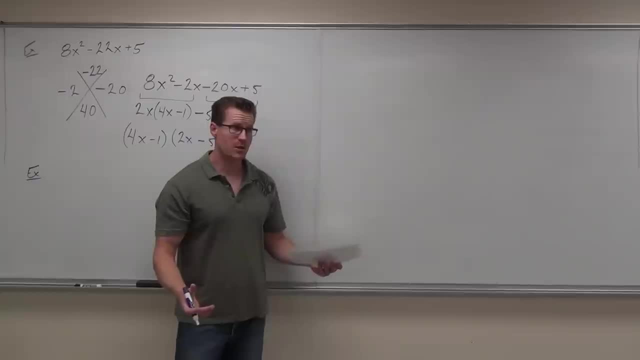 The more practice you do, the easier this becomes, until ultimately, in Chapter 7, you're like: oh yeah, that's just one small part of what we're doing here. That's what I want for you. Yeah, not where you've got to worry about it. 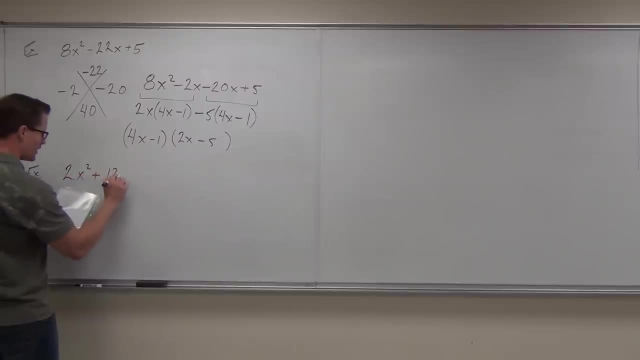 Oh, my gosh factoring again. Well, you might still do that, But at least you're going to be able to do it. Okay, so we're going to quickly walk through this problem and I'm going to give you something to do on your own. 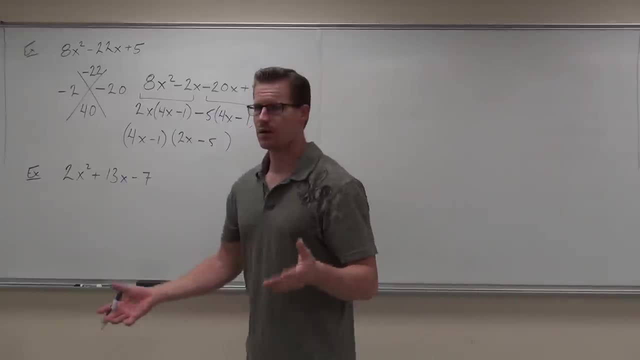 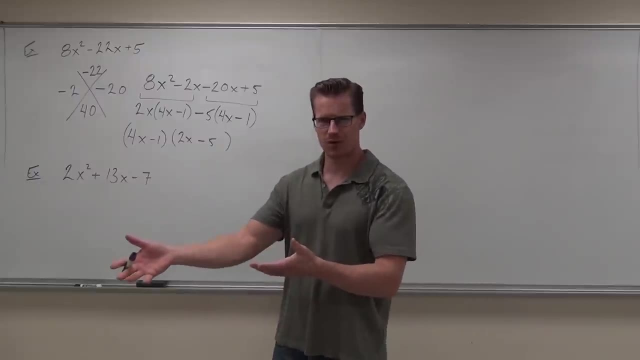 So first thing we check for what is that? Is it an order? Second thing we check for first term: is it positive or negative? That's great. Do we have a? what are we looking for? Is there one? Okay, next thing we check for is what? 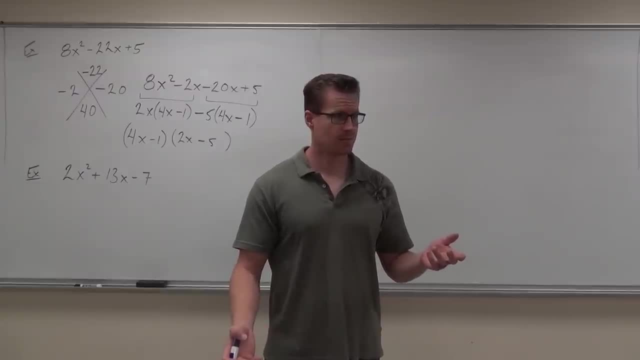 Why are we choosing the diamond method here? Good, Is this going to be a shortcut diamond problem or a long? or is this going to be a standard diamond problem? Long, Okay, so let's go ahead and do that together. What number goes here? 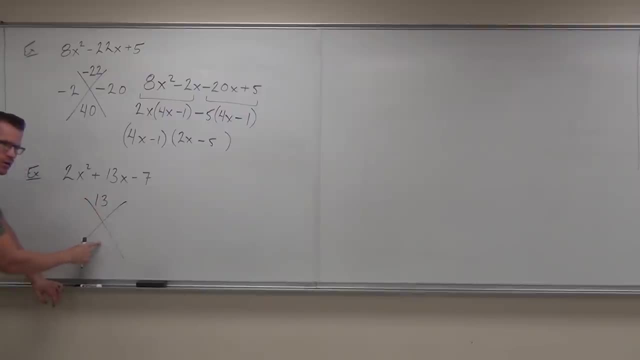 Thirteen, What number goes here? Negative 14.. How are you finding the negative 14? Negative 7 times 2.. Okay, so the A times the C is exactly right. And then we find two numbers which add to 13 and multiply to negative 14.. 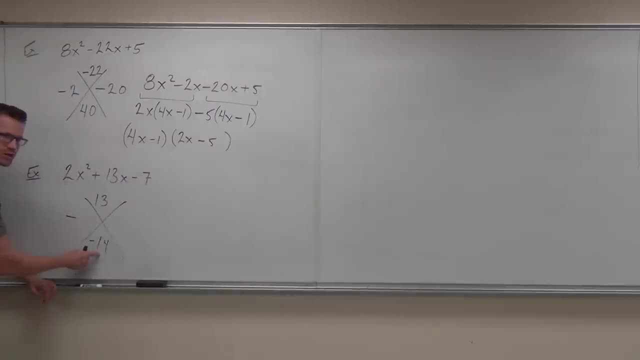 Of course, if you look at it, one of them has to be negative, because you're multiplying two in negative. That's the only way that that can work. So two numbers that multiply to a negative, whose difference is 13.. These numbers have to be separated by 13.. 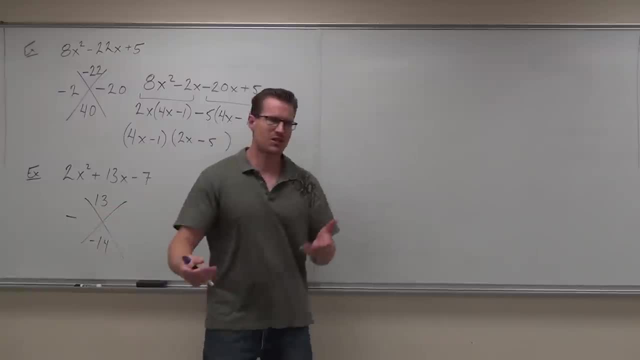 Well, can you think of it? One and negative one, Fourteen and one somehow, where the bigger one is positive. So 14 and negative one. Not negative 14 and one, but negative one and 14.. Let's double check. 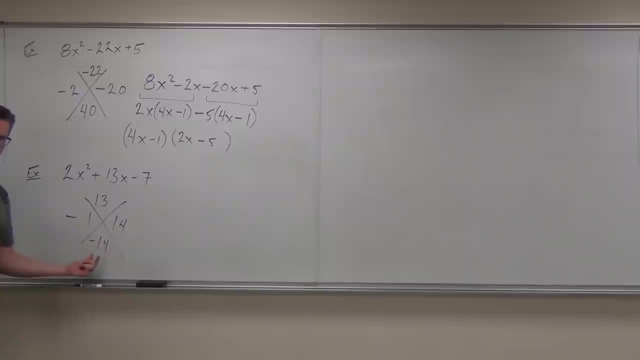 Does this add to positive 13?? Does it multiply to negative 14?? And trust me on this one, You're going to want to check your work before you go any further, because if you're going to do this, you're going to want to do this. 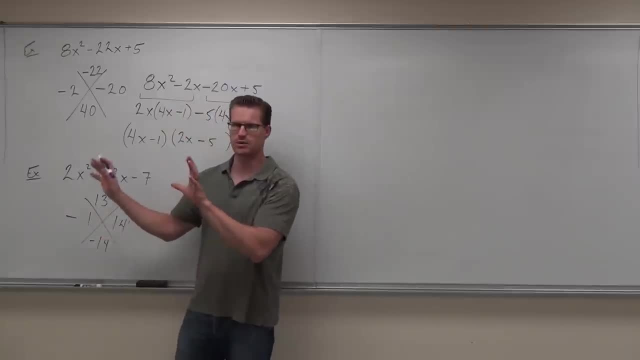 You're going to want to do this. If you mess the sign up and don't check it, your problem is smoked. Okay, you're done. So please check that. Okay now, I asked you before, but can I go directly to my factors with my shortcut? 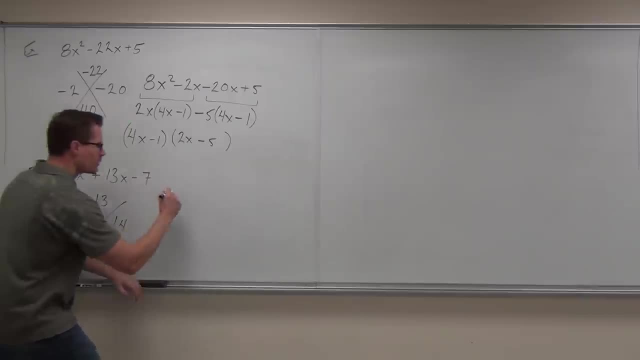 No, this is the. since the a is not one. we have to do the long way. So long way is: take those two numbers. allow them to separate your middle term Minus 1x. I don't have a 1.. 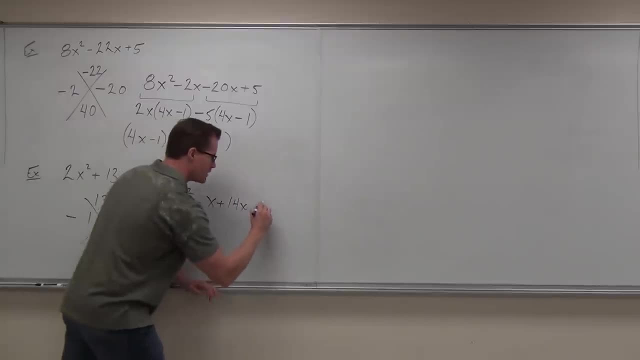 Minus x is minus 1x, Plus 14x Minus 7, and then we're going to group it. I'm going to go a little quickly on this, because I'm going to give you the opportunity to do this on your own in just a minute. 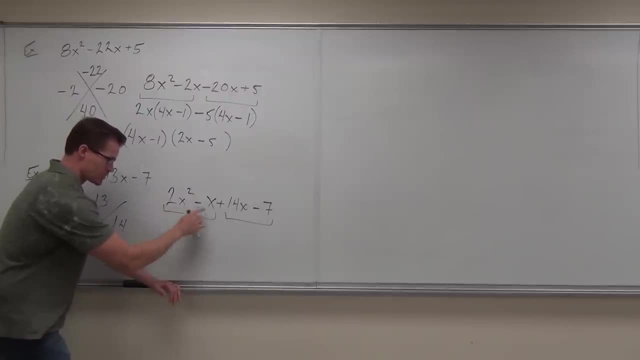 Grouping. here the only factor that goes into both those terms is x. We get 2x minus 1.. Here that says plus. I'm factoring on a positive number. No signs are going to change it when you factor a positive 7.. 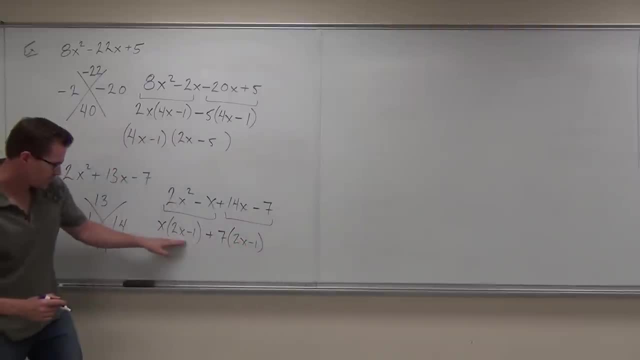 That will be 2x minus 1.. I'm going to check my work real quick. If I have the same thing, I know I've done it right and that's great, So let's factor that out. We get 2x minus 1, and the remaining factors from these two large terms. 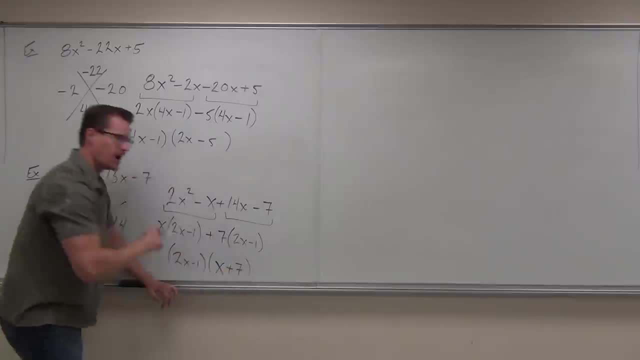 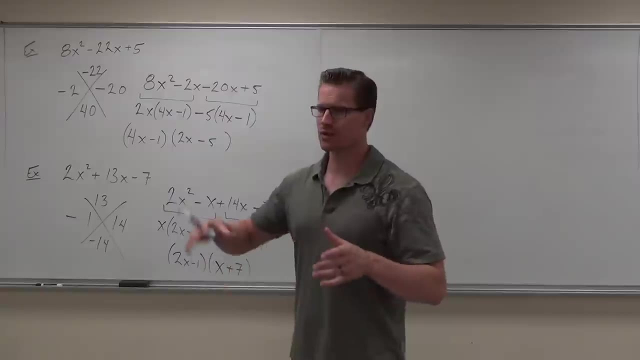 after I divide it by 2x minus 1, is x plus 7.. I would double check that with distribution if this was a test, to make sure that I have that right before I go any further. Show of hands, if this is making really good sense to you. 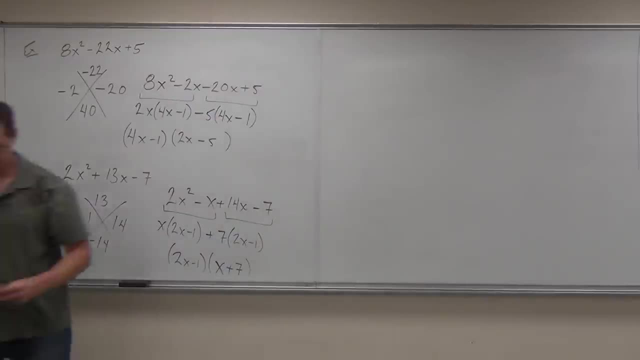 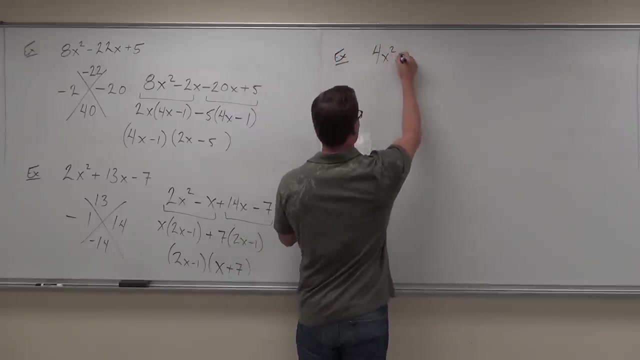 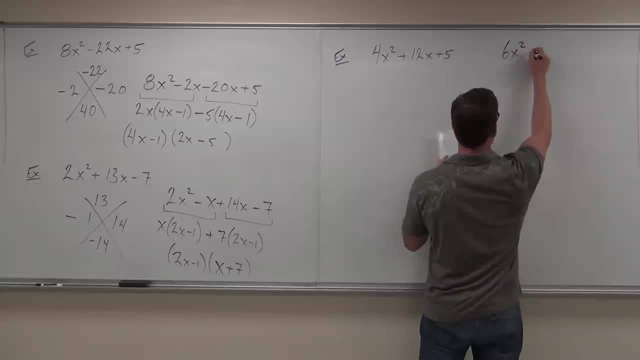 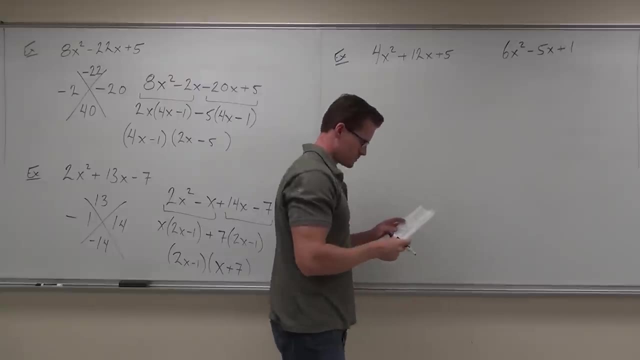 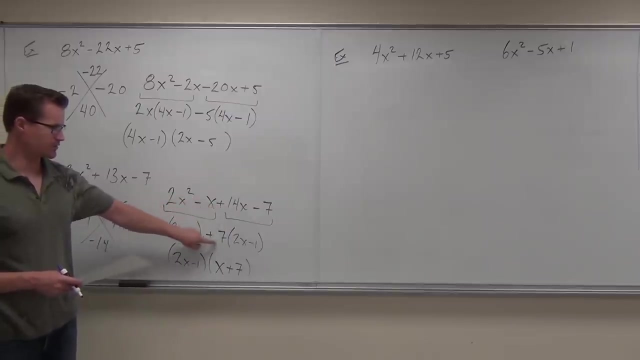 And let's do this one. We are vectoring a positive rate here. We're vectoring positive 7 out of there, because it says plus you have to factor a positive 7. So divided by 7, you get 2x. 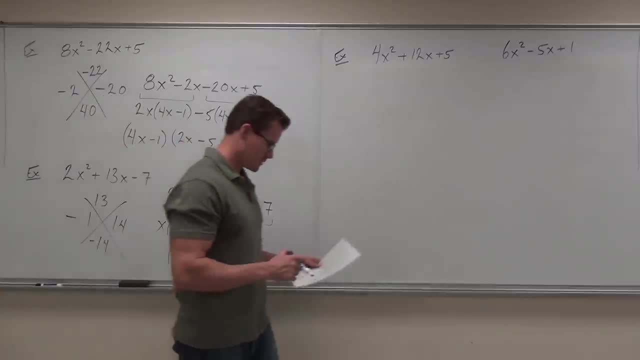 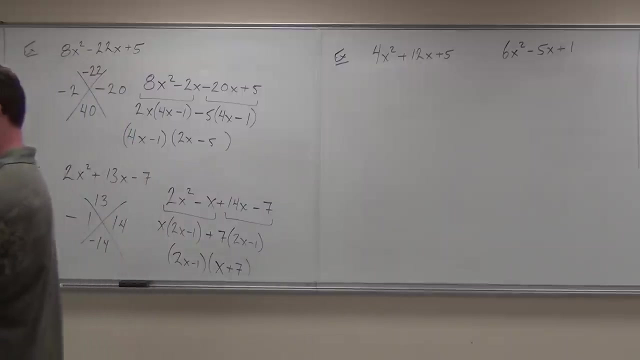 Divided by 7, you get 1.. We're dividing, We're dividing. So we check the order. Check negative out front. if there's not one, Cool Check for GCF. if there's not one, No problem. Check the number of terms. 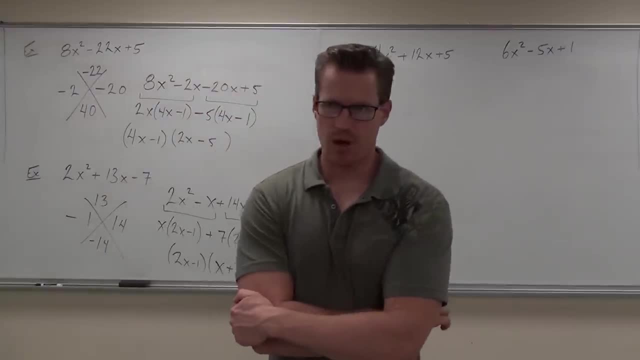 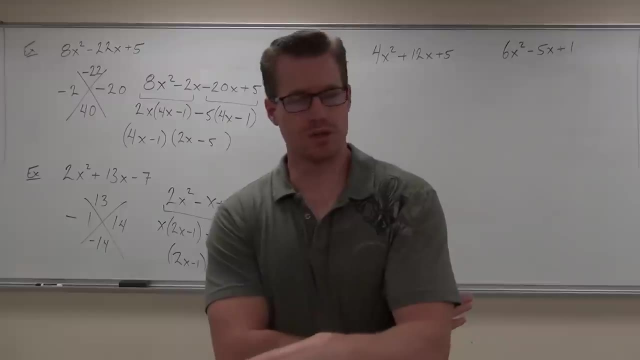 Three terms: Diamond problem. Remember that a diamond problem only allows you to break it up, to make it four terms to allow you to group. So really we're trying to get to grouping. So use a diamond problem to allow you to make four terms out of it. 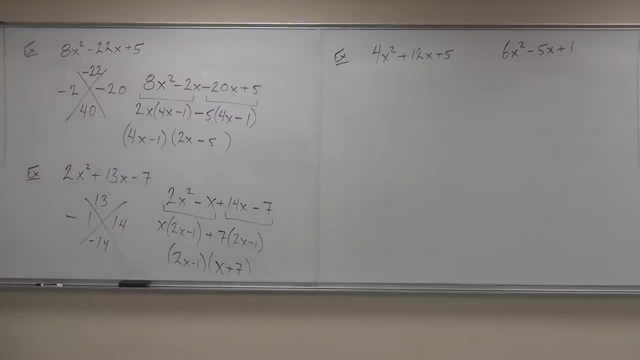 Okay, I'm going to get started up here. So these are both in order. They both have the first term, positive. You have to have that. There's no GCF in either case And there's three terms which, when you see, 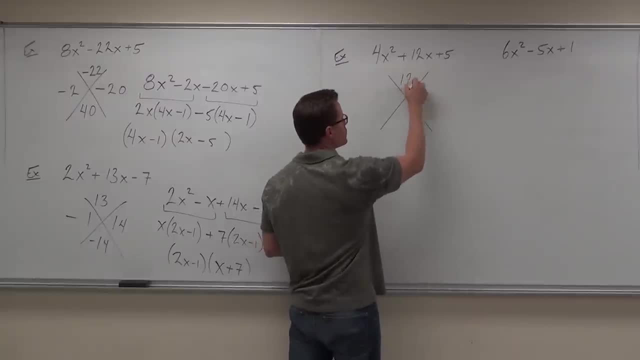 this is on a test and I say factor, you're going to do a diamond problem. So this is 12, and we're going to get 20, because we have the A times C gives us 4 times 5, or 20.. 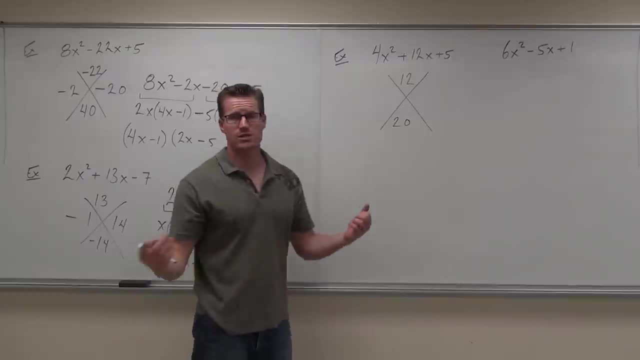 Now two numbers which add to 12, multiply to 20.. What's nice? they're both going to be positive. They're both positive numbers. So here we have 10, and we have 2.. Does it matter the order in which you have those? 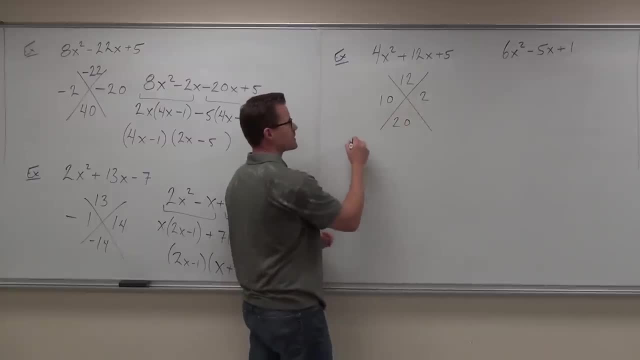 It doesn't matter, It's going to factor either way correctly. So what this does- because we have an A that's not 1, it says: all you've basically done is set this up so that grouping will work, and that's the whole plan. 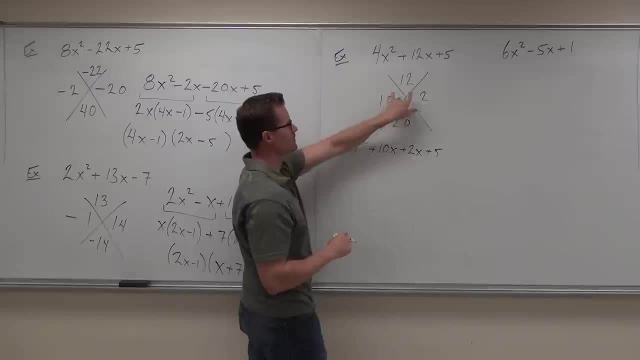 So we've got our 4x squared. cool, We're splitting this up: 10x plus 2x plus 5, and then we group it Here. we've got a 2x and we've got 2x plus 5.. 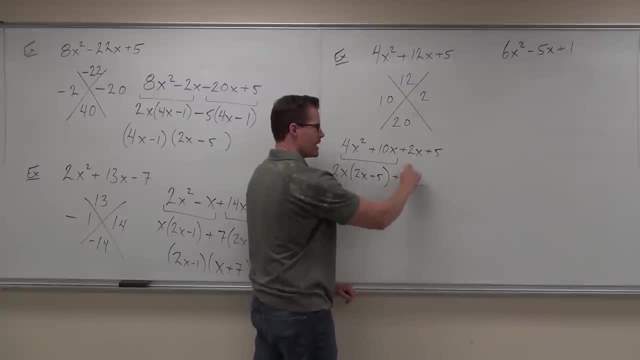 Here we wait a minute Switching. Do you have to switch them? Switch the 2 and the 10x, You can. Can you say plus 1 and then have 2x plus 5?? Sure, yeah, What goes into both those numbers? 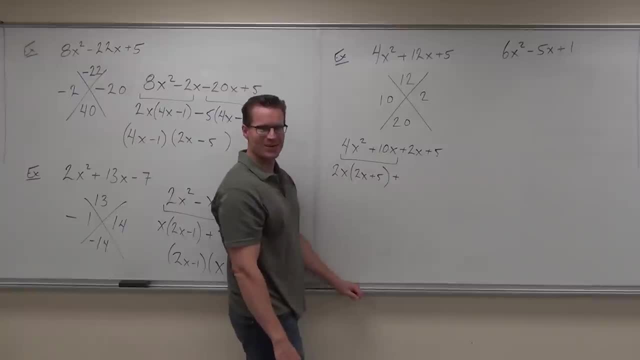 Nothing. 1. Don't you tell me nothing? What divides both of those terms? 1. Yeah, put the plus 1. If you factor out 1, yeah, it's kind of trivial because it doesn't do anything. 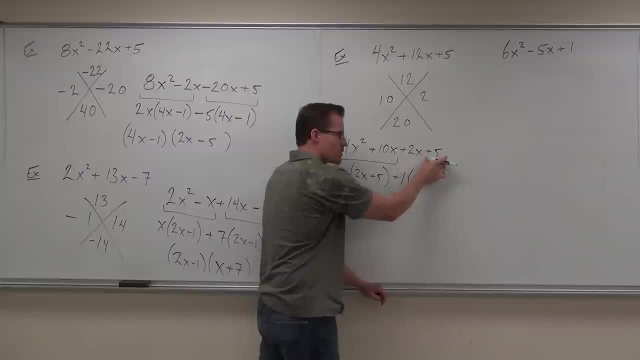 but you've seen this a couple times now- where, if nothing divides both those terms besides 1, put the plus 1.. It's not going to change then, but it will allow you to see that you have the same factor here and when you divide out that factor. 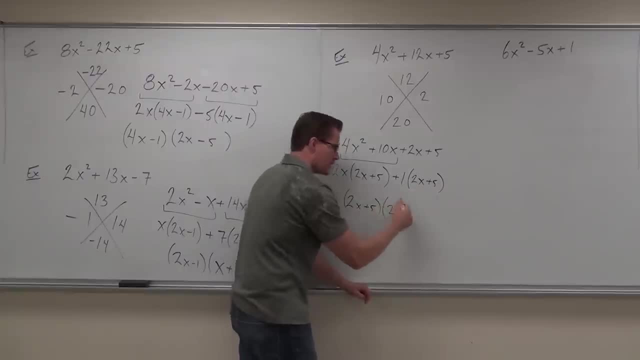 you don't have nothing. You have a 1.. You have a plus 1.. If you change those around, if you switch those around, will you get the same answer? Yes, Yes, it'll just be out of order, Does that matter? 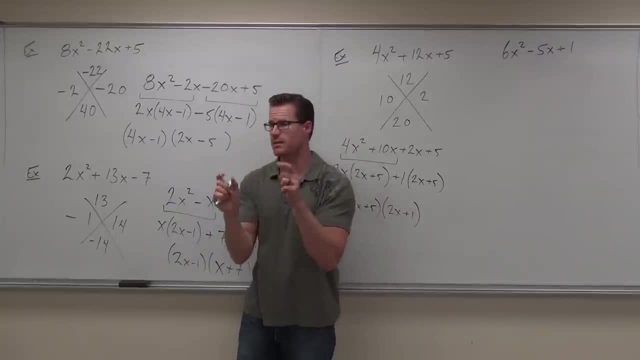 No, it doesn't matter. Okay. multiplication is commuted, so it does not matter, Okay. next one, By the way, how many people got that one? That's really good. If you guys keep this up, you're going to be pros at factoring. 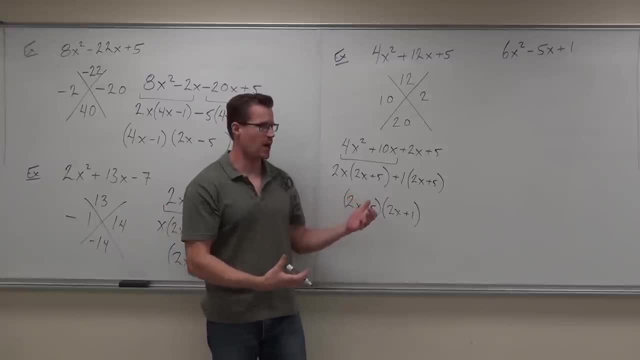 Okay, this is great. If you're having, if you're struggling with this, take some practice. Actually, everyone's going to take some practice, but keep up the practice If you get the idea of factoring. that's what's important. 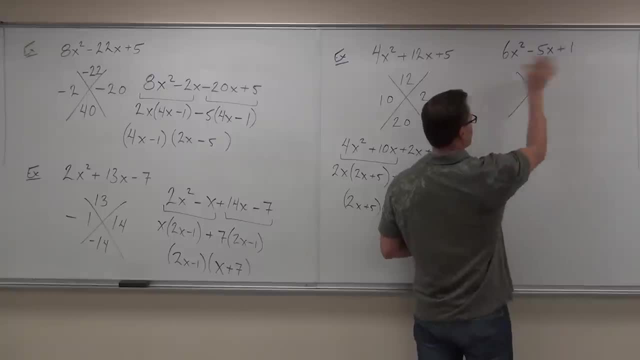 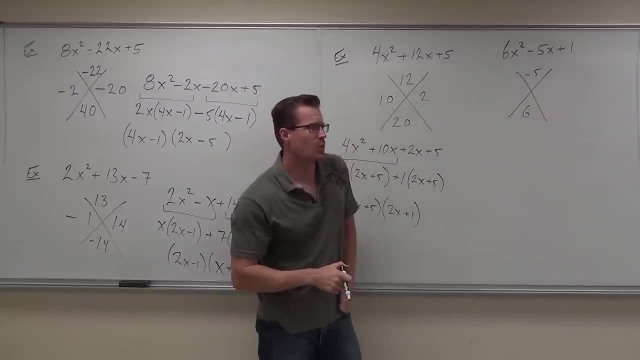 Okay, next one. So it's in order, no problem. no, GCF, put your negative 5,, put your positive 6, and think of a couple of numbers which add the negative 5 and multiply to positive 6.. Keep in mind: what do you know about the signs? 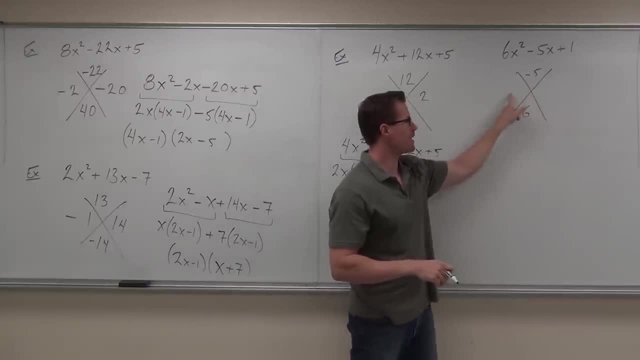 of both of these numbers. If 1 is positive and 1 is negative, what would that be? They're both negative. If they're both negative, will 6 and 1 work? Oh, will 3 and 2 work? 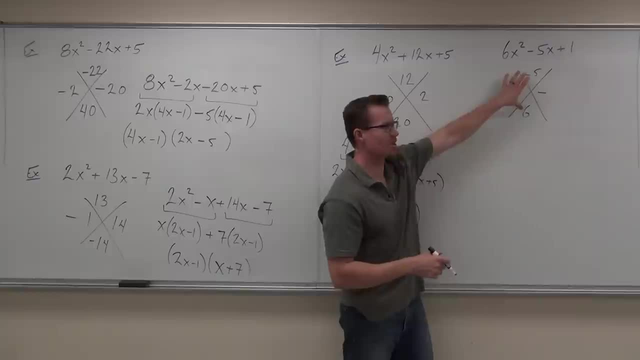 3 and 2.. So this is one of those ones with these two numbers. If people kind of get those messed up a lot, be careful And when you're sure that you're sure, double-check it again. okay, Make sure that you're sure that you're sure. 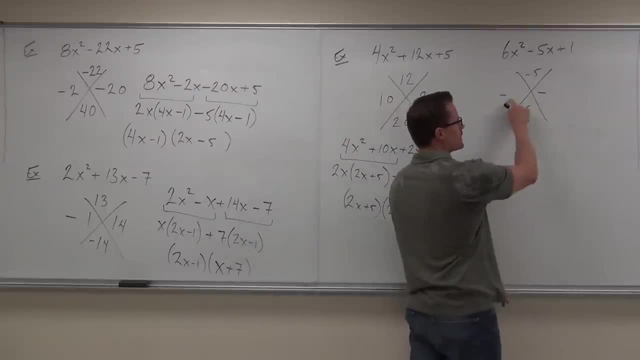 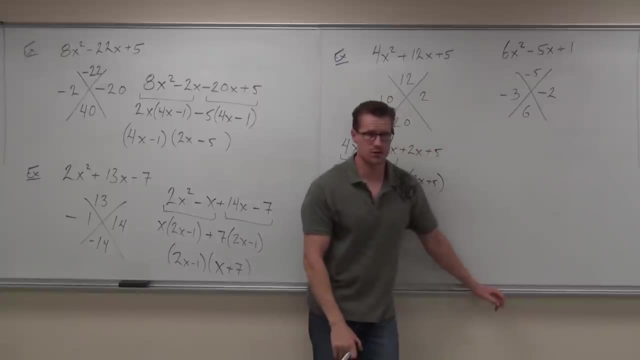 You sure? Anyway, both negative. we want a couple of numbers that add to negative 5, multiply to positive 6.. The only ones that are going to do it are negative 3 and negative 2.. Double-check it, triple-check it. I don't care, but make sure. 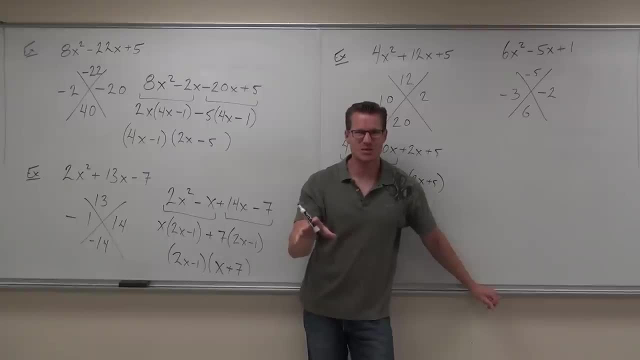 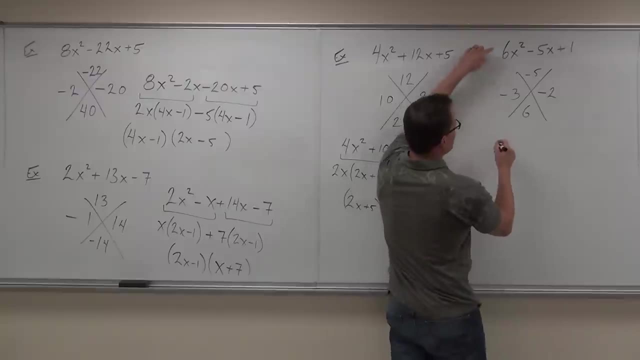 that that is correct. Did you guys get those ones? It's easy to do the 6 and 1 sort of thing or the 5 and 1 a lot, because you want to make it work like that, but be careful After that. well, we don't have a 1 there. 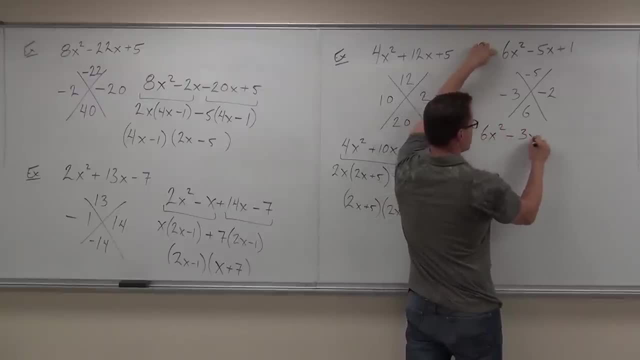 so this is just allowing us to separate our middle term, so that grouping will work. And if we do that, it doesn't matter the order. it's going to work either way. We'll group it 3x here. we get 2x minus 1.. 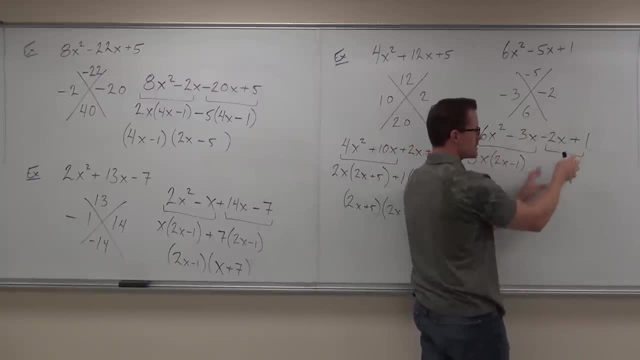 Here, check this out. I wanted to get this one 2x Here. check this out. Here, check this out. Well, next up, we've got this one there Again, there are four, 8 and 7.. 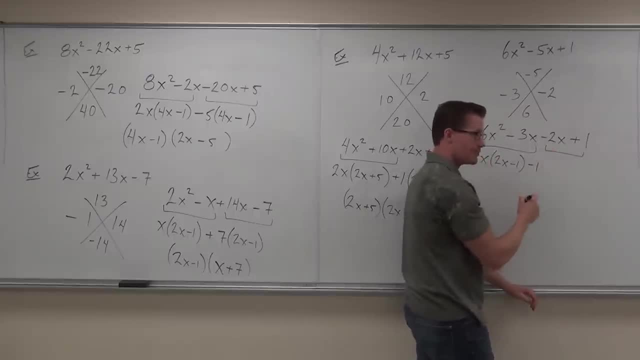 So these numbers are going to be yours. I channeled them to you on purpose this particular way. What goes into the 2x and 1?? One does, but this says it's got to be negative. so you're forcing it to factor out a negative 1.. 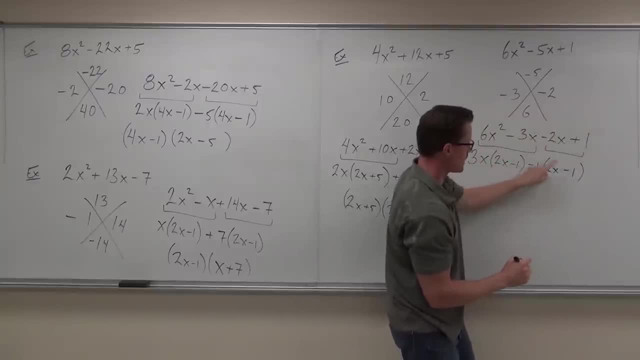 What does factoring a negative do to these two terms? So this will be a positive 2x, this will be a minus 1,. No, it's right. These have to be the same. If they're not the same, you've made a mistake. 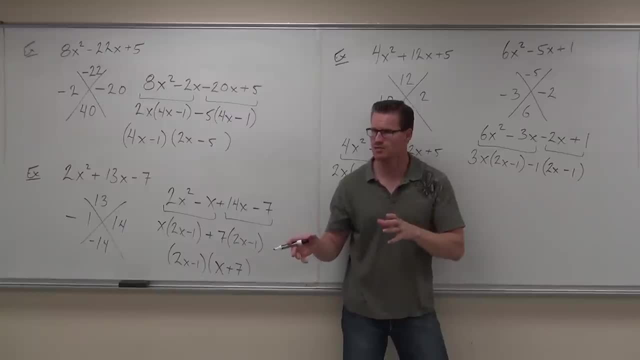 And most of the time it's just a sign error. It's just a negative where it should be a positive, or vice versa. So if this works, you have to have these the same. If they're not, you've made a little mistake. 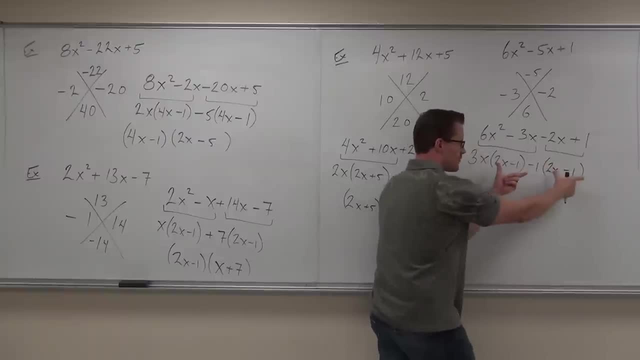 Go back and fix it. So since we have two large terms, same factor here, we're going to divide that out 2x minus 1.. We'll put the remaining factors in a new parentheses factor. It always creates parentheses. We get 3x minus 1, and we're good to go. 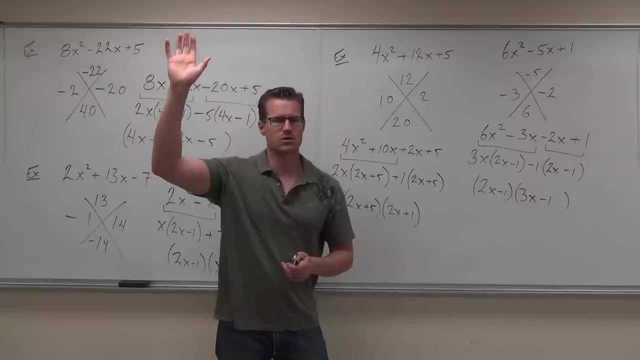 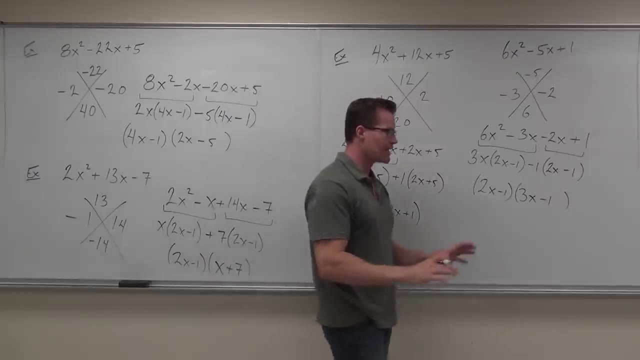 Now a lot of students who have had this class before at high school or somewhere else, and it's been a while. a lot of students really, really, really want to try and solve this right now. They want to go. oh, let's set this equal to 0. 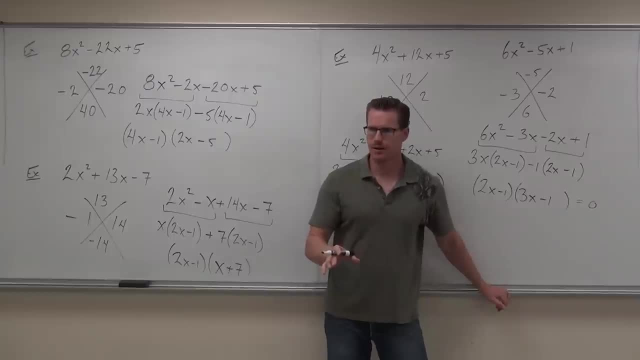 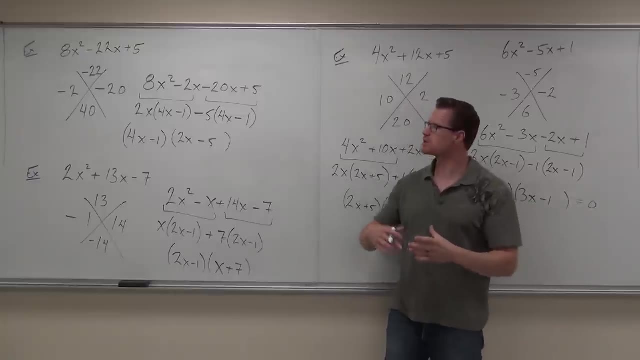 and set each factor equal to 0 and solve it. This is not what we're doing. If I haven't given you an equation, don't introduce an equation. It's not an equation right now, It's an expression We're just factoring. 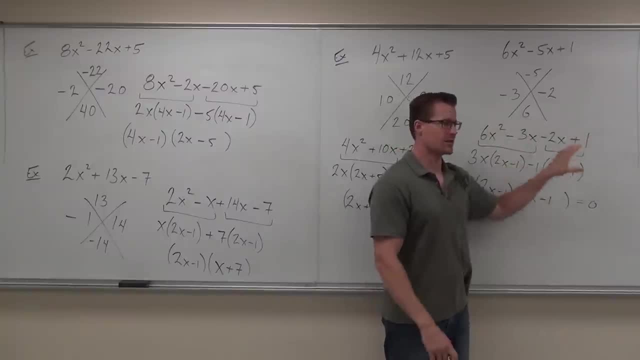 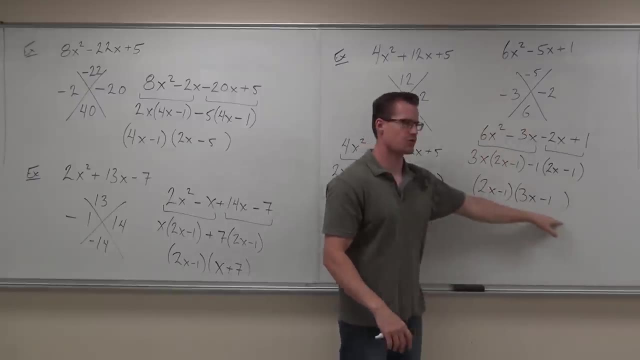 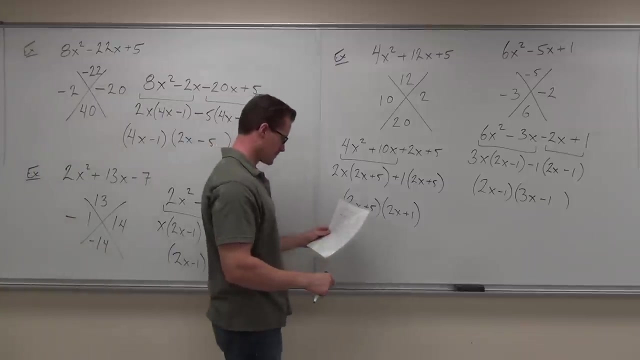 Does that make sense? We will get to the point We're actually solving, but it's not now. So your answer here is: if I ask you to factor it, here's your factorization. That's it. Tell you what? let's do two more. 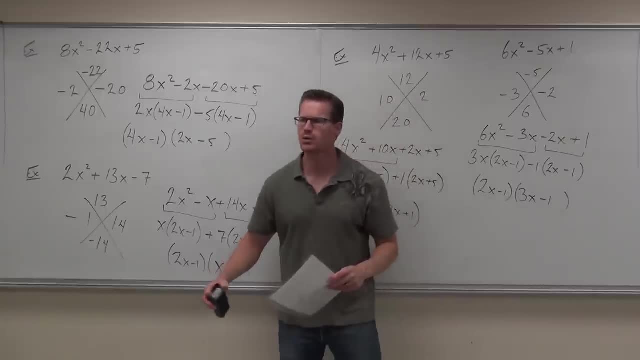 Let's just practice real well with two more. to make sure everyone's good. I'm going to walk around the room. I'm going to make sure that you guys have it okay. Treat this like a mini test. See if you can do it without. 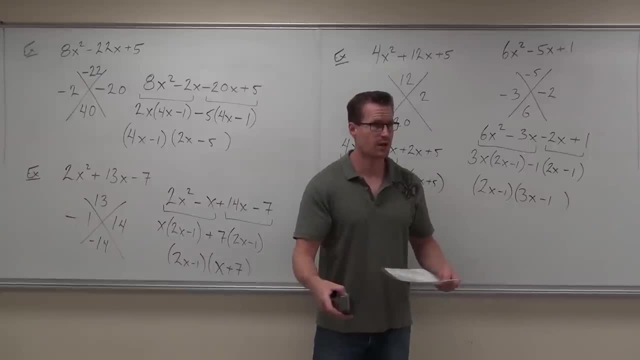 Look at your notes. I think I've given you enough opportunity to really go back and forth, right? So let's see if you can do it. If not, okay, look at your notes. Let's see if you can do these two problems without it. 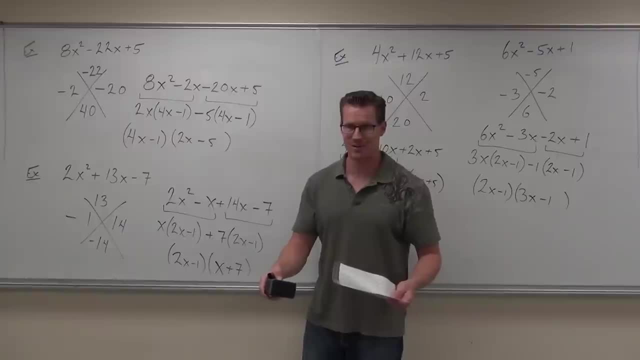 And if you can, you know that, you know it. Are you with me? These are going to be a little challenging. Well, one of them is a little challenging because the numbers are bigger. See if you can do it. You may, of course, use a calculator. 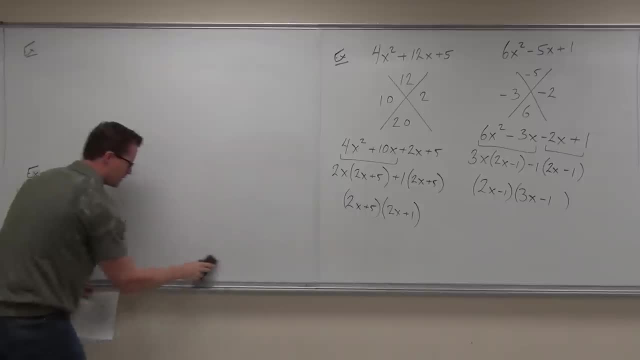 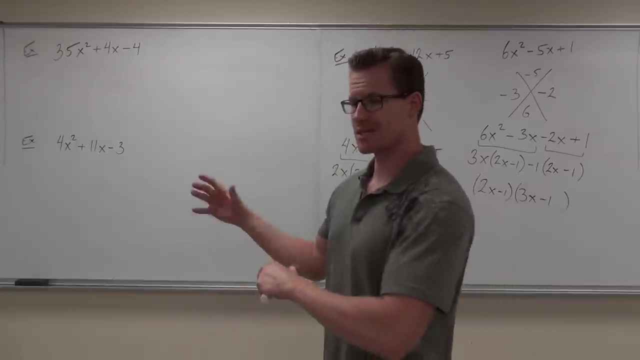 So if you struggle with finding the factors in your head, no worries, Use your calculator, That's okay. So these are the last two basic ones that we're going to do, And then, just like last section, I'm going to give you some special cases where you might see this. 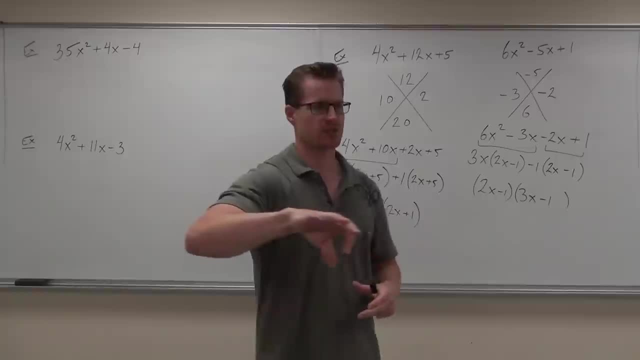 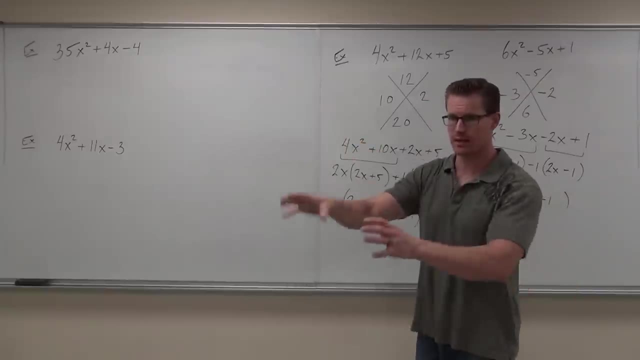 where you might see something where it looks like it doesn't originally work, but then we can use this process for it So that you don't get intimidated by them later on. okay, So right now do the best you can on factoring those blindly, without your notes. 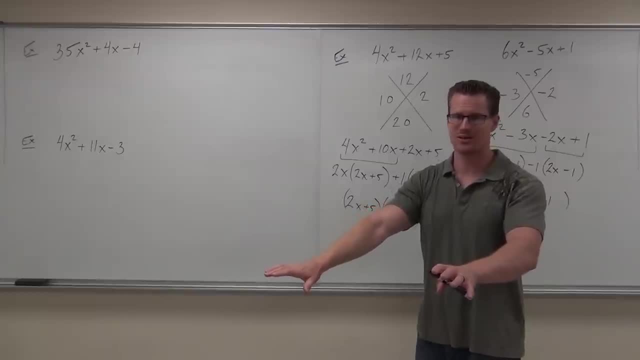 Not blindly like you're not looking at it. okay, That would be really cool, but you're going to have to look at your paper. So factor as best you can without looking at your notes And if you get stuck, okay, then use it. 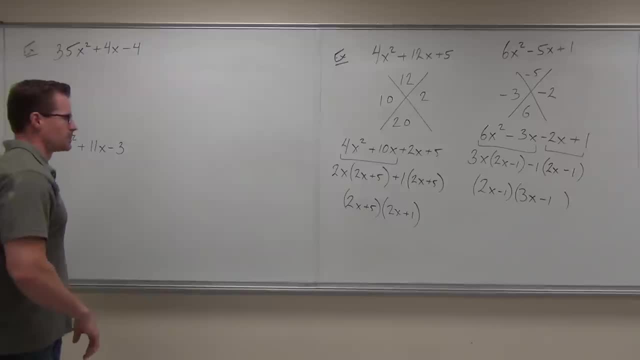 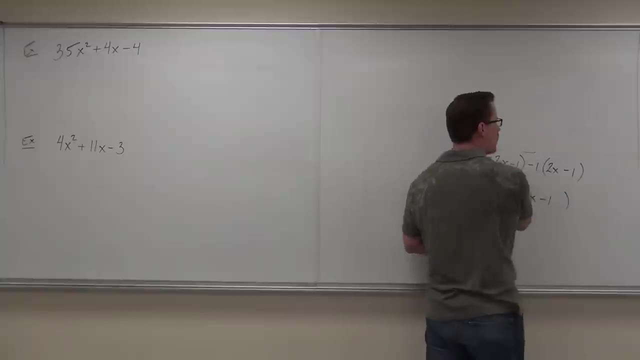 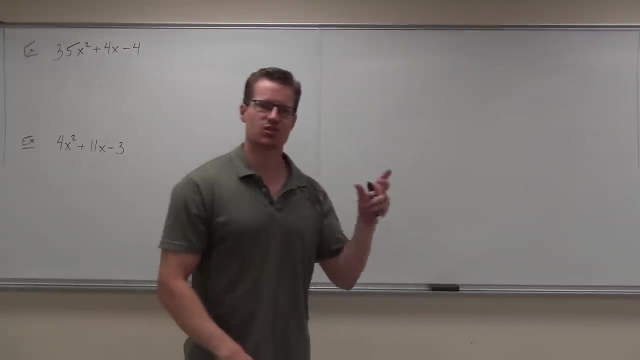 But try to do it without it. Also, I want you to think through the process, Think through all the steps, All the steps I've given you. are they in order? is the first term positive? is there a GCF? how many terms do you have if it's an extra step, diamond problem, or if it's a shortcut? 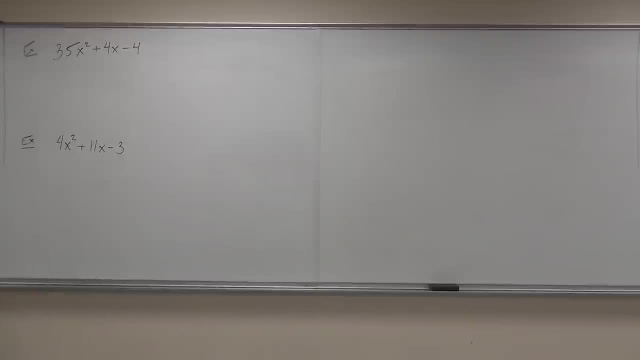 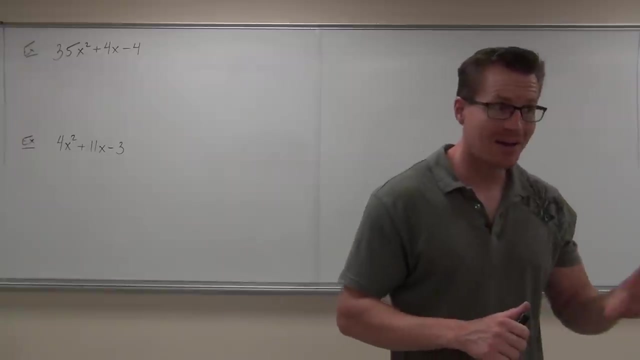 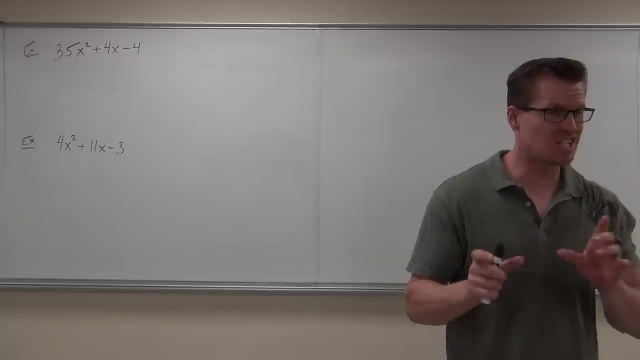 Think through that stuff every time. I know that negative 140 is a big number, I get it, but think about what the signs have to be there. Recognize they have to be different signs, do you see it? That means the difference between: there has to be four. 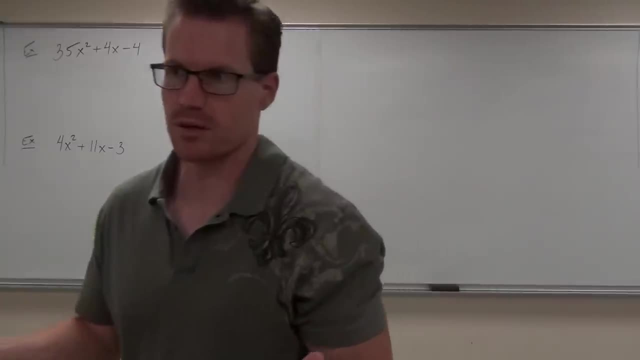 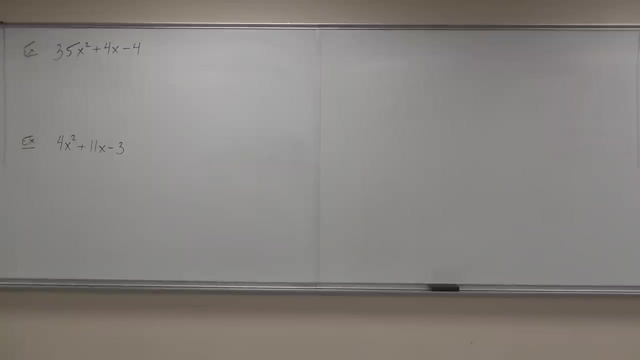 Think about two numbers where the difference is four that multiply to 140,. okay, And then you'll get it. Okay, I'll tell you what. I'm seeing a lot of people stuck on the first one right now. So what I'm going to do is I'm going to give you the diamond problem set up for that. 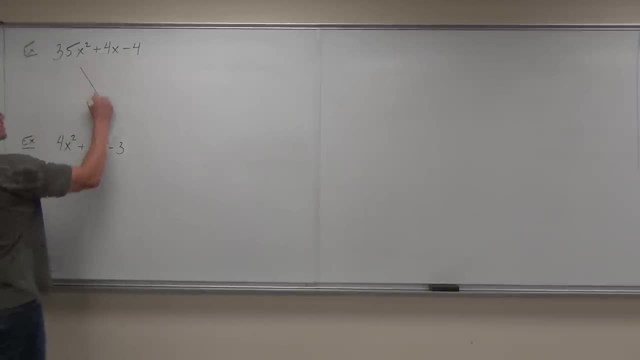 I'm hoping that you've all made it down to. I know that you, because of some of us who work. I know you got this and I know you got this. okay, Yeah, you can get stuck on these ones if you don't think through it. 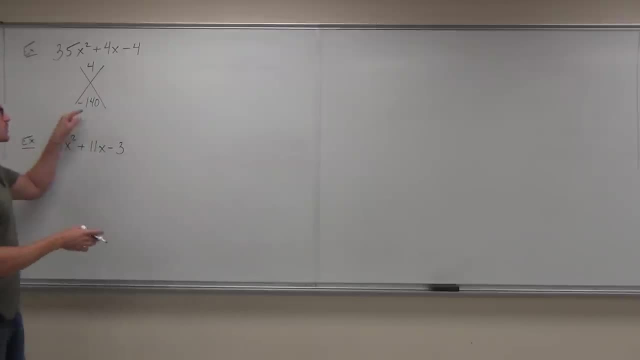 Listen, you've got to really think about this. If you're multiplying to a negative, one of these things is negative and one of these things is positive. Do you understand that concept? They're not both negative, because that would be a positive. 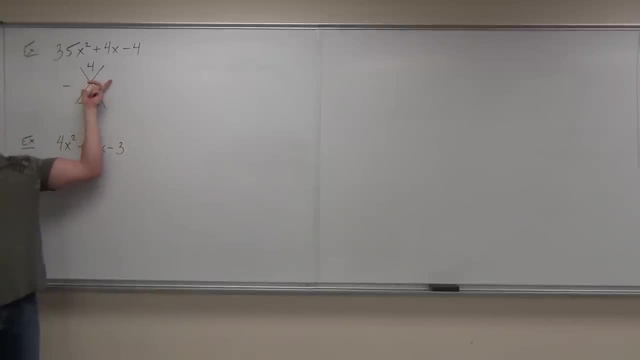 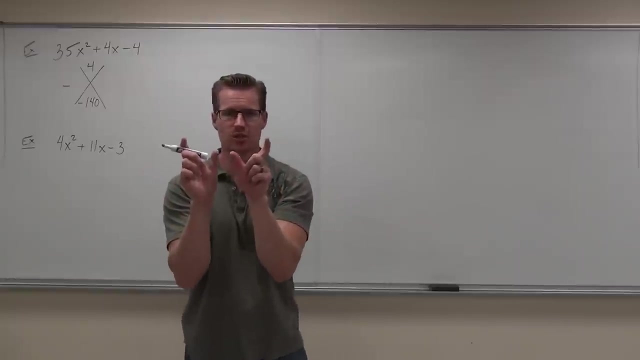 Negative times. negative is positive. Now, if you have different signs, think about how adding works with different signs. If you add with different signs, you're really just subtracting. so the difference between these two numbers you're subtracting. The difference between these two numbers has to be four. 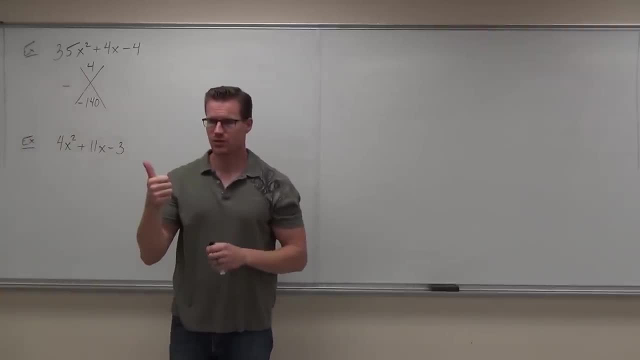 What that means is that one number is only going to be four units away from another one. Well, I'm thinking of two numbers which multiply 140. that are four spots away on the number line, The only thing that's going to work there. well, there's a lot of factors for 140,. 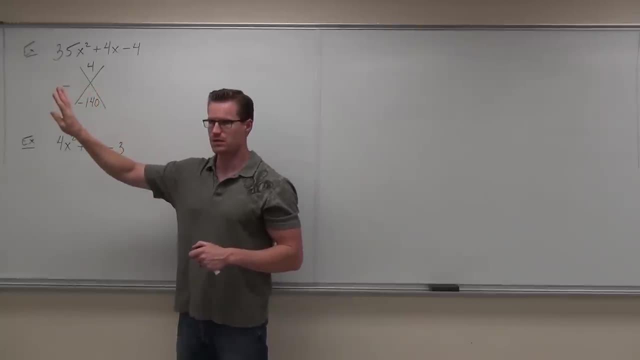 but the ones that I know that are only four units apart are 10 and 14.. Do you see what I'm talking about? Ten, four spots apart, That's. if you have different signs, use that. So for us I'm going okay: 10 and 14.. 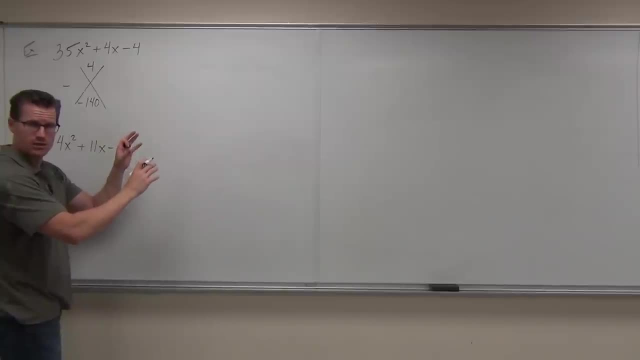 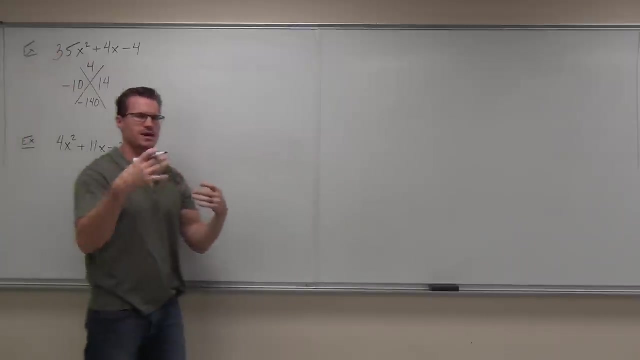 Which one's got to be the positive one, the 10 or the 14?? The 14,, because that's a positive number. It's got to be the bigger absolute value. wise has to be the positive one. That's how you'd set that up, okay. 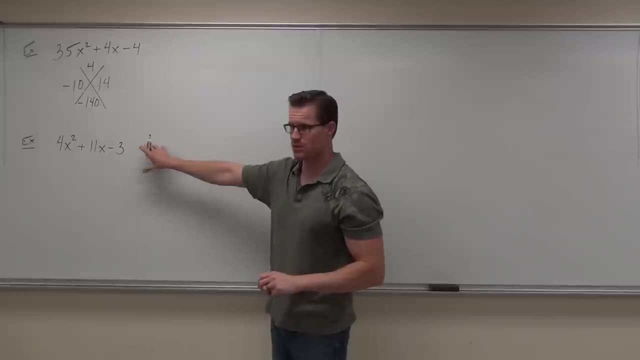 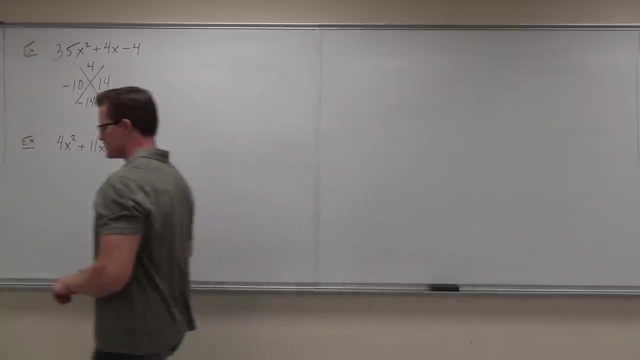 From here, I want you to finish this problem and then I want everyone to be able to do that problem. So go for it. Another Mm-hmm, Another Sure, If you feel like challenging yourself just a little bit. do you recall that we did an example very much like that last time, but we didn't have the 14?? 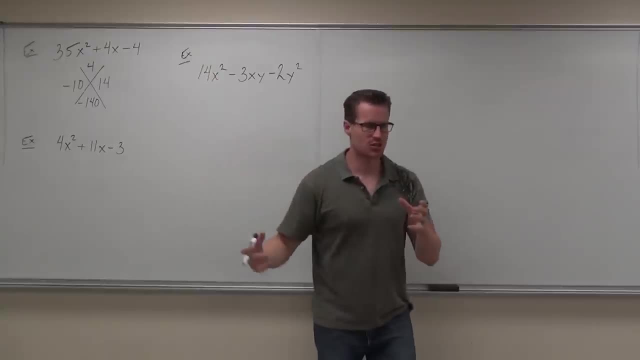 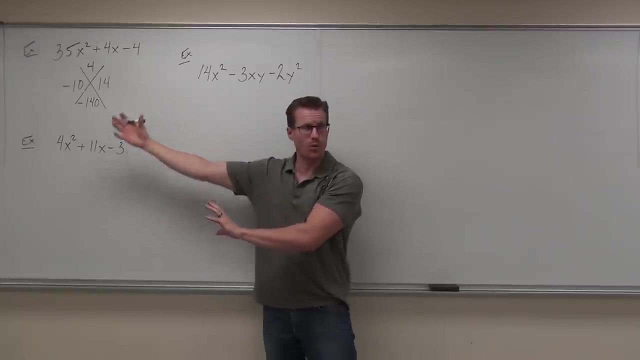 Do you remember that? It's those three terms. There's no GCF If you're done. if you're done, I'll do these two for sure first. okay, If you're done with these two. If you want something a little bit more for the next minute and a half, which is all I'm going to give you, try that one. 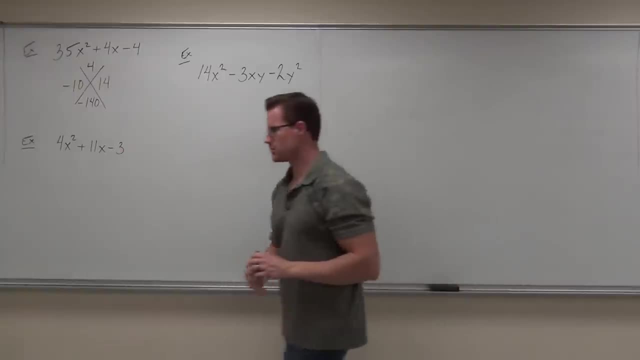 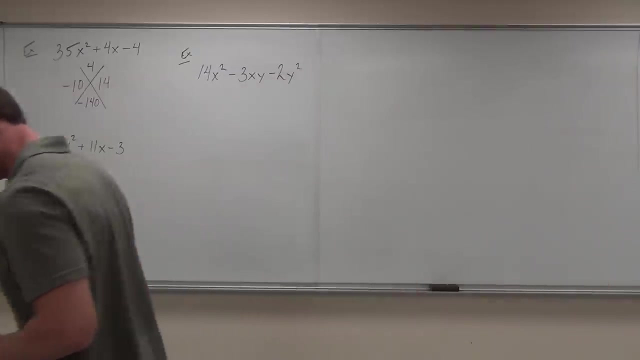 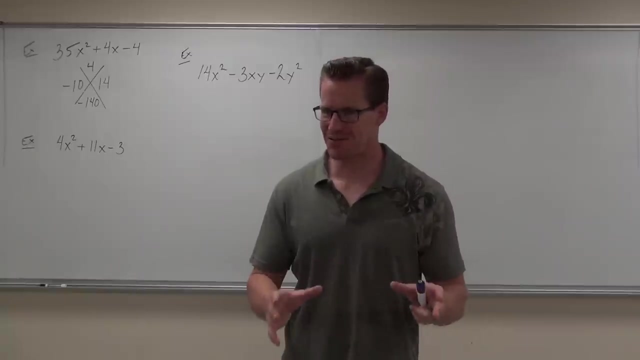 See if you can set it up. If you're done with these two, try that one. Okay, tell you what. I've given you enough time to either be finished or get really stuck. all right, So we have enough time to have done those two problems. 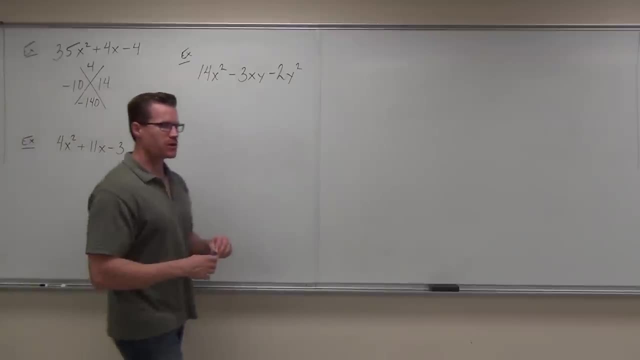 Let's go through and see how we did. okay, Remember that if you got stuck right now, if you got stuck on the, there's two ways to get stuck on this. You either get stuck on the other side or you get stuck on the other side. 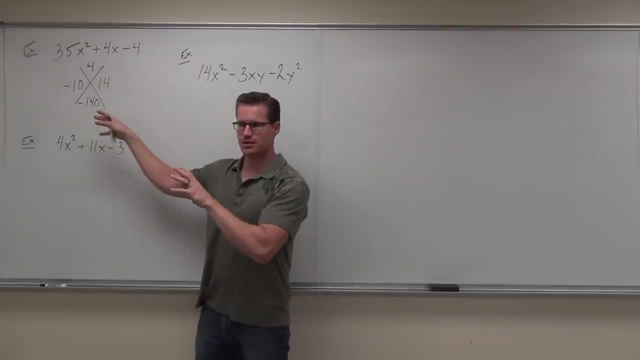 You either get stuck on finding the numbers or you get stuck on the process. What I can't afford for you to do right now is get stuck on the process. The process should be very clear at this point. Is the process clear for you? 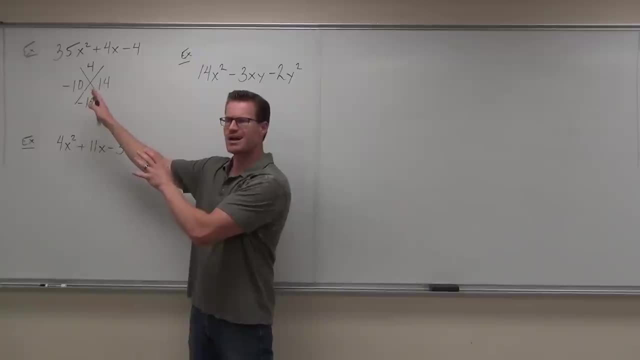 You understand what to do next. right, That's the process. If you're like man, I just can't find the numbers. that's different. What my job is to teach you is the process of doing this: how to do it every time without fail. 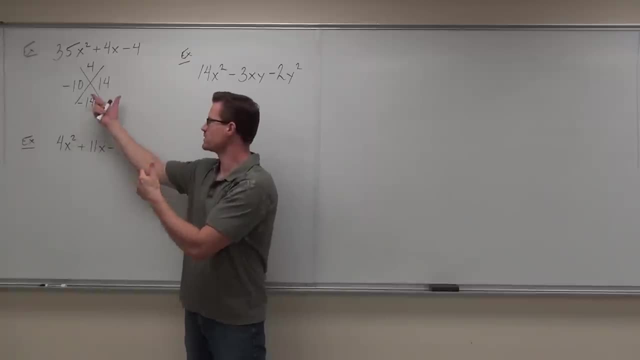 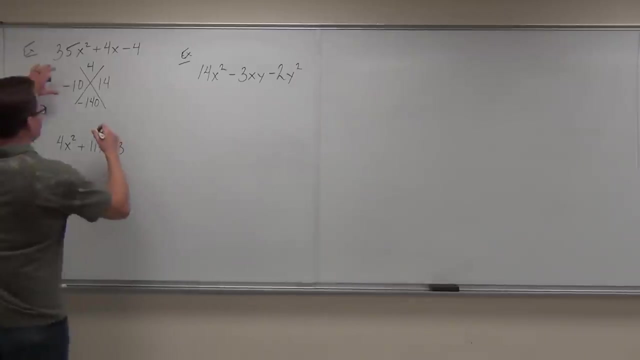 And that's what's going to happen here. If you fail to find the two numbers, that should take some work on factors And thinking through what works here. So here we go, Those two numbers. they definitely add to four. they multiply negative 140.. 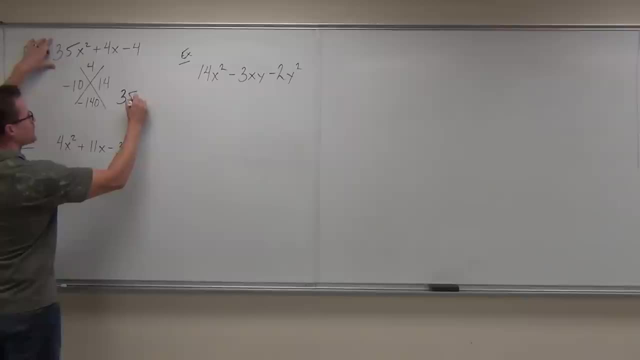 This, because that's not a one. this only allows us to split up our middle term And then to factor by grouping After we factor by grouping. if you write out the correct factor by grouping, which I know, problem is done. 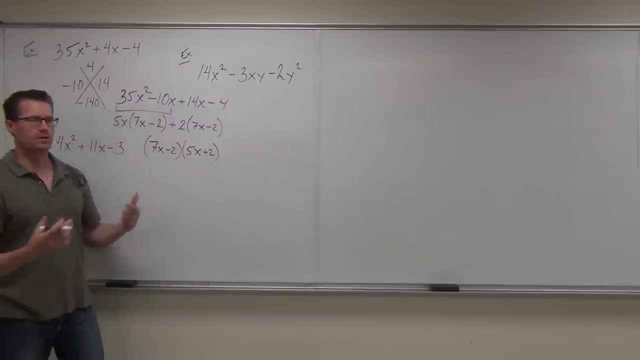 7x minus 2, 5x plus 2, those are the only factorizations. that's actually going to work here. In either order, that's fine. I want to know how many of you were able to make it there on their own. 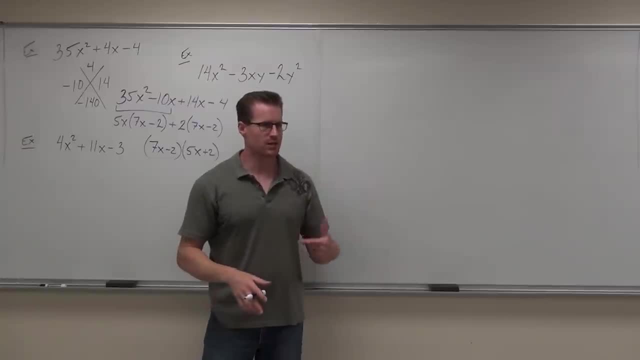 That's really good. If not, that's okay, But try it again later. okay, See if you can go through the process again. Next one Same thing. it's a diamond problem, It's 11,, it's negative 12.. 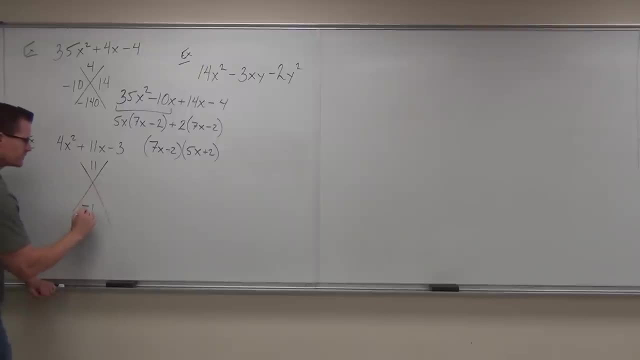 Did you guys get 11 and negative 12?? If you set that up correctly, you at least know the setup. Now find out the two numbers which add to 11 and multiply negative 12.. You've got to use some critical thinking here. 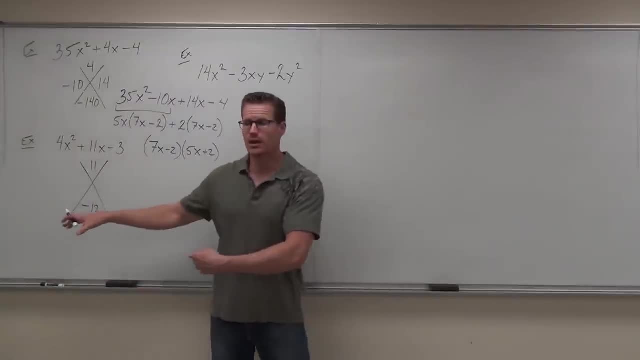 You've got to think through it. If that's a negative, one of these is positive, one of these is negative. Has to be, Because a negative times a positive gives you a negative. It's only what happens. So if you're going to do this, you're going to have to do it. 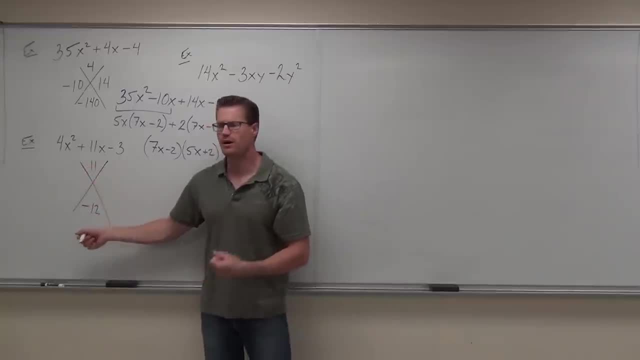 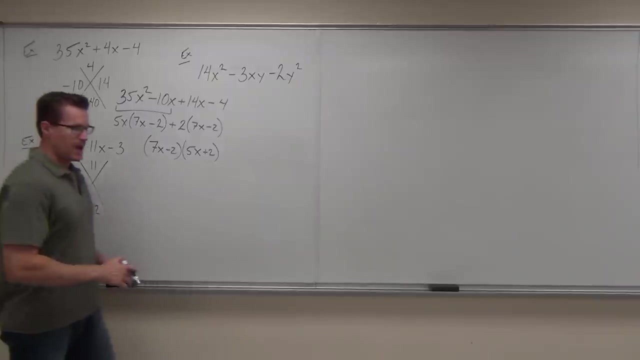 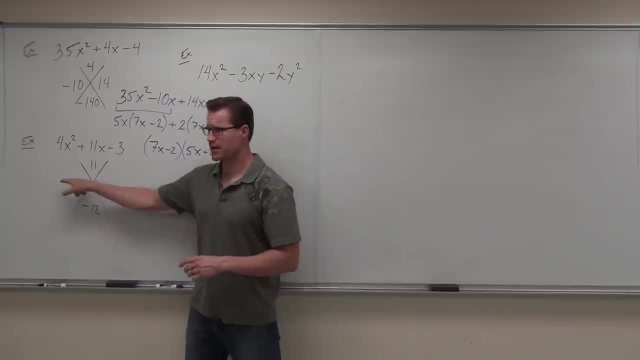 different, the two numbers will be 11 spots apart. If the signs are the same, these two numbers literally add to that one. So if the signs are different, you're kind of subtracting All right, if the signs are the same, you're kind of adding. 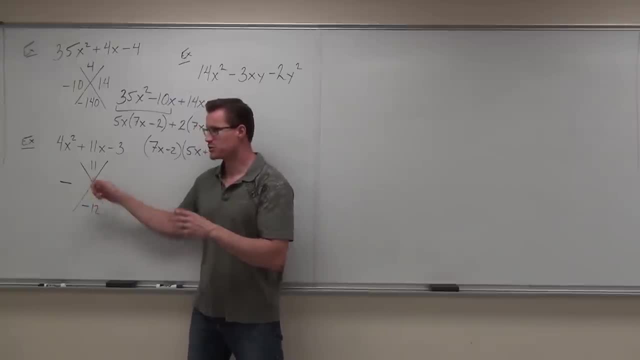 So if these signs are different, the difference between them in terms of absolute value is 11 spots apart. What two factors multiply to 12 and are 11 spots apart, 1 and 12.. That's it, It's the only thing that's 11 spots apart that multiply to 12.. 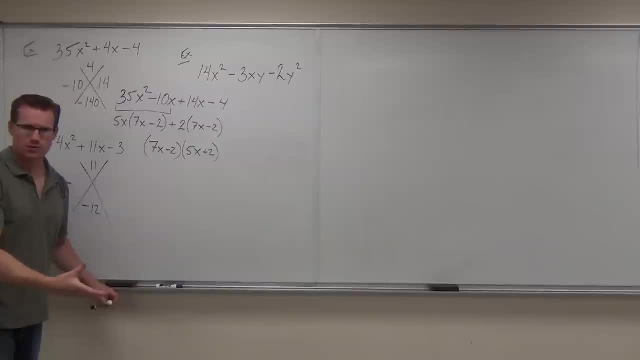 And that's how, with these larger numbers, you can think through it, if it doesn't just come into your head. So anyway, which one's negative? the 1 or the 12? 1 and 1.. So again, because our a is 4,, not 1,. 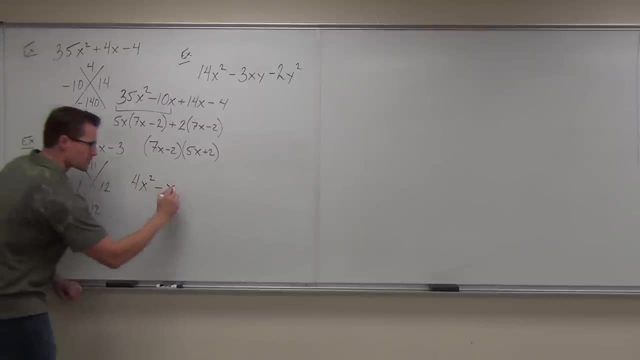 this allows us just to separate our middle term And then to factor by grouping And then check our work. Ah, it's the same, I've got to be good to go 4x minus 1.. Put your extra factors here. 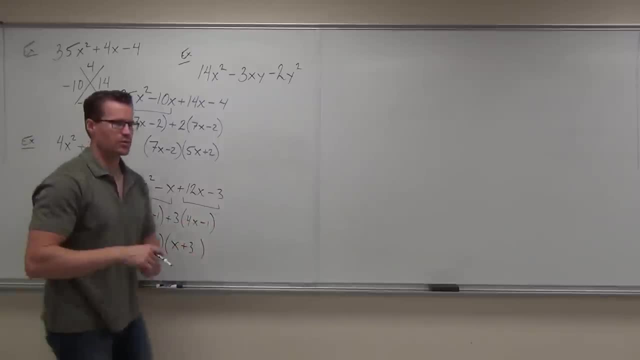 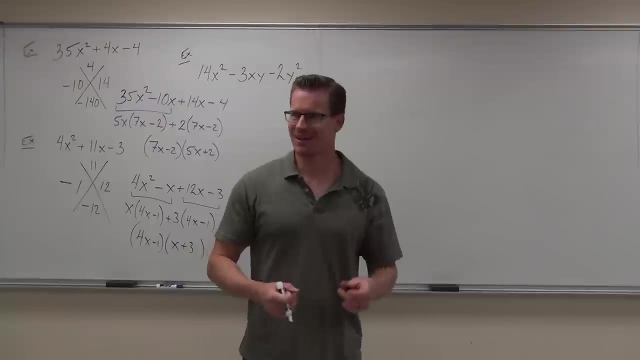 After you've factored this out inside of a new parenthesis, And this should all be kind of making a lot of sense at this point, Be kind of old at this point. Is it getting that way? Okay, Is it? Okay? I get it. 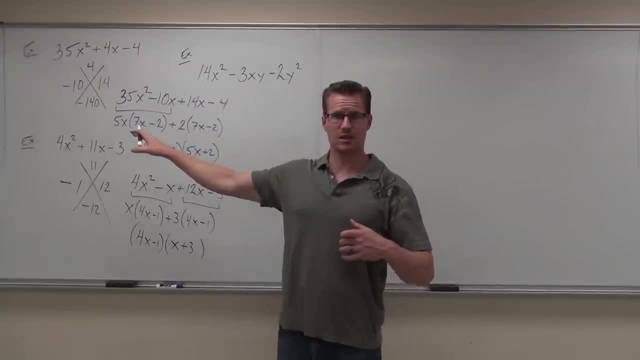 When I'm doing it. can you follow it? Okay, Are you starting to get to be able to do it on your own Pretty easily? That's good. That's where we need to be okay. Okay, Now this last one. 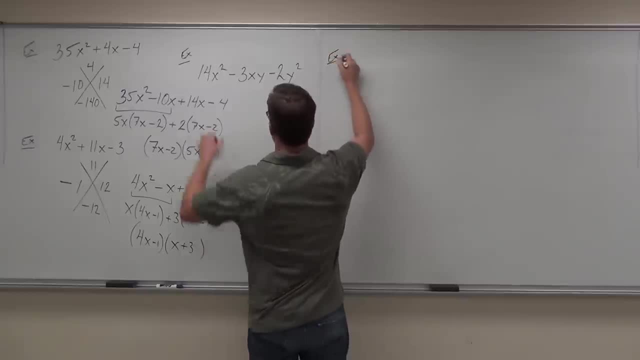 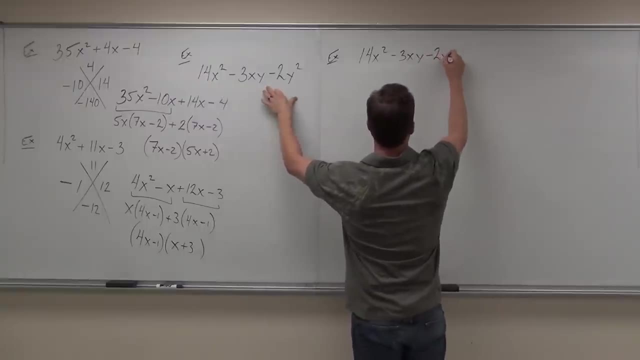 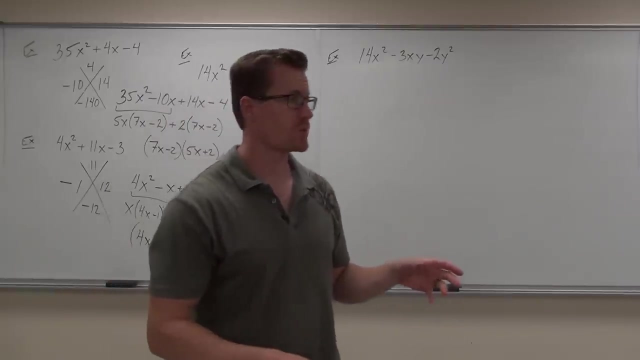 I kind of ran out of room on the right over here. I told you, if you want something a little challenging to do, that one it's not super bad, because it's very similar to something we did in section 6.2.. Let's think through it. 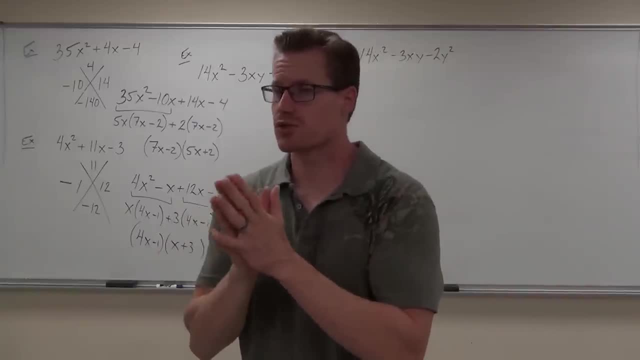 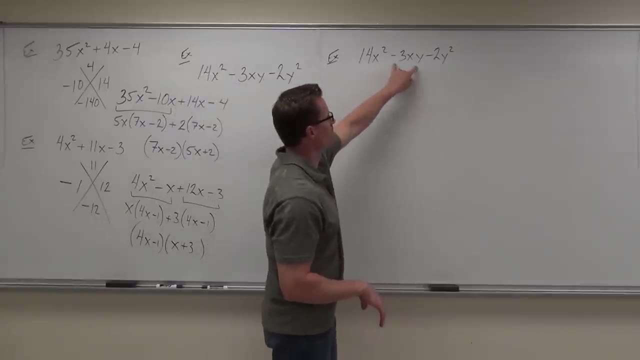 Let's see if the process still works. What would you check first? Order, Yeah, order And order's a little weird. What I told you about this type of order is: put the x squared first, put the x and then have no x. That's fine. 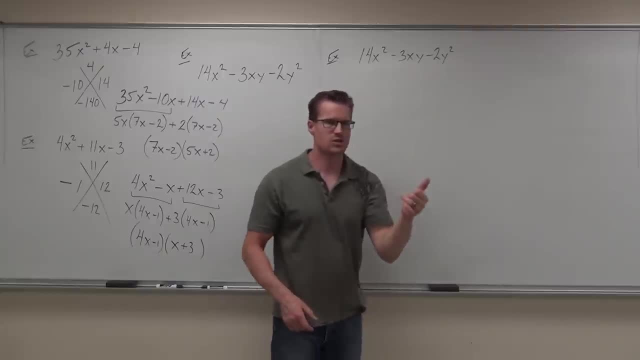 That's at least in some sort of an order. Next thing to check for: is the first term positive, Is it? It's great We want that. Next thing we check for does it have a GCF? Never fail to check, though. 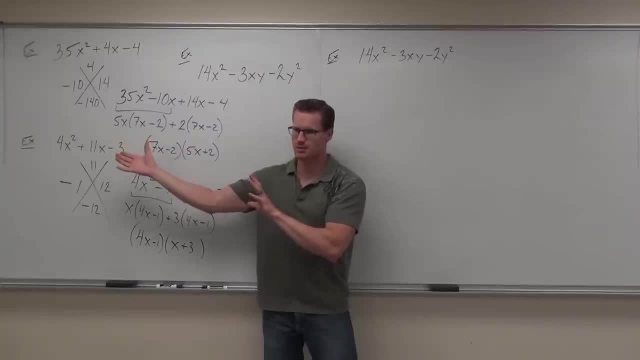 Sometimes it won't- Most of the times for us here it doesn't, But sometimes it will- If it doesn't have a GCF besides 1, I guess I misspeak when I say it doesn't have a GCF. The answer's always yes. 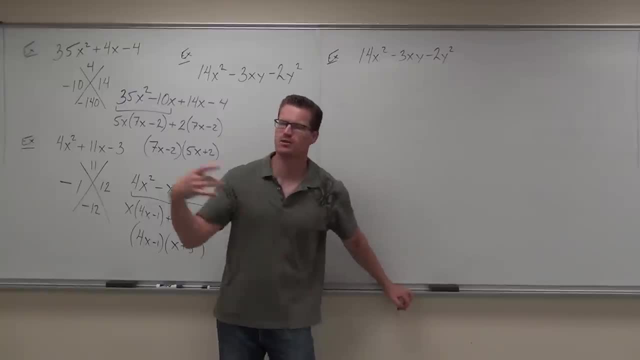 Does it have a GCF that's not 1? No, So we can't factor anything out of it. That wouldn't make sense. So then we start counting the number of terms. How many terms does it have? Three, If it has three terms, a diamond problem. 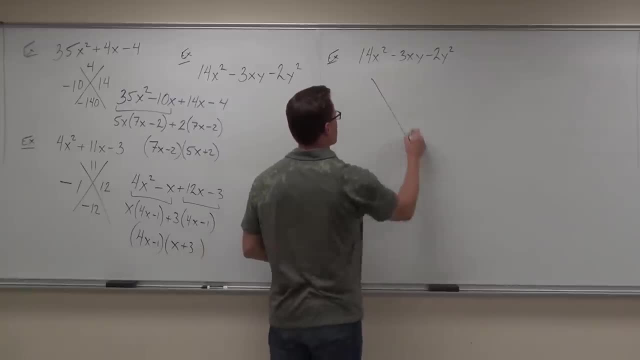 will still work for us. I showed you this last time. What number goes, here Negative, And here Negative, Negative. Do you understand that one of these will be negative? I'm going to put it here, just to reiterate. one final thing. 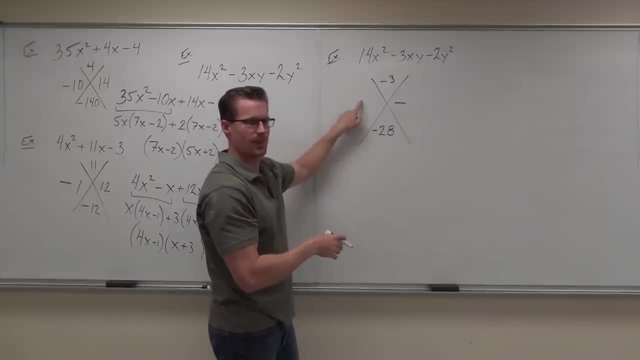 One of these numbers will be negative and one of these numbers will be positive. Did you guys get that Different signs? Hey, how about that? So that means that the difference between these two numbers has to be three. These factors find two factors that multiply to 28.. 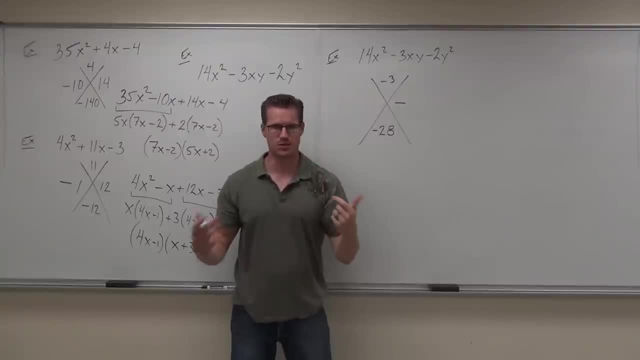 Or the difference between them is only three, And you'll find it's four and seven. It's only two factors that are separated by three. Since the signs are different, you can use that, And the bigger one has to be negative. Let's double check. 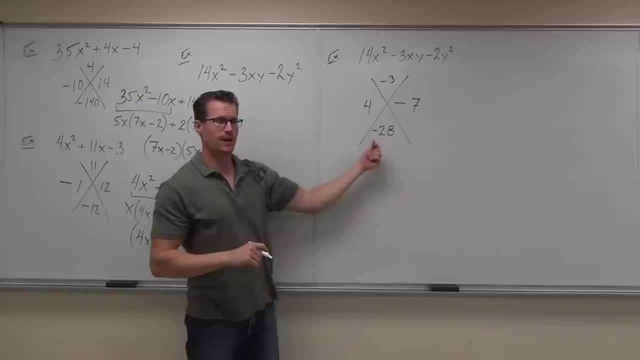 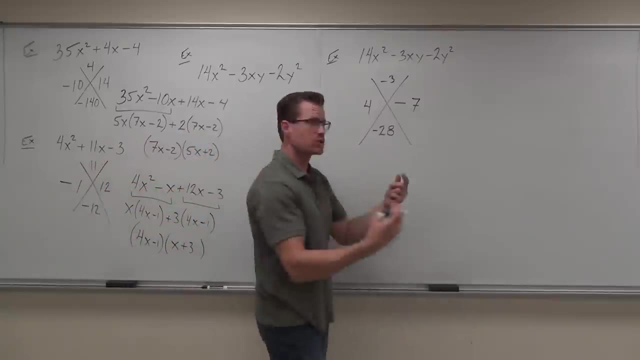 Does that add to negative three? Yes, And does it multiply to negative 28?? And should I go do my shortcut or should I separate my middle term? Separate Absolutely. When you're doing this, use the same exact structure as you've done. 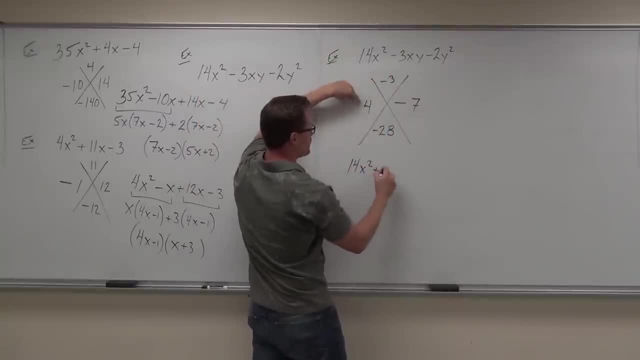 We just have the 14x, The 14x squared, we add the four. just keep this xy. Don't separate those, don't separate these variables. okay, It's 4xy minus 7xy and then minus 2y squared. 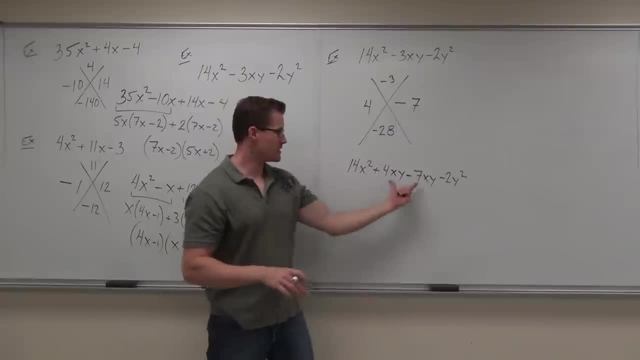 If you do that, vectoring by grouping works really, really well. Can you verify that? this really is the same as that? Yes, Okay, And then we continue, Because we have a few more variables. you're going to factor a little bit more stuff, but it's the idea is the same. 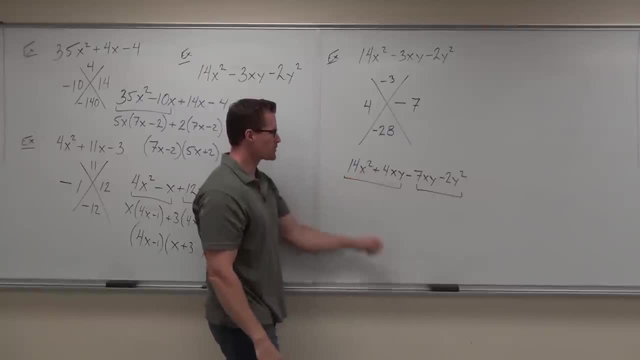 We've done so much of this, it should hopefully be making sense. Yes, What factors out of these first two terms? 2x, 2x, And we get 7x plus 1.. A little bit off. 2y. 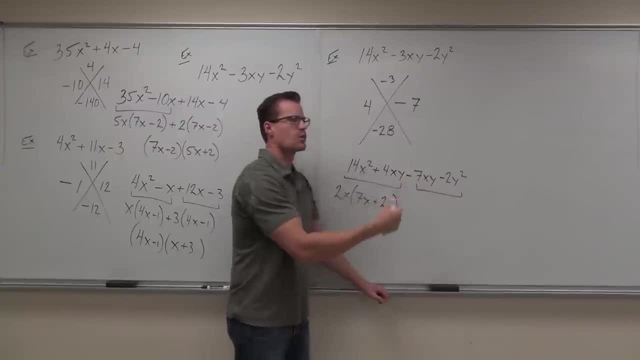 2y. Okay Here. I did this on purpose to show you one more time that if that's a minus you have to factor a negative. I want to kind of hammer that home. That way I don't give you all the easy stuff. 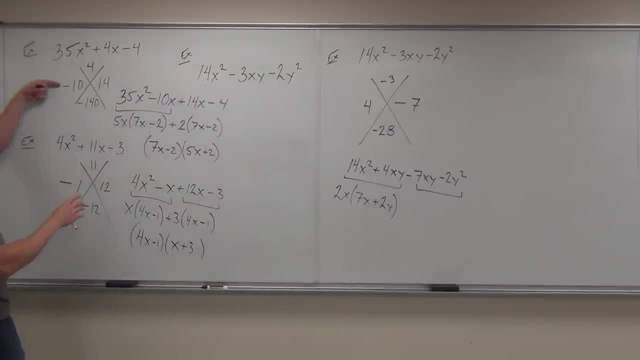 You'll find that how I set these up normally is I put the negative number first, That way you don't have to factor out the negative and that you kind of avoid that. But I want to make sure you, I want you to be able to see it. 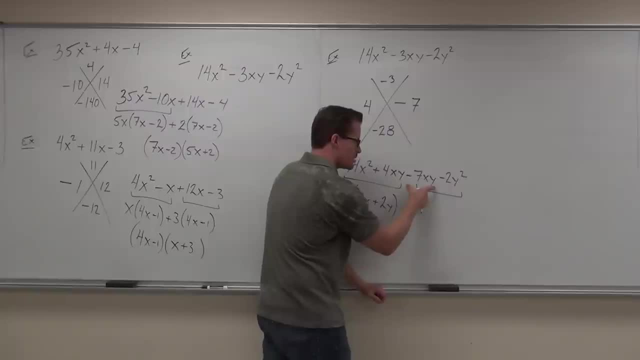 What factors out of these two terms please? Y Y, Negative y. I like how you said negative y, because that forces you to factor the negative y. There's 7x and Plus 2y, Plus 2y. 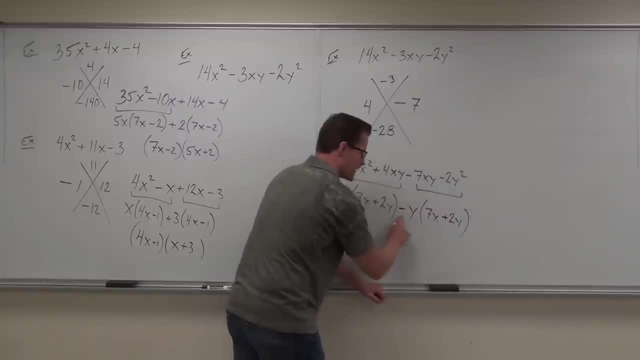 Why does that sign change? You can pull it up. You factor a negative Factor, a negative divide by a negative. it changes the sign. If we keep on going, we pull out our common factor, We create parentheses because we're factoring. 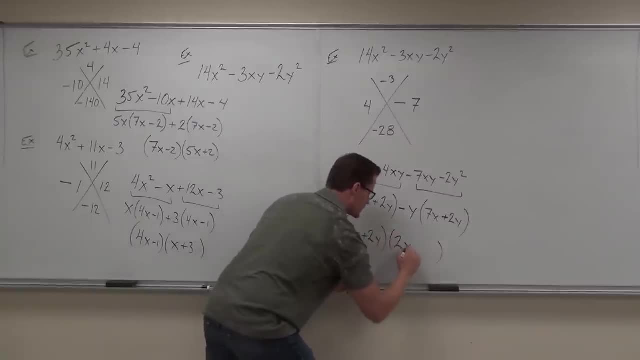 We put our extra factors that we did not factor out. We put them together and we're done. Feel okay with it. Mm-hmm, All right, So let's continue a little bit. We're going to just do some special cases. give you the overall what you can do with this. 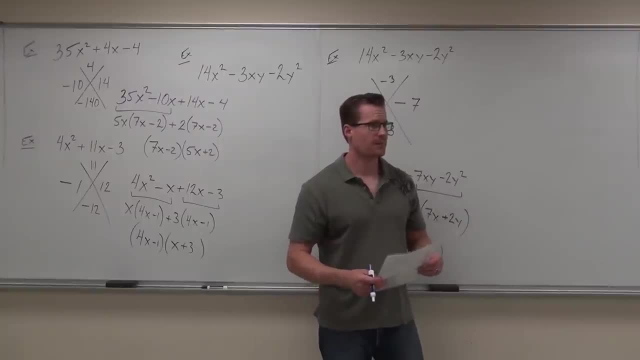 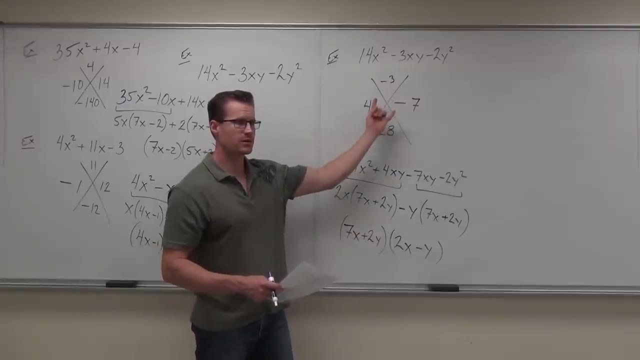 and how to go about losing these problems. Question: There's actually two ways to do that. Did you get the same answer? Yeah, Okay. Were you never switched? Yes, Okay, Yep, I used the 7 and the 14. on the group B. 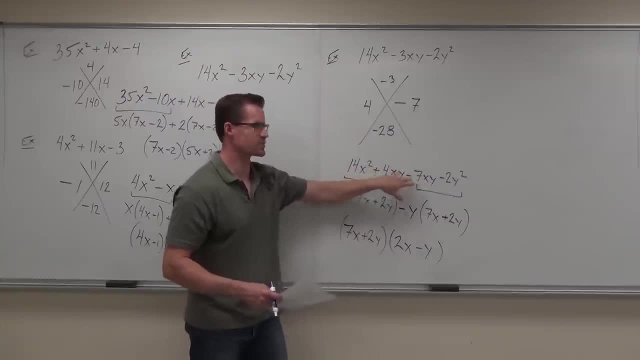 You used 7 and 4.. Oh, I'm sorry, You have this here and this here. I used 14 and 7.. So you have this here and you have this. These are flip-flopped, That's fine. 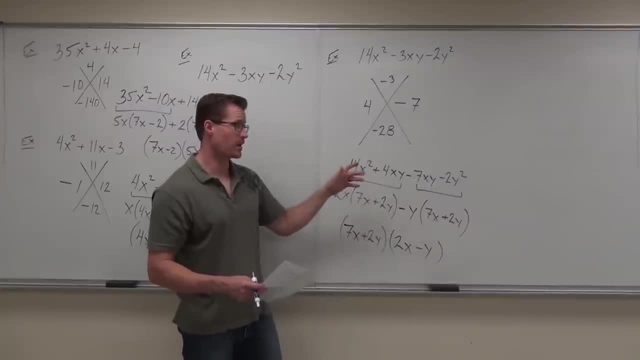 It doesn't matter, In fact, how I would normally do. the problem is that way because I like my. if there's different signs, I like my negatives first. That way I don't have to factor a negative here. So I just show you this every once in a while to make sure you see that. 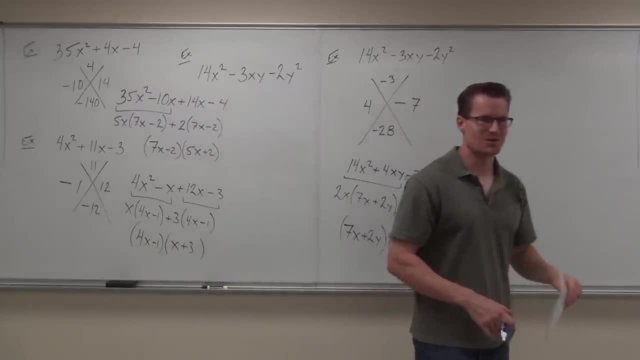 if that's the case, I'm going to get a negative. If that's a minus, it forces you to factor a negative. Just keep you on your toes. I'll make sure you're here with it, Ready, Mm-hmm. 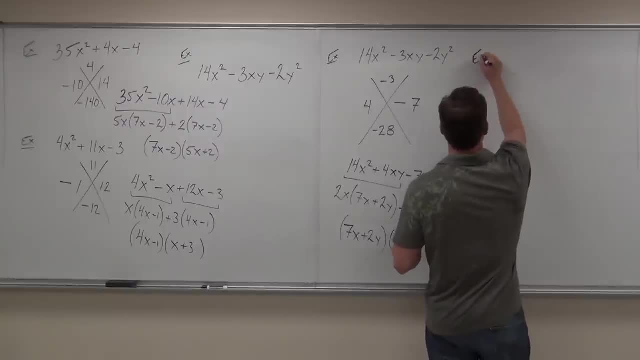 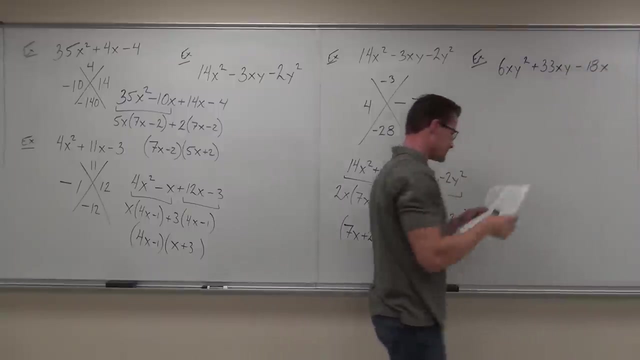 Okay, Okay. we haven't done this in a while, so we're going to do this. We're going to start with the left side and go row by row on our steps here. I want you all to really be with me on this. 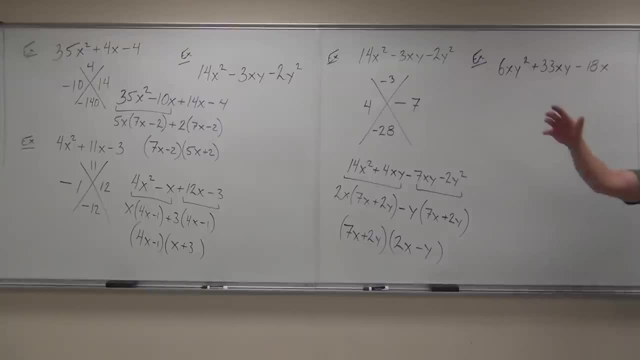 So, left side you guys. you're my left, by the way, and you're my right, because I get confused. So first row over here, left side row. What's the first thing? you're checking for Far left. You're not the far left row. 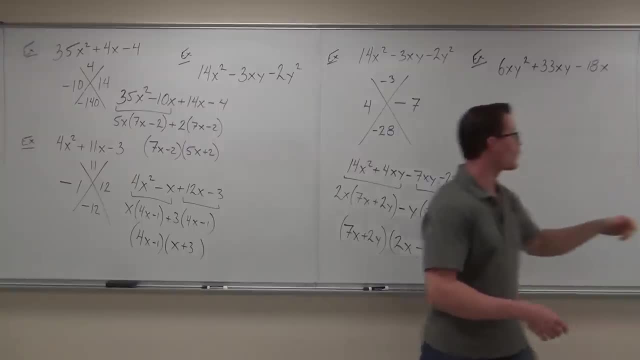 You just get. okay. so order. yes, Is it an order? Yeah, for the most part We're going xy squared and then xy and then x. Okay, so that row. The next thing you check after order is what? 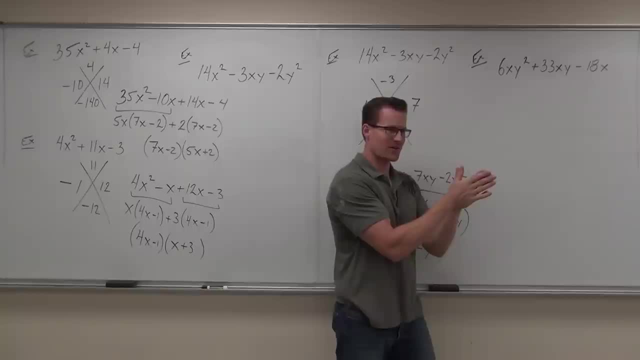 Our GCF. We are out of order, aren't we on our order here? That's okay. We do a GCF besides one. We're also checking when we're doing that, to make sure our first term is positive. Now, if you skip the checking for a GCF, this problem explodes in your face. all right, 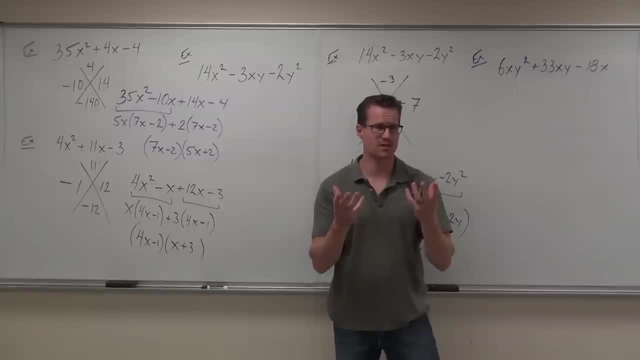 Kind of like my daughter's poop rocket this morning because she's eight days old. That's what your paper's going to look like, And you don't want that because that's nasty. So true story. I'm not going to say it on video, because it's nasty. 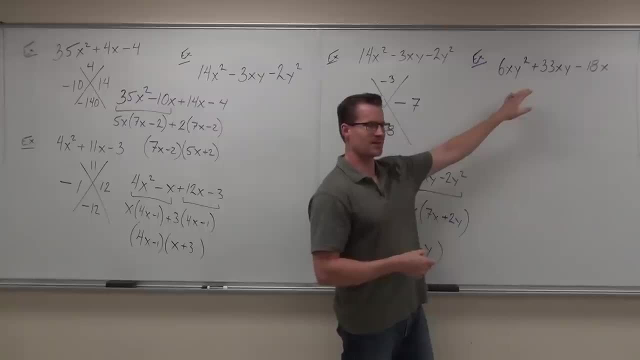 Anyway, eight-day-olds can't really control their bowels, apparently suckers. So you check for GCF. You have to factor the GCF or some of these things get really ridiculous or near impossible. okay, So this row. is there a GCF in this problem? that's not one. 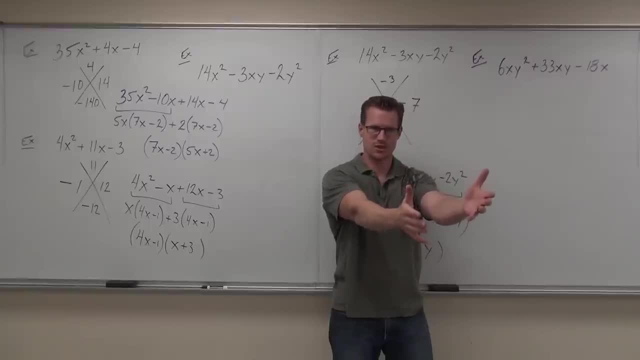 Yes, What is it? Three X. Do you see the X? Don't lose the X. This thing will not be fun. okay, You have to get a GCF. When I say that, I mean you don't make a mistake on it. 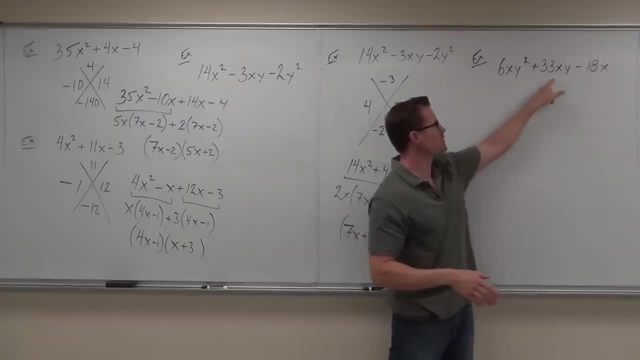 You get the three, The three's, pretty easy. Yeah, three goes into all three numbers, But X goes into all three terms as well. Three X's is a GCF. You all with me on that one. I cannot stress enough how important factoring a GCF is at the start of this. 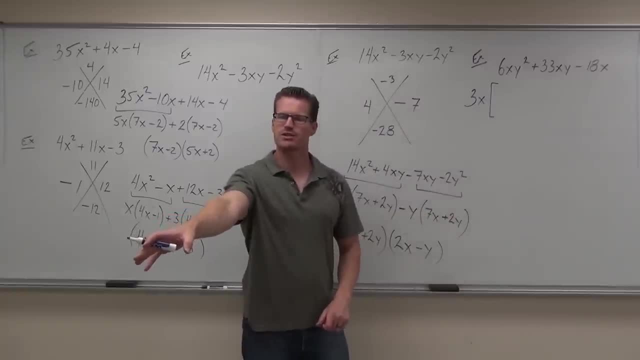 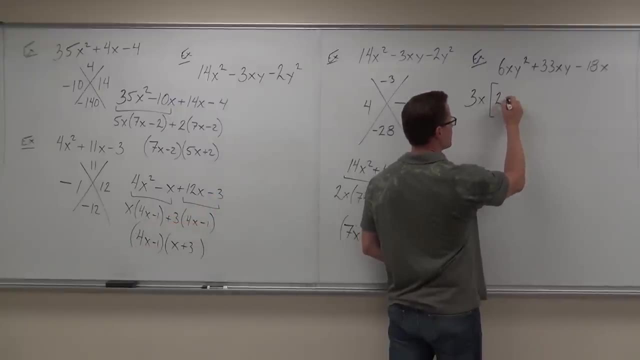 If I do factor the GCF, we'll go to this row. What are my terms? Say them nice and slow so I can hear you. okay, What's the first term? Two X, Two Y squared, Two Y Plus. 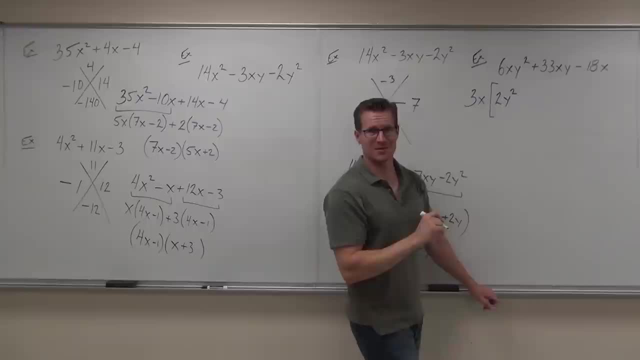 No squared Squared. Okay, very good, You can say them a little faster than that. What's the next? I know you are. Let's go to someone else. What's the next one besides two Y squared Plus 11?? 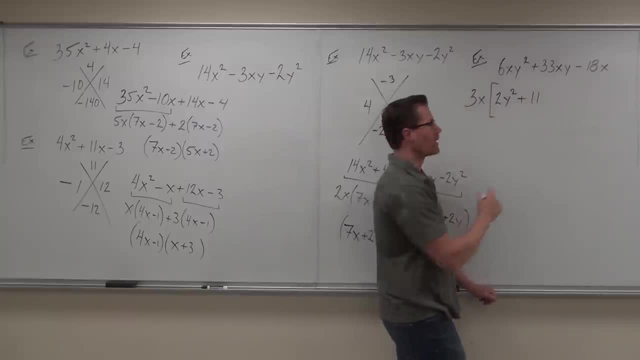 Y, Just 11?? Y minus One. Okay, one One, And then Someone else in that row. What's that? What's that at? So we got two Y squared, We got, plus 11 Y, We got- I know it's going to be minus. 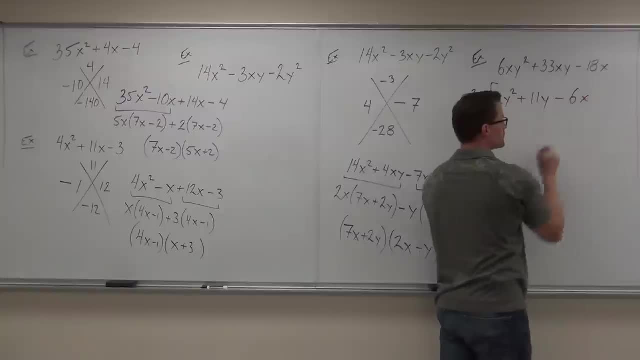 Minus what? Six X? Six X, Six X, No, no, just an X. Okay, because we're dividing the X, So no X. Can I get a double check on that to make sure that we're right? Are we right? 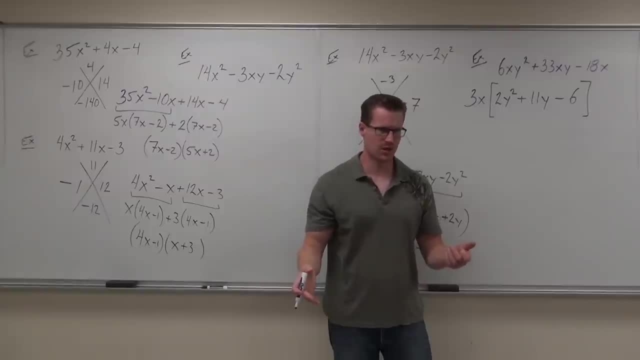 Yeah, Can you double check it? Yes, How easy would it be to double check this right now? You can distribute. That's it, So make sure that you have that right before you go any further. Okay, always double check Next row. 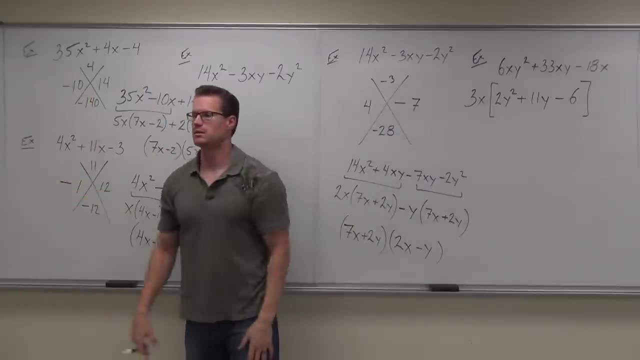 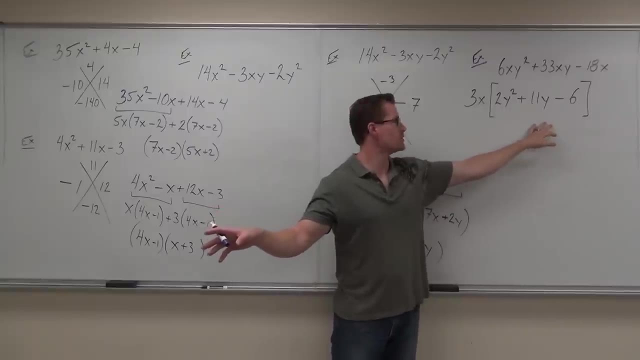 Next row, you guys. Am I done? No, No, I've just factored GCF. What is it going to take here? Diamond, Okay, now the diamond problem that you're referring to: is it going to be the shortcut one where it should go right to it? 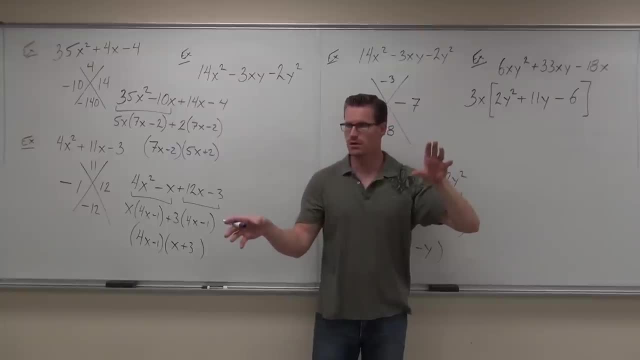 Or am I going to have to split that middle term, Split it up? And how do you know that? Because the game is not one. All I heard was- but I'm assuming that you said that's not one. So good, Yeah, that's right. 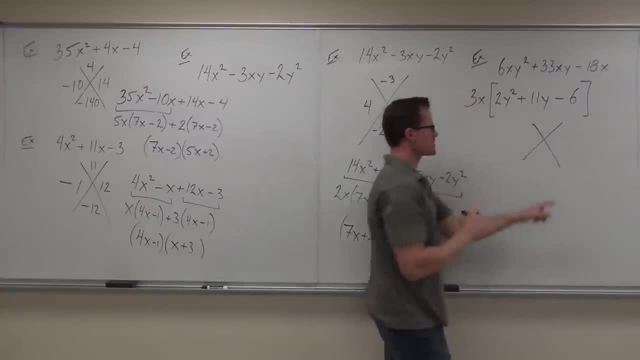 Okay, next row over. We're going to set up a diamond problem. Can you please tell me what goes up top, Up top Good And what goes here Far row? you get the fun job. you get the good stuff. 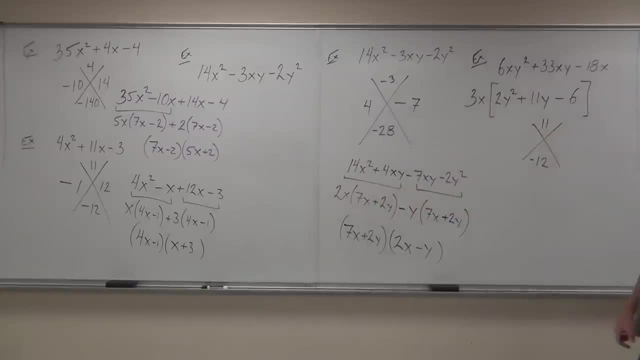 I'm looking for two numbers which add to 11 and multiply to negative 12.. Negative 1 and 12.. Yeah, hopefully you saw it up here. on the same numbers: Yeah, negative 1 and 12.. Go back to this row. you guys didn't even get a chance yet. 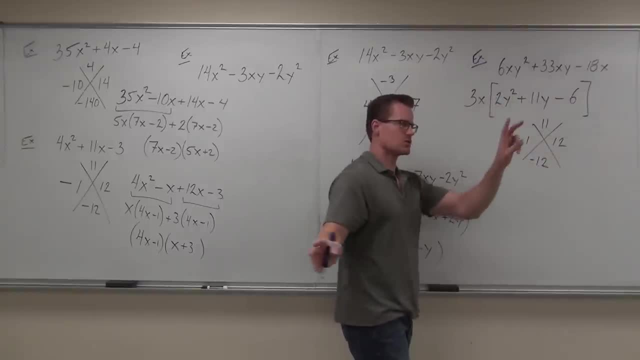 because everyone was speaking for you. I asked them the same question. you're going to get two questions. Firstly, can I go directly to x, X minus 1 and x- I'm sorry, y minus 1 and y plus 12.. 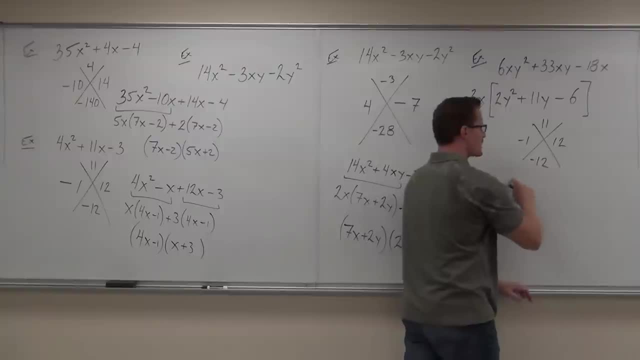 Is that a good idea? Okay, tell me exactly what I need to write. You need to write 3x with parentheses, Good, And then 2y squared minus 1y, excuse me- plus 12y and then minus 6.. 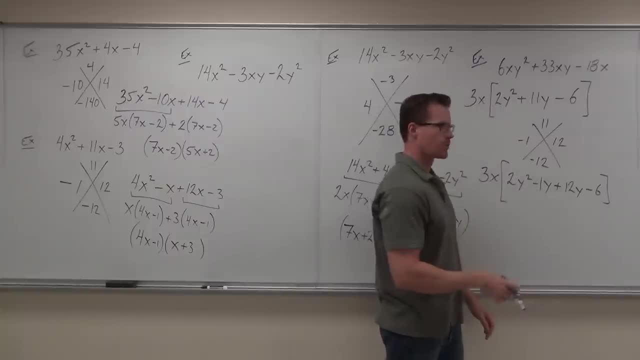 Perfect, that's exactly right. Okay, next step: We're going to factor by what's it called. Let's do that all together. okay, I'm giving everyone a chance now. Can you all tell me, please, what factors out of 2y squared minus 1y? 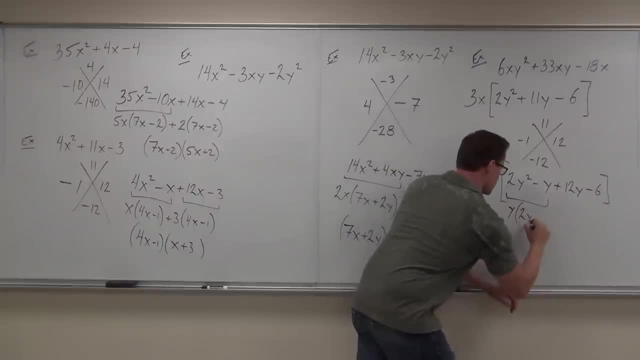 1y, And we get 2y minus 1y. Perfect, What factors out of 12y minus 6, please 6.. That plus is a positive 6, and we get what 2y minus 1y minus 1y. 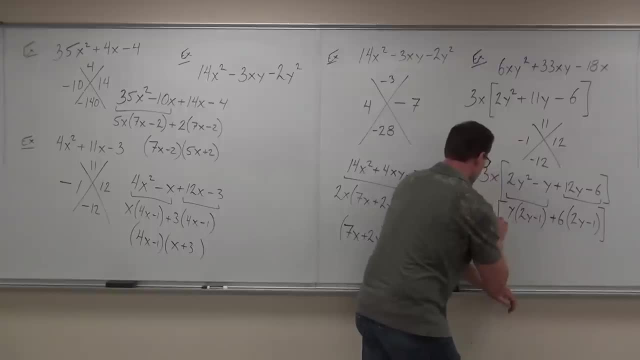 Can you verify that we have done this correctly? Yes, because they're both the same. That's how we know. If we know this is right, we can do it. Okay, If we know this is right, then these have to be the same. 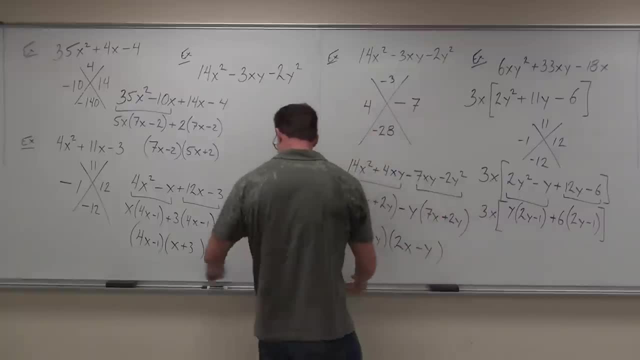 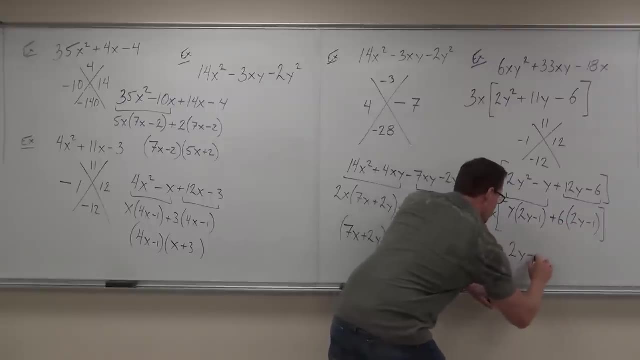 After that we're really really close to done. The only thing we're going to do is continue our grouping. We're going to keep that 3x out front. We're going to have 2y minus 1.. We factored that. 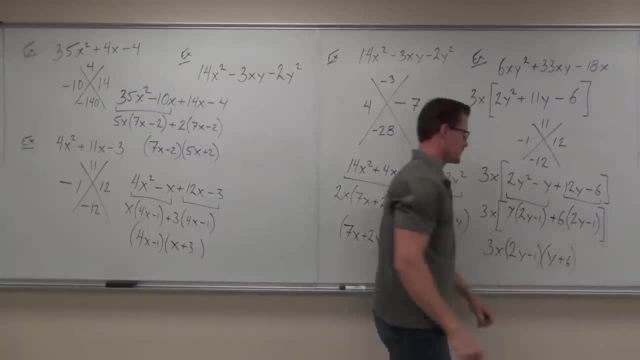 We're going to have y plus 6, and that's completely factored. We talked about this a little while ago- I think it was, I don't know, a couple of lessons ago. These brackets as soon as you're done factoring. 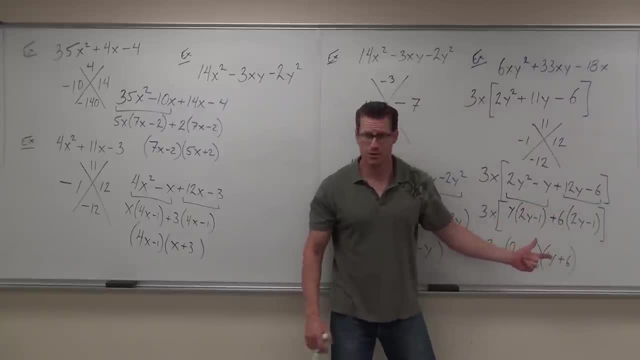 are kind of irrelevant. They are irrelevant, They really don't do anything. So if you want to keep the brackets, okay, but if you want to drop the brackets, that's fine too, because multiplication is associated with a commutative. 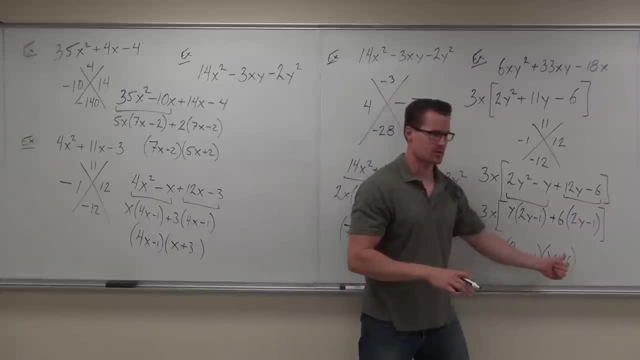 It doesn't matter the order in which we have it, So you can drop them, but keep it in this order. Two of you feel all right with that. so far, All right, fantastic. So when you did the underline, it doesn't matter if you do the. 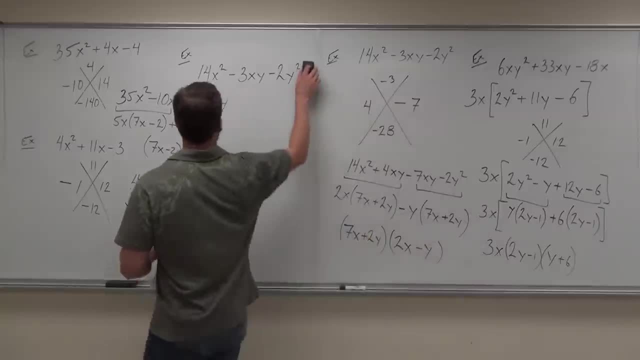 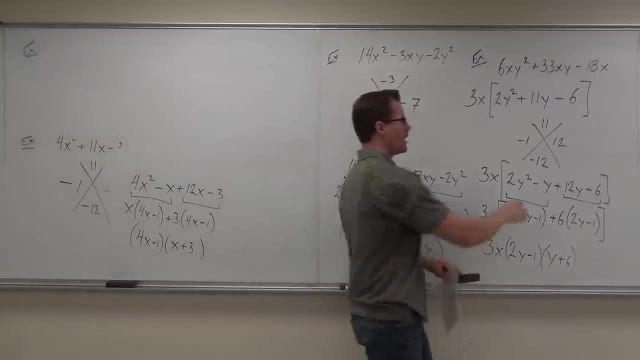 because I did minus 12, minus 1.. I did the opposite. Okay, I think I've said this a few times, but let me reiterate For the last, for the last time. I'm going to do it again, For the last time. it does not matter the order. 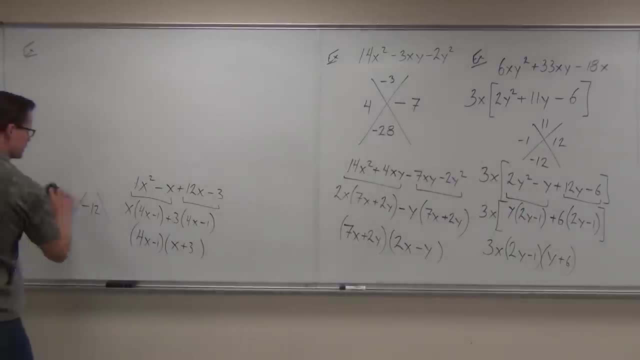 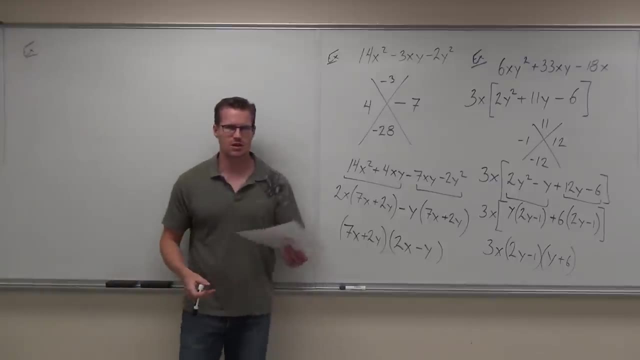 in which you have those numbers ever. Do you want to try one on your own, just to make sure you got it? Yep, Okay, after that I'm not going to give you any more to actually do on your own. I'm just going to go through a few of them. 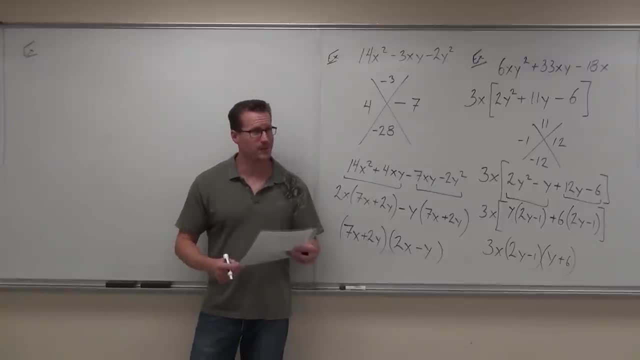 You know what? now I might give you one to do on your own at the end I got to cover these a couple to make sure that you really see it. We're going to move pretty fast on the next three examples, The reason why we're going to do that. you already know how to do this stuff, okay. 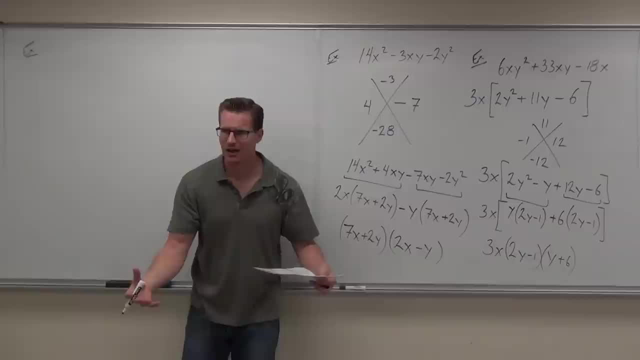 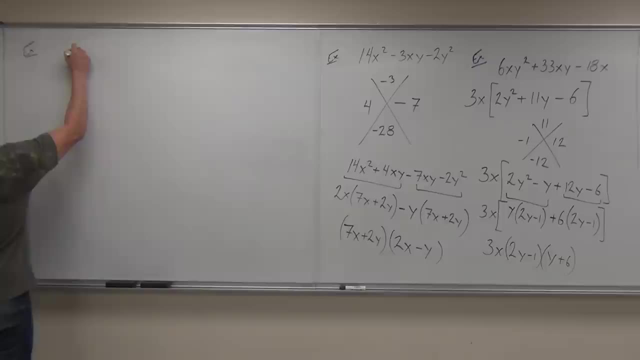 I'm going to give you some special cases on. here's your first step sort of idea. That way your factoring becomes easier. Are you with me? So check it out If you ever see a factorization where everything is in order. verify order. 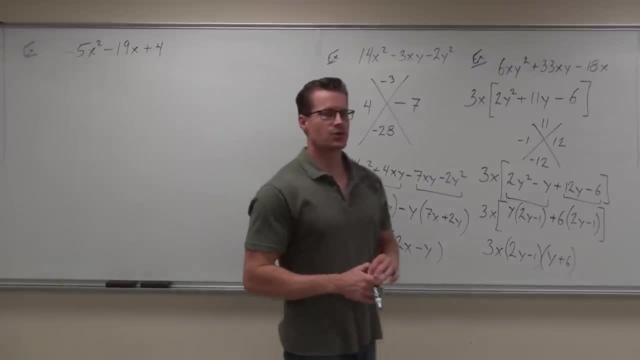 and your first term is negative. That first term is negative. That first term being negative kind of acts as your GCF if no other one is present. So here: 5,, 19,, 4, there's two prime numbers in the fourth. 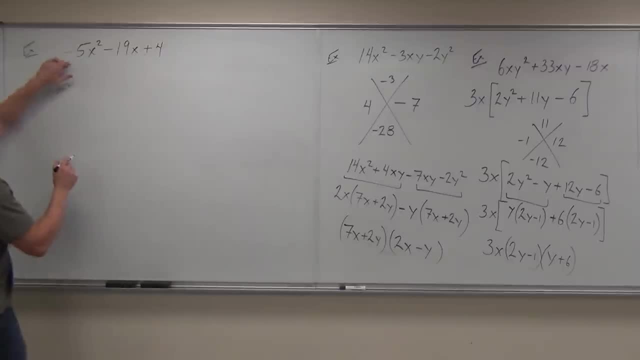 They're not going to have a GCF besides 1, but because that's negative. are you listening right now? Those are not Okay. this is important. If that number is negative, you treat your GCF as negative 1, and you're going to factor. 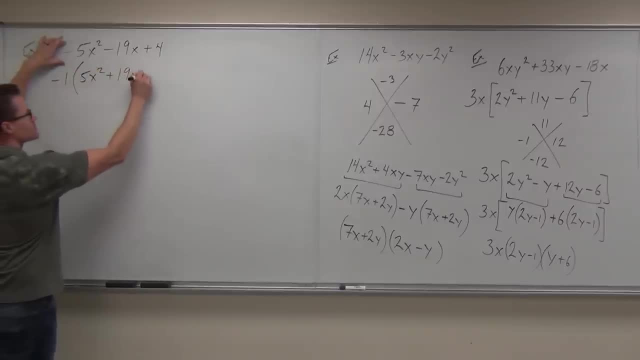 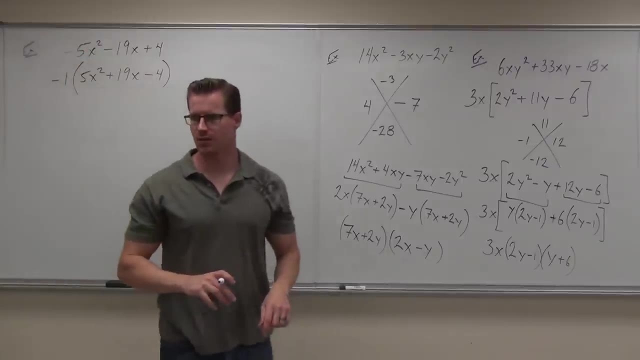 that negative out and basically it just changes all of your signs. So if I divide by negative, 1, positive, positive, negative, Quick head on if you're okay with that one. So do you see how it's changing? It's changing all three of your signs. 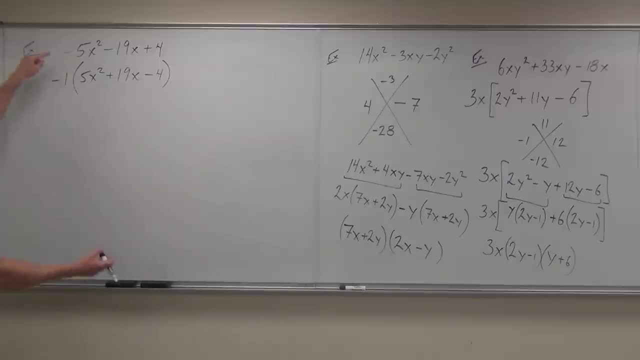 What that does. it allows the diamond problem to work for you. If you don't do that, it's really hard to do the diamond problem. All right, This makes it easier. So once we factor the negative, then we set up our diamond problem. 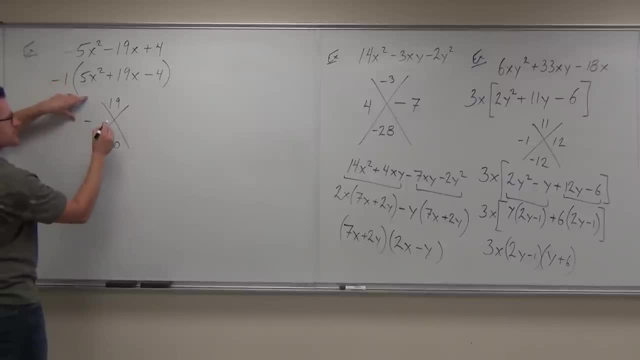 We're looking for different signs. The difference is 19.. That's got to be positive 20 and negative 1.. I said I'm going to go quick on this, okay. So when we do that, we're going to have 5x squared minus x plus 20x minus 4x. 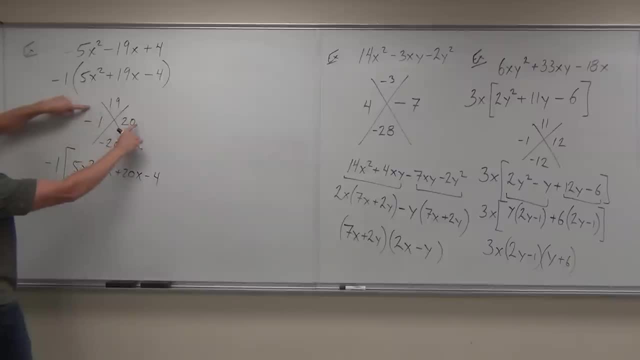 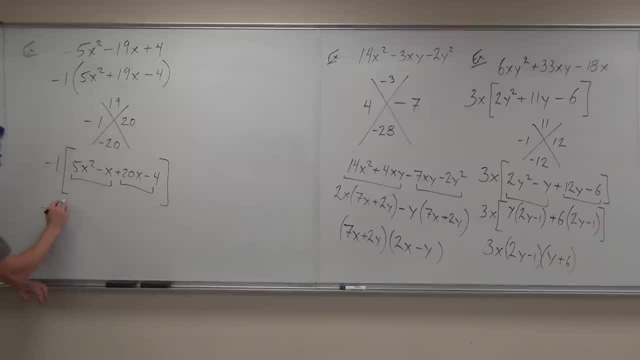 We'll continue our factorization by grouping. Keep your negative 1 up front. We got x and 5x minus 1 plus 4 and then 5x minus 1.. Hey, look at that, We did it right, because our factors are exactly the same. 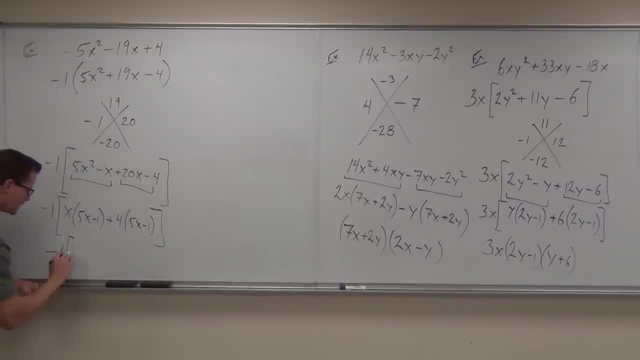 So we'll have our negative, We'll have our bracket, We'll have our 5x minus 1, because that's a common factor. We'll have our x plus 4, because those are remaining Parts of my terms that didn't factor out and that's our final answer. 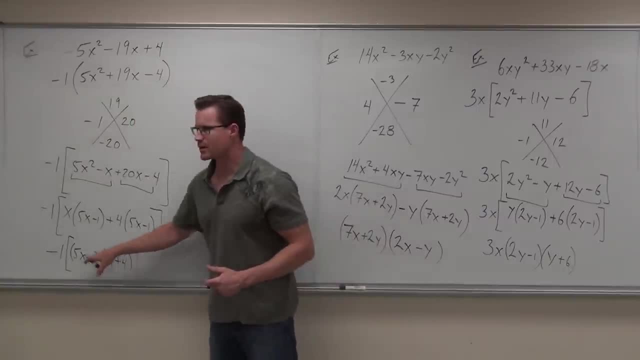 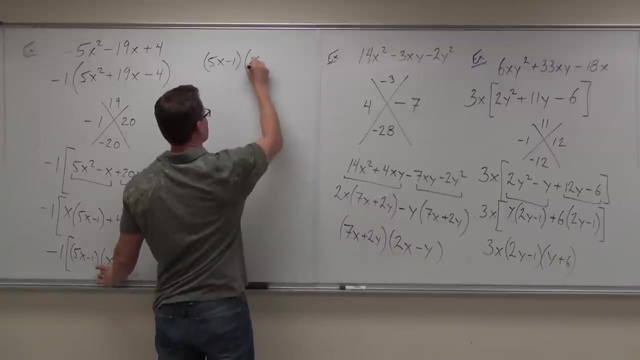 You should really clean this up just a little bit, because this has a lot of stuff you don't need. Here's what I mean by this. okay, You don't really need these brackets, You don't really even need that 1.. How this should look is 5x minus 1, x plus 4, with just a negative in front of it. 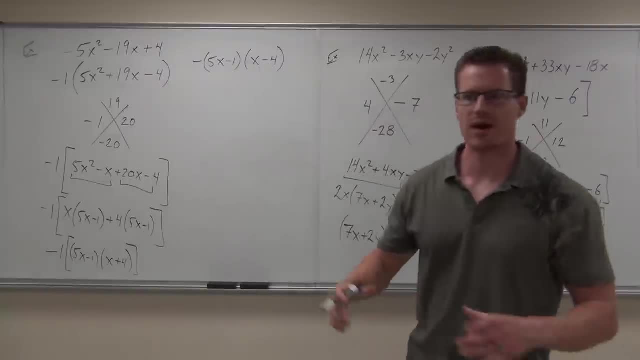 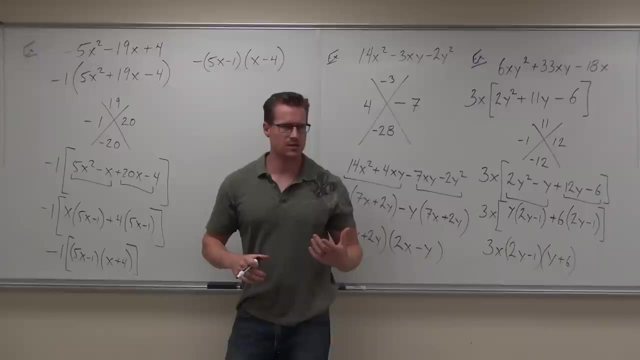 and that's appropriate. That negative it stands for negative 1. The brackets were just kind of holding this thing, So we're going to put this stuff in here until we finish our factoring, and that's just fine. Did I explain that well enough for you guys? 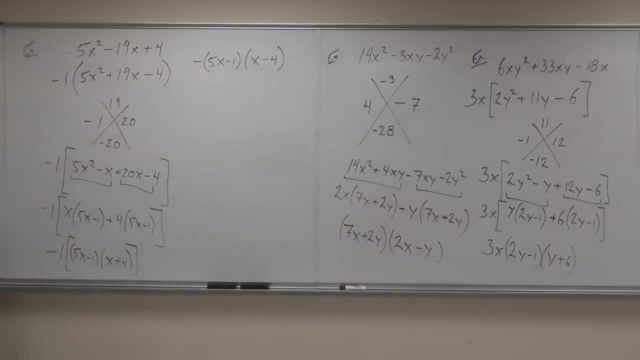 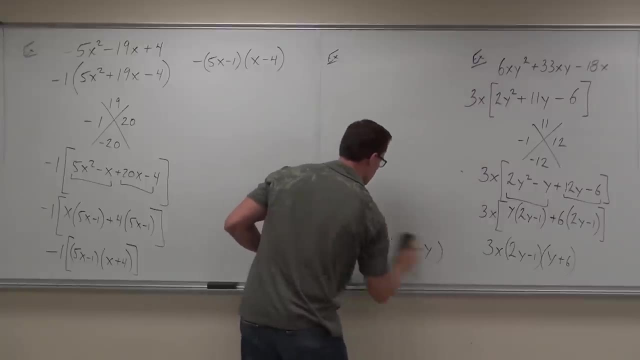 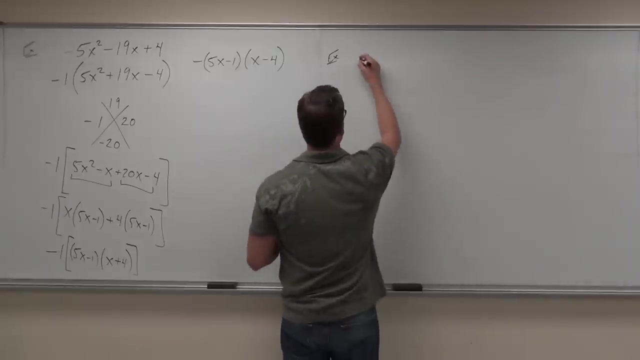 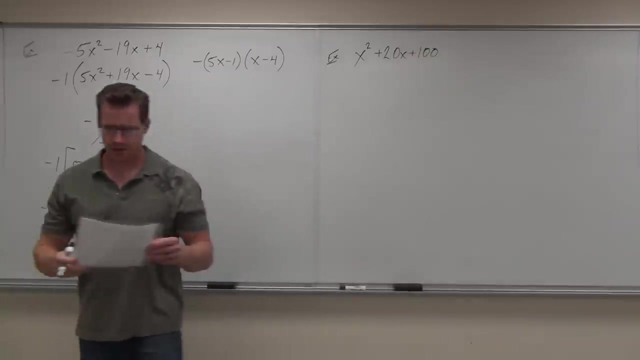 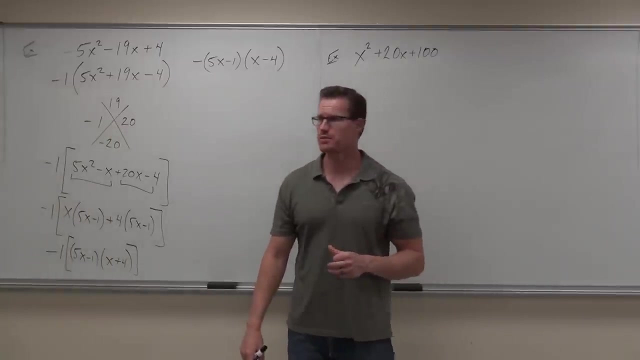 Yeah, Okay, So two more. This one's going to go really quick. Can you check the order for me? Is it good? Do we have a GCF? How many terms have we got Diamond 20 and 100.. 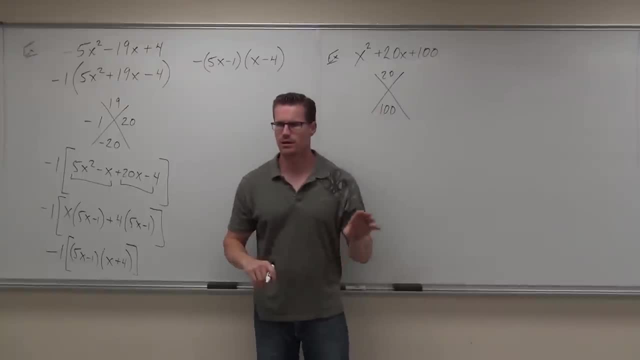 Can you give me two numbers which add to 20 and multiply to 100?? Now here's a question: Do I have to go through this whole process or can I go directly to my factors? Can I do the shortcut? Yes, 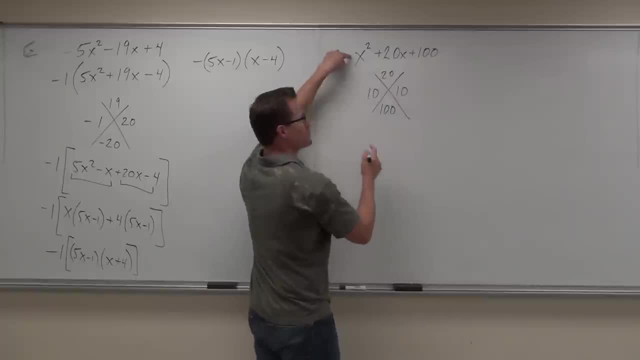 Why I just want to do one number. That's beautiful, It's a beautiful thing. So this would be X plus 10 and X plus 10.. The reason why I'm giving you this example is because this is absolutely right, but we like to make, as mathematicians, things as concise as possible. 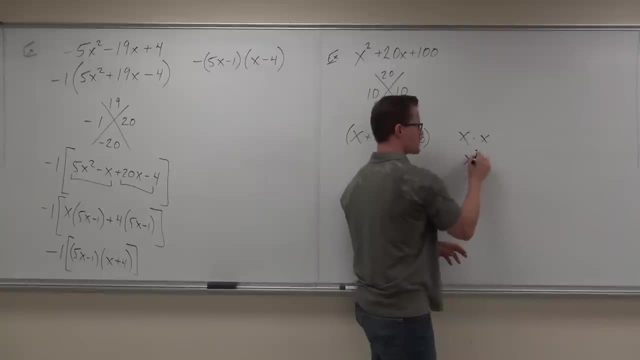 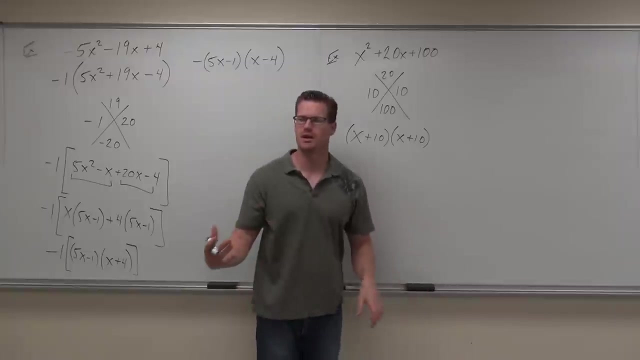 Now you know that X times X gives you X squared correct. In fact, any two of the same factors that are multiplied together, we can represent that by an exponent, hence its repeated multiplication. Same thing happens here: If we get X plus 10 times X plus 10, we do X plus 10,. 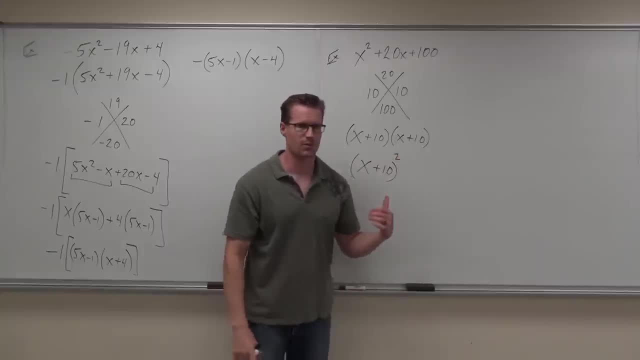 and then we square it. And that's all I wanted you to see out of that problem. Firstly, don't forget there's a shortcut, okay, because that saves you time. Secondly, whenever you have the same factor twice, just have it as that factor to the second power. 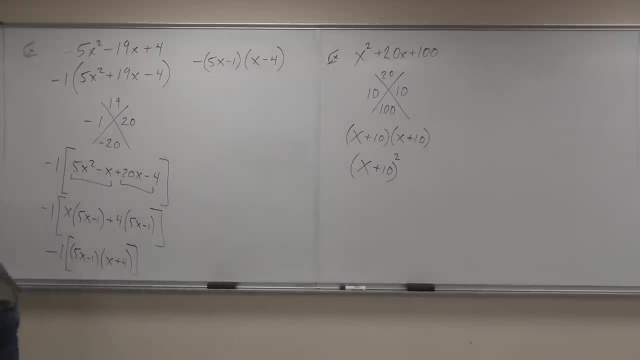 So far, so good on that one. Mm-hmm. Okay, You know what? Maybe I can. I'm going to give you one. Let me see How far are you going to get in that A minute. Can you do it? 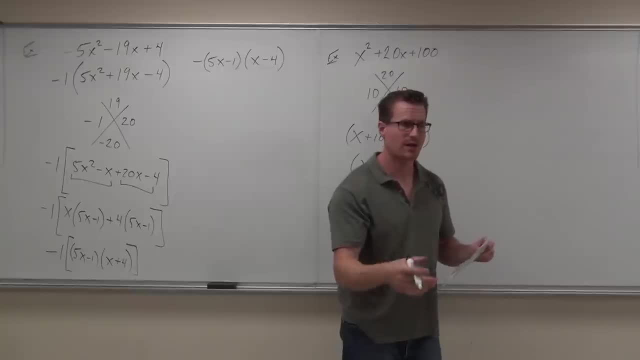 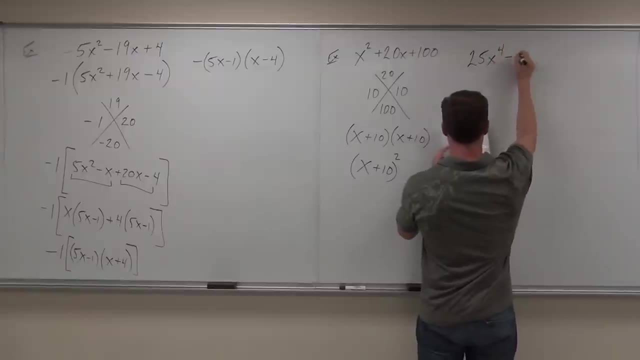 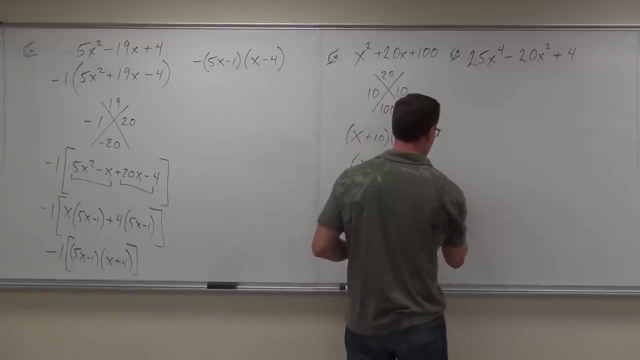 Mm-hmm. Okay, This is. this combines a couple ideas that we've had already, but just just be careful, Go for it. We're not going to have time to do this very last problem and I'm not going to do it. 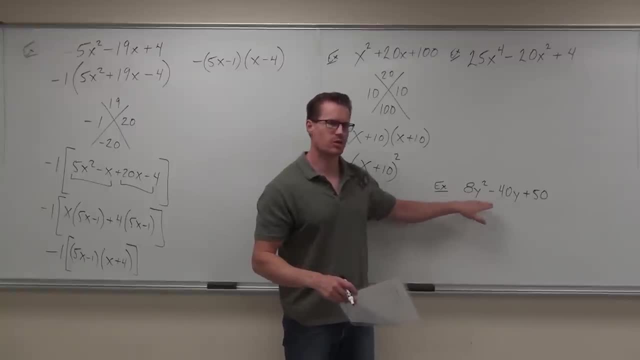 But I want you to think of something on this problem. Just think about what your first step would be. okay, Can you do that for me, Don't? you don't need to do it. Just think about what your first step would be. 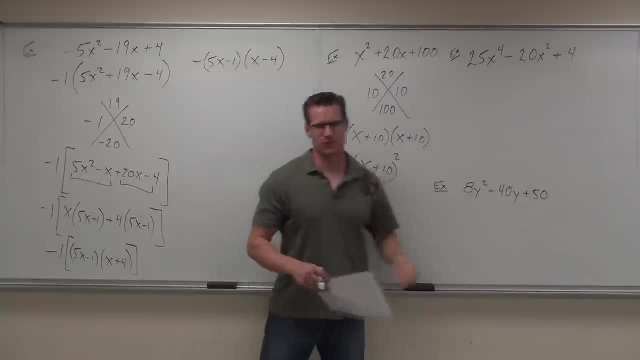 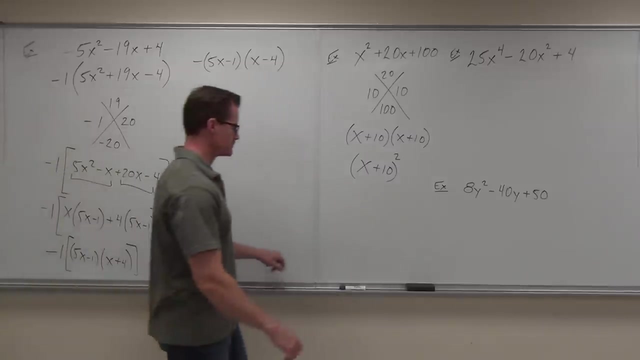 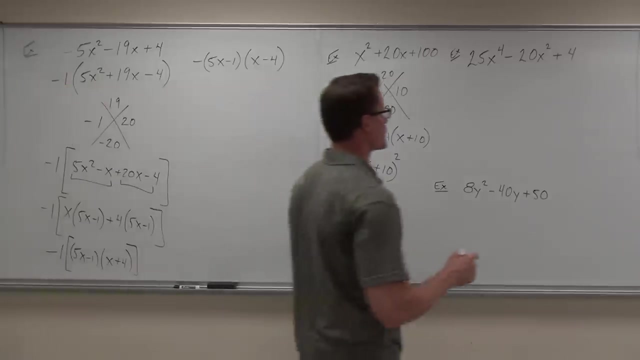 So I want you to try this one. I'll give you about another minute And then I want you to think about your first step. Okay, Thank you. Okay, I'm giving you as much time as I can because I've got to wrap this thing up here. 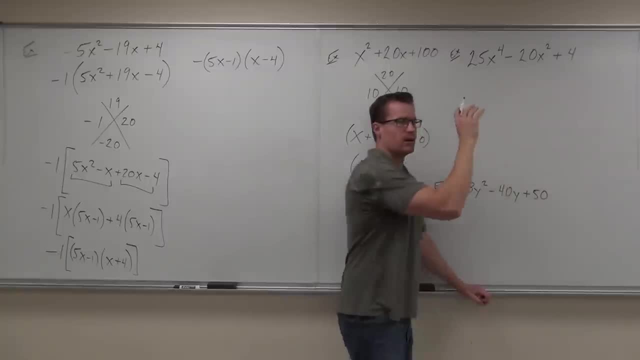 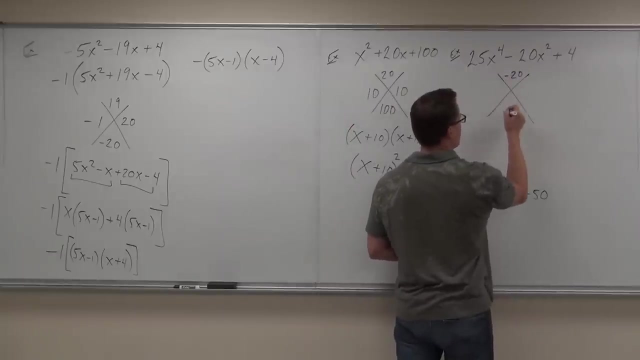 So first one order: Sure, Positive first term. Yeah, GCF, besides one. No, You want it to be, Looks almost like it is, but it's not, You can't do it. So since there's three terms, we do the diamond problem. 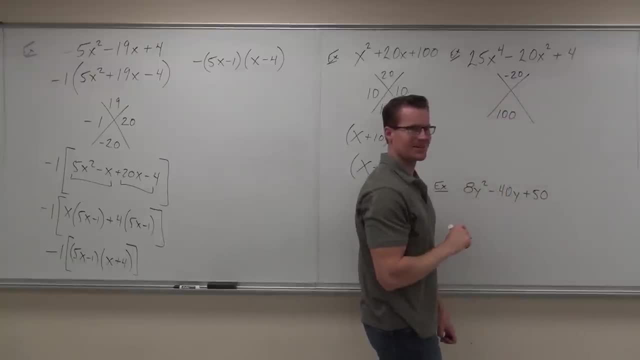 I want to give you really nice numbers, didn't I? What a nice guy I am today. Look at that. Such a nice guy. Negative 10,, negative 10.. Did you find that? Yeah, Okay, Don't go to the shortcut. 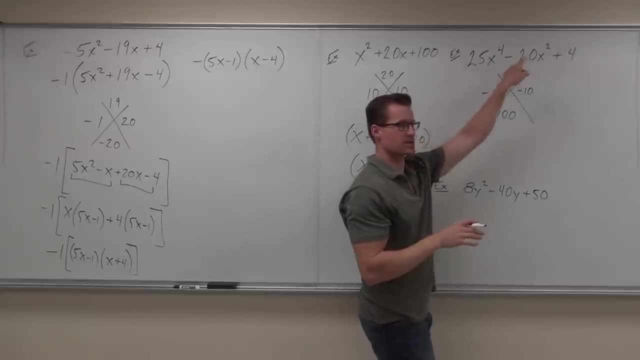 Do the grouping and don't forget that that is an x to the fourth power and that's x to the second power. Okay, you've got to split it up like that. So we have 25x to the fourth minus 10x to the second. 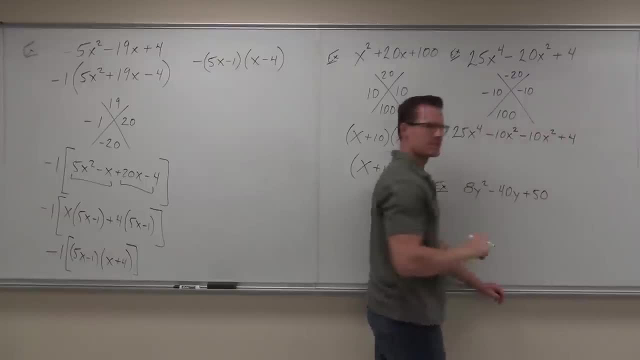 Okay, Does that make sense to you? Yeah, You've got to have the x squared. After that, our grouping will work just fine. We'll factor out the 5x to the second and we'll get 5x to the second minus 2.. 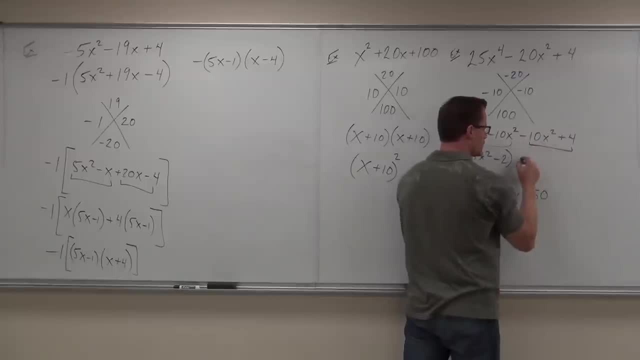 This says you have to factor out a negative. So when I group these it'll be negative 2, and what that'll do is change our sign to positive 5x to the second minus 2.. And you can see right here: this factors very nicely as 5x to the second minus 2.. 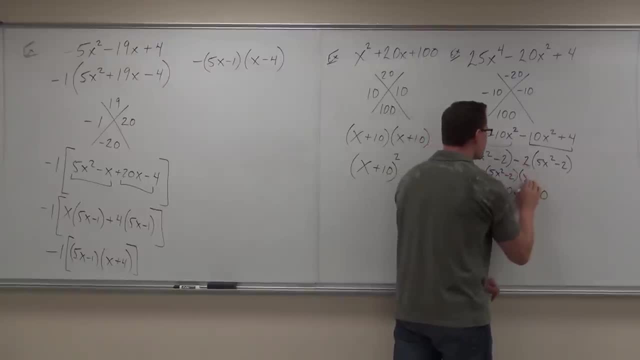 Oh, wait a minute, And there's another 5x to the second minus 2.. Should I leave it like that? No, Is it technically correct? Yeah, But we want to make it nice with it And that's the idea. 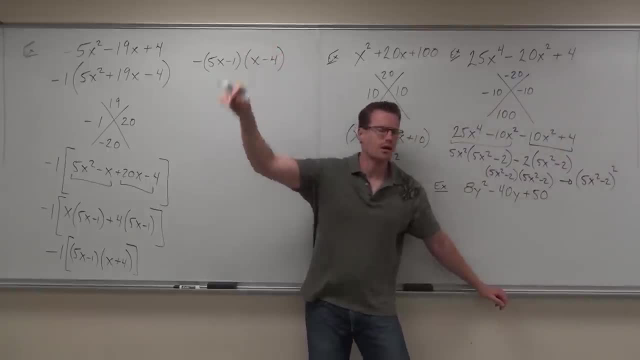 Should we be okay with that idea? Okay, before you go, I'll ask you for one thing: What's your first step? Is it in order? Yes, Is your first term positive? Yes, What do you do after that? Is there a GCF besides 1?? 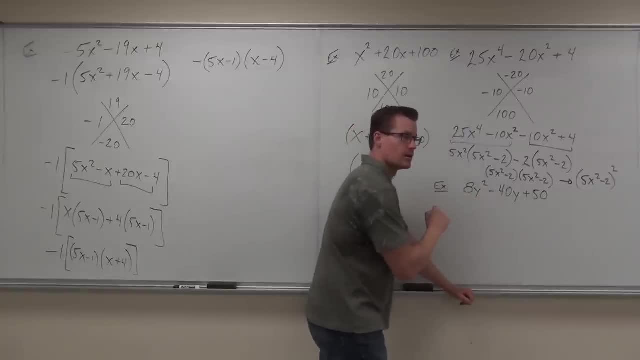 Yes, Okay. so your first step here is to factor. You're going to figure out what: 2.. 2. The factor of the 2, you get 4y squared minus 20y plus 25.. Can you go away before you go?